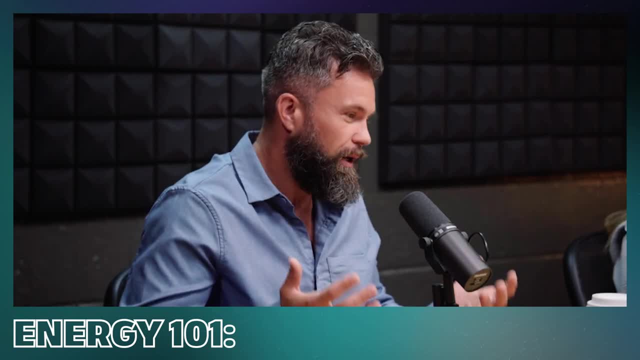 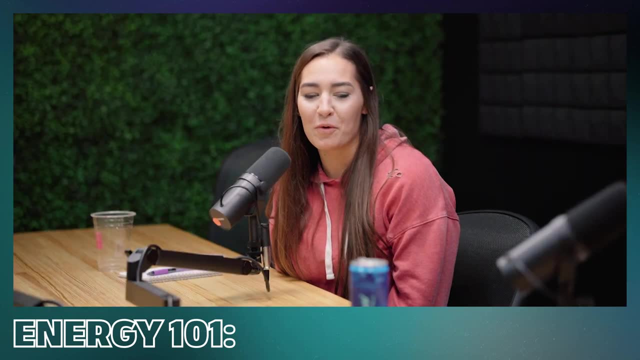 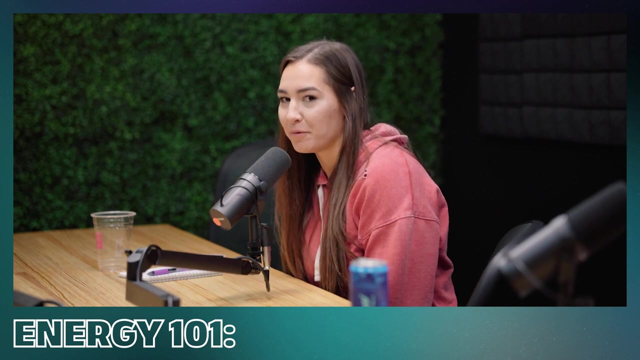 you ladies, nowadays you be careful. um, maybe you identify something else, I don't know. but however, uh, yeah, no super pumped to be here. so thank you, yeah, so excited, um, so kind of what you were saying. we, we don't want to educate not the echo chamber but outside of that. we want to really reach the. 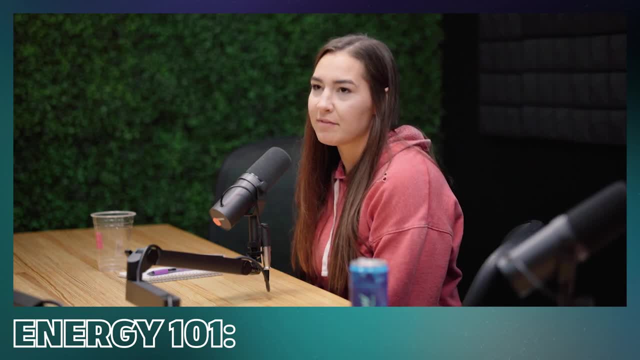 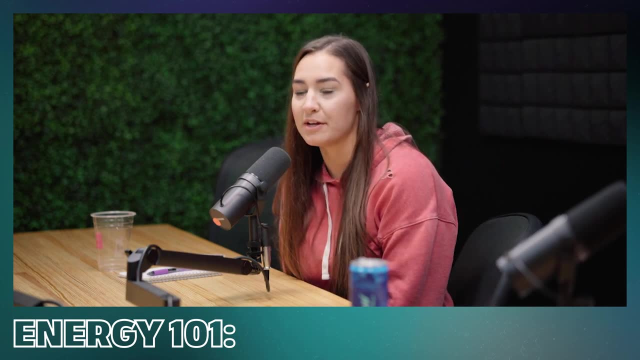 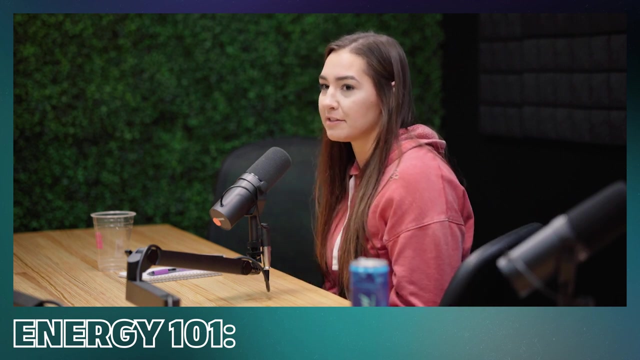 people who don't know anything. and it's interesting because I did have a conversation yesterday. I was talking to a parent at jujitsu. he's from San Francisco. they moved to Houston, um in January to become entrepreneurs, so they are in real estate and they're just like this. 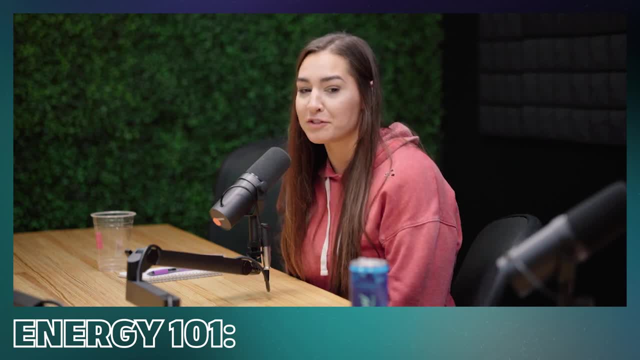 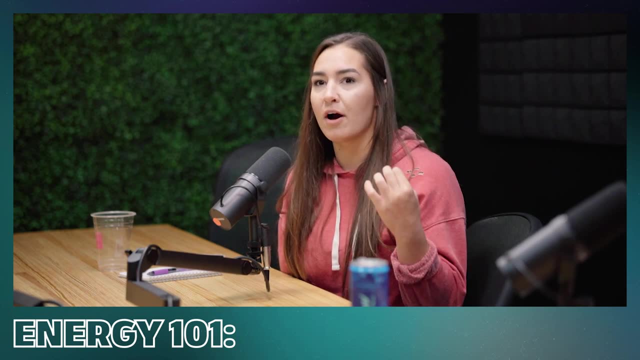 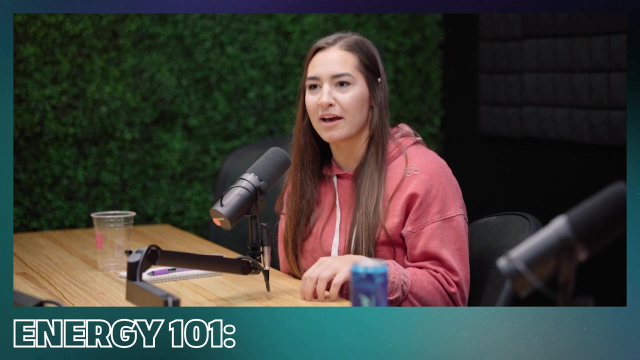 is a place to be. they know nothing about oil and gas. so when I started like saying talking about digital wildcatters and oil and gas energy, his immediate thought was to talk about um, electricity prices and like those companies and I'm like: well, that's not exactly like. 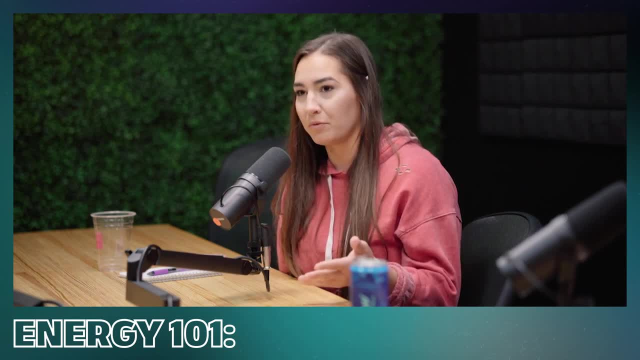 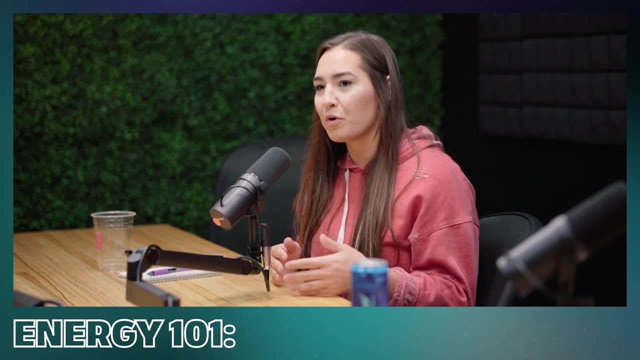 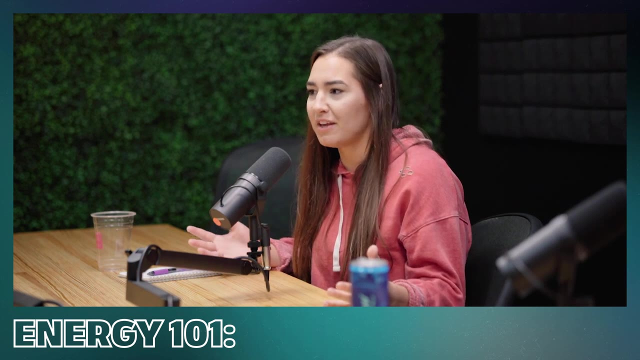 what the companies do, that we kind of work like our clients and who we like try to educate, like that's different. but I didn't know how to explain that, sure. so how would you explain oil and gas to someone who, like him, he's like I have, like it seemed like he had barely even heard. 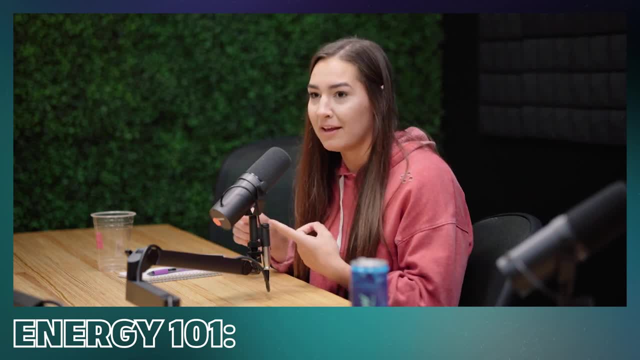 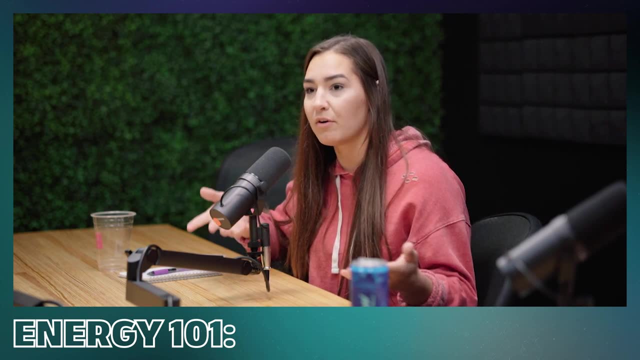 yeah, of oil and gas, like I think he thought of gasoline, right, and then of, like, the electricity companies, which that's not wrong, it's just right. how do you kind of explain that? yeah, no, that I mean, it's a great question and I think that's something that we 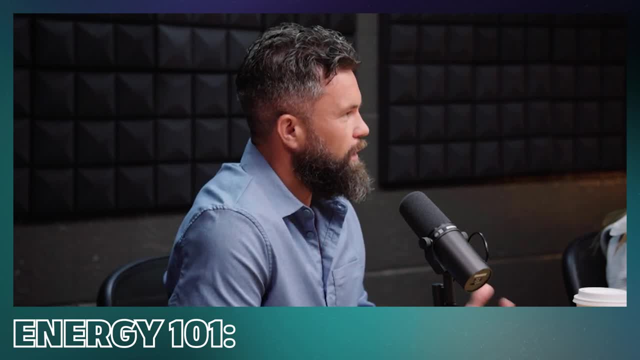 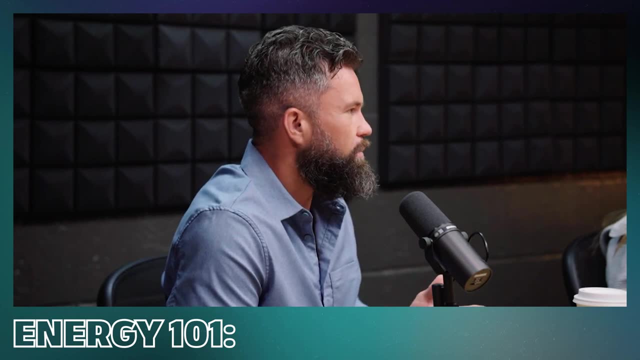 need to. it's kind of like when you go, when you have a company and you have a sales pitch or an elevator pitch, it's like, well, what do you do? you need to be able to explain it within like 30 seconds, maybe less. if not, it's people use too much energy- energy to try and figure out what. 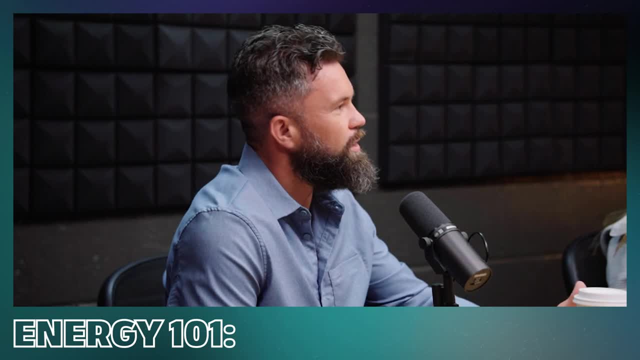 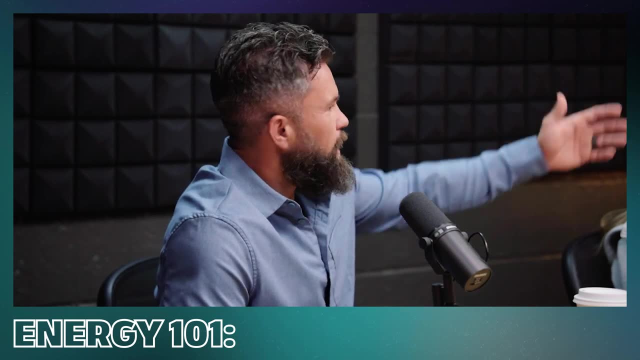 the hell you're trying to talk about um. so so that's an interesting question and an answer. anyone within the oil and gas space or in any space, whether you're um, you design signs or you know you're an oil and gas, or you provide electricity or you make coffee cups like you. 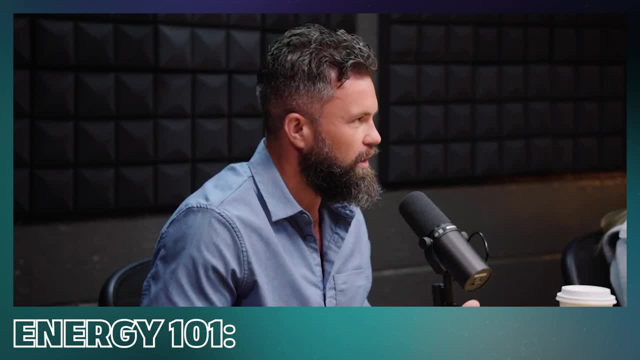 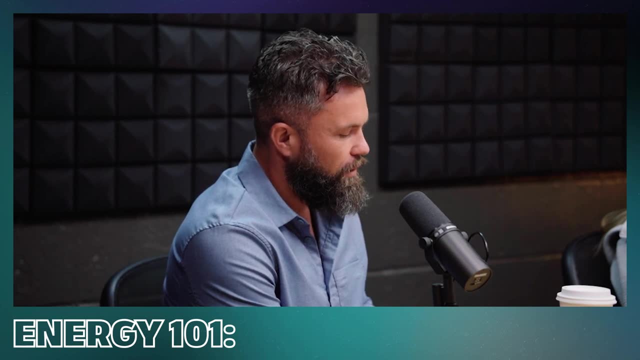 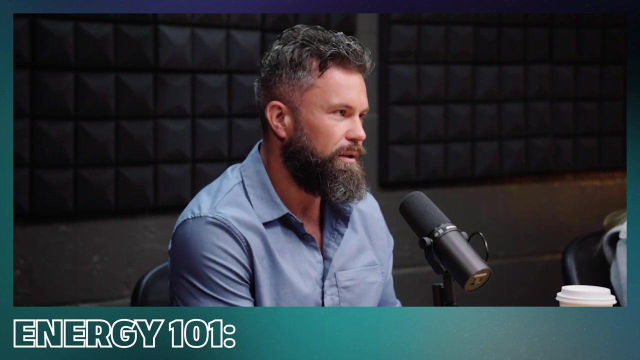 should be able to explain it simply to where people like can digest it and say, oh, like, that makes sense to me. um and so and I'll answer your question. but, uh, I had the pleasure of having a gentleman on my podcast who connected with my wife over LinkedIn. he's in the real estate, uh industry. 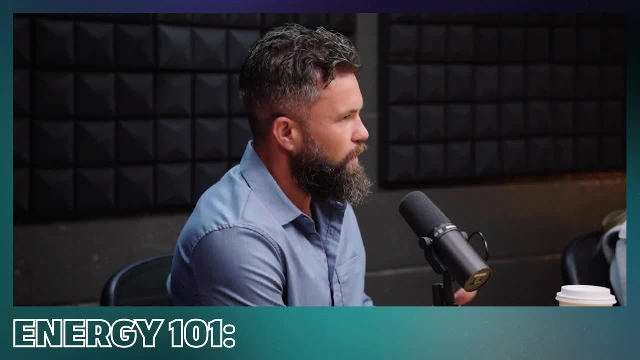 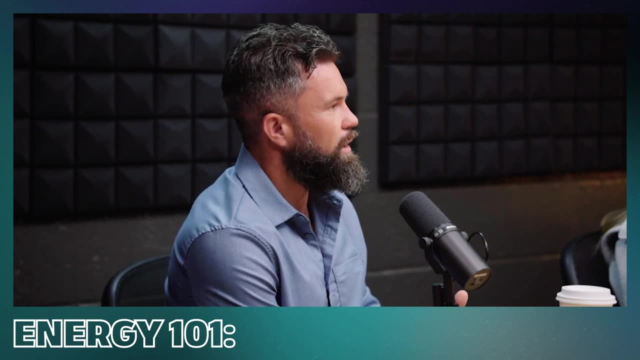 he also had no idea about oil and gas. he, although he was from Oklahoma, he had traveled growing up quite a bit and um he was starting to make comments on my posts, um just saying oh wow, that was interesting or whatever. and so I looked at his background- not oil and gas related at all. I 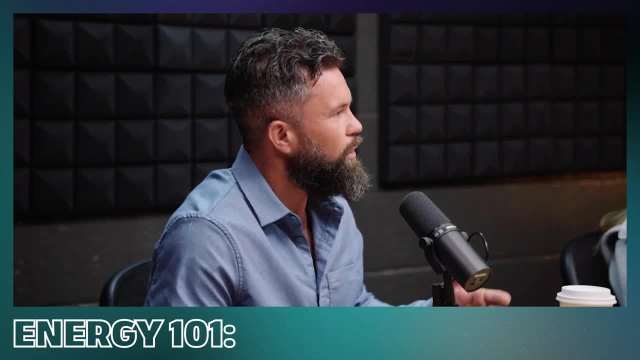 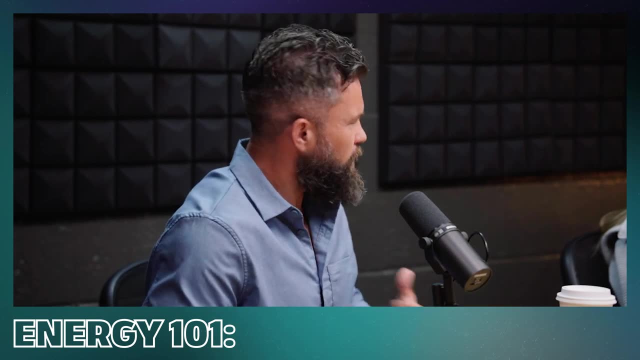 was like: man, why don't you come on my podcast? because I was like I'd be interested to hear your perspective as someone who is outside the oil and gas, you know, ecosystem. like give me your honest opinion on us as an industry. because I'm curious, because anyone I ever talked to has 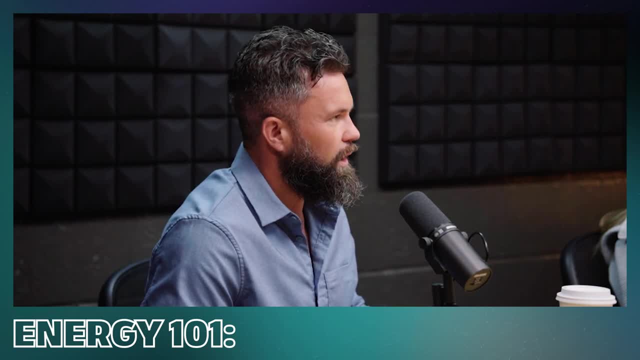 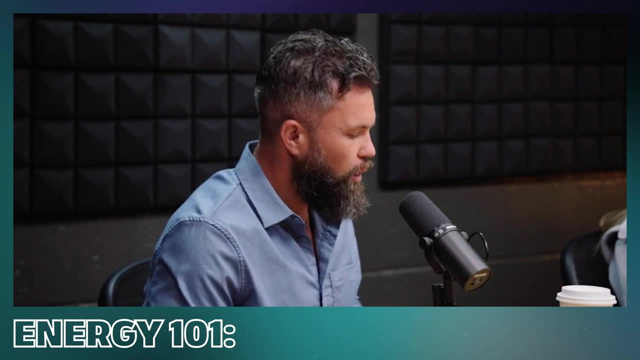 ever talked to. I mean, I have people within my social circle that aren't oil and gas but they're here in Houston and so like they appreciate the industry for what it is and what it provides. but this gentleman had no, you know no experience with it and so I had him on and you know we had a great 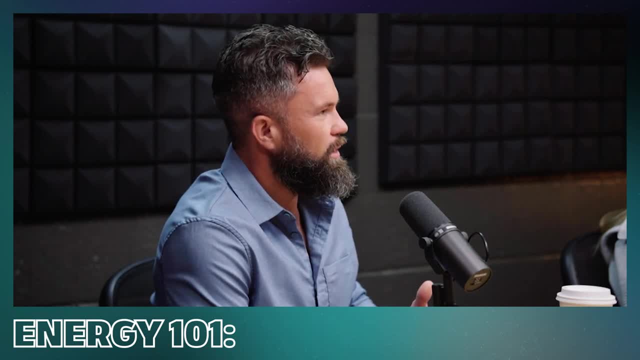 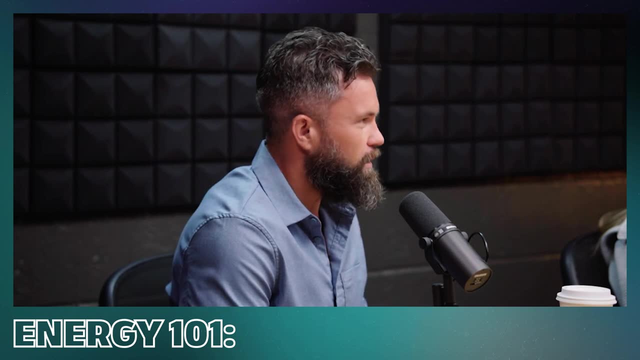 conversation and he said: man like I, I listened to your podcast and he's like to be honest. growing up, he's like it was like the big bad oil and gas companies that all they wanted to do- is you know, is ruin the earth and make as much money as possible. and he's like, but after being you know, 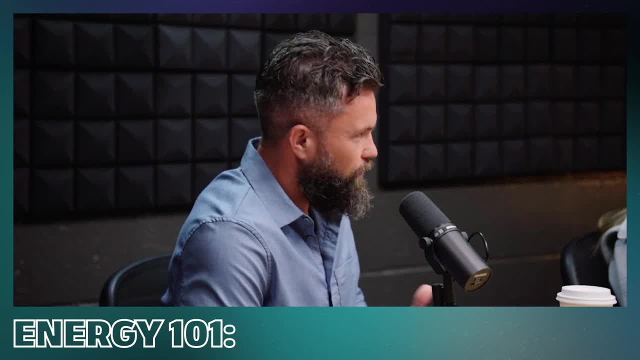 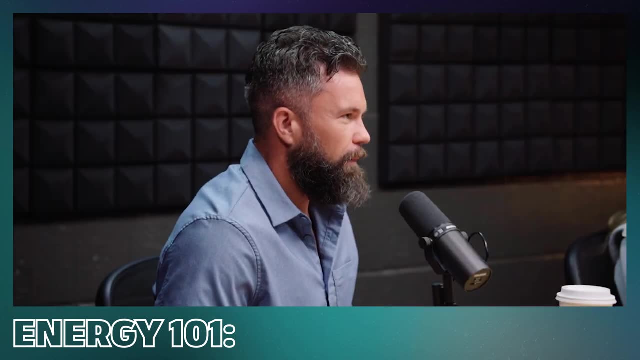 listening to your podcast, looking at your content- a you're a good guy, which you know- I thought everyone in oil and gas was just like a bunch of rednecks who were mean, right, or whatever, like whatever the perception was. um, so you know, we got that sort of you know biases out of the window and then you know he, he said yeah after. 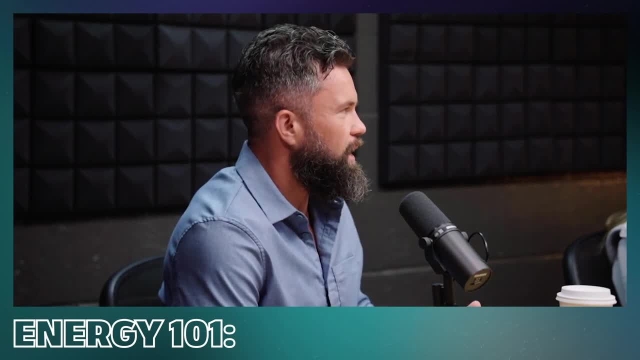 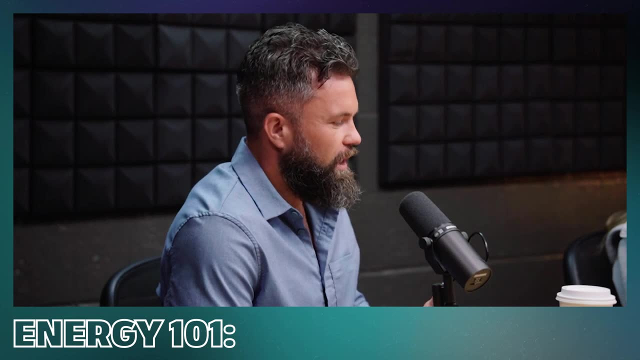 he's like. I listened to one of your podcasts and it was funny because that same day he was with his friends and they were complaining about gas prices. and then he's like. you know I'm not not big on like economics, this and that he's like, but I I had enough of an understanding based off your. 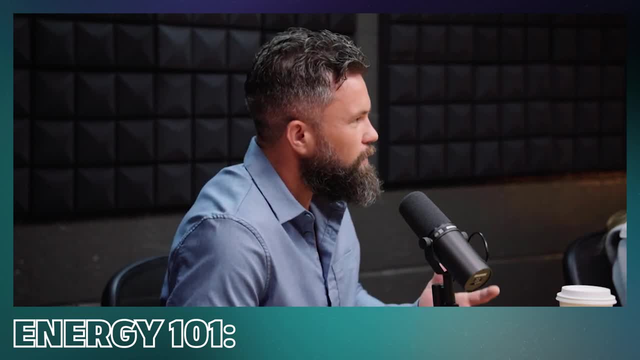 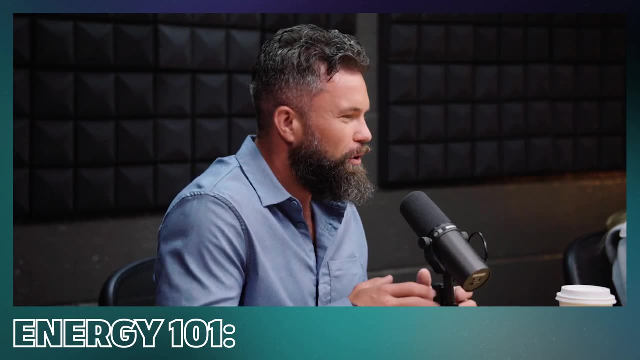 I could explain. like it's like the oil companies aren't the ones that you should be blaming and, according to this podcast, like there's this thing called supply and demand and he like tried to piece it together. but ultimately I helped him and I say I, you know the people that I had on, you know the. 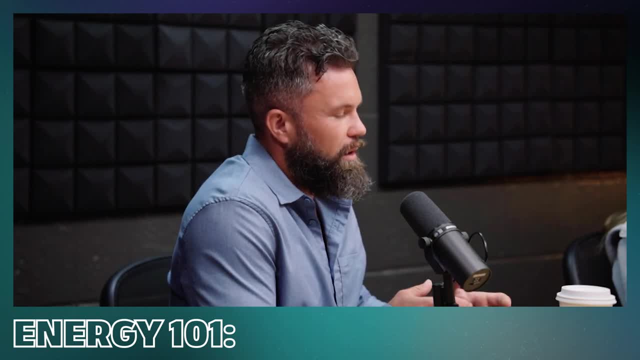 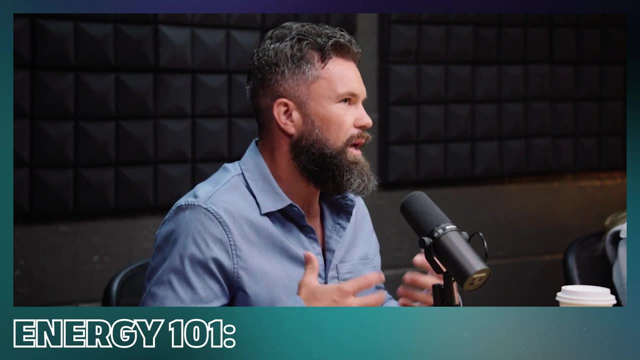 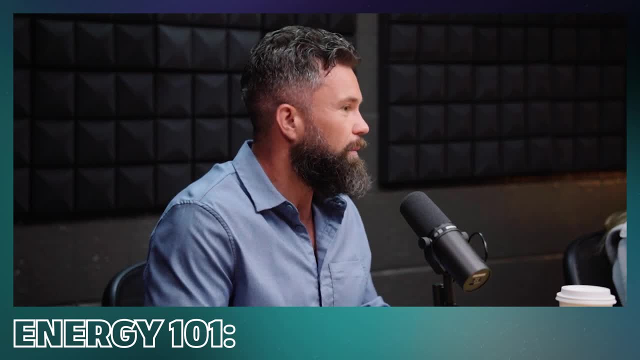 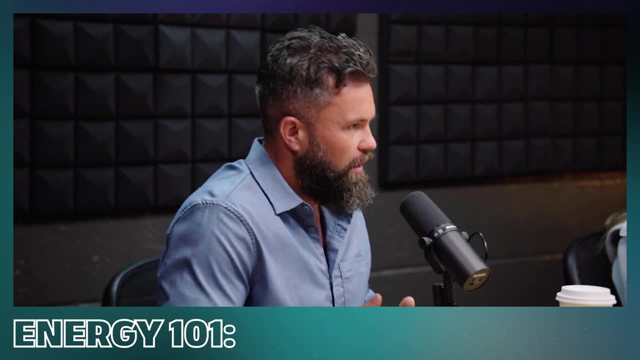 oil and gas is actually extremely important. I didn't realize that, um, because he said he grew up in a family or it was kind of demonized and everything else. but but now he and he said I actually would love for my kids, like if they told me they wanted to get in the oil and gas industry. 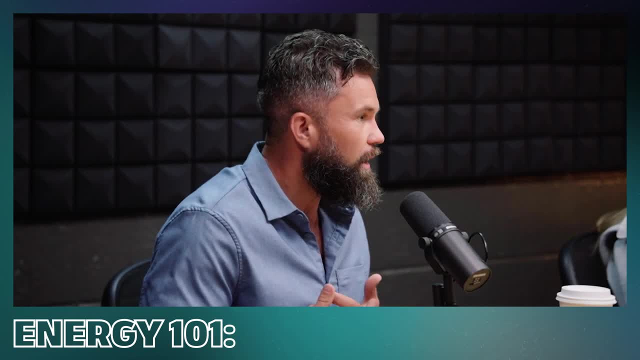 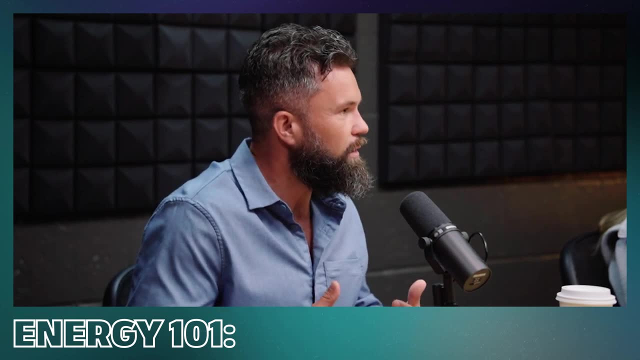 I would encourage them to do so, because it sounds like there's plenty of opportunity, and that was amazing to me. like I, I ultimately hope that, like that, next generation of his family can at least appreciate and have a decent understanding based off their dad's knowledge of the industry. so 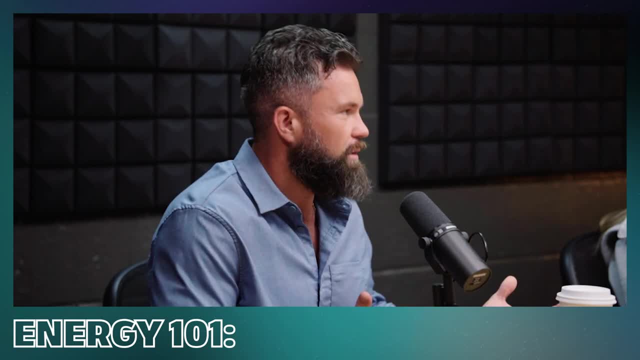 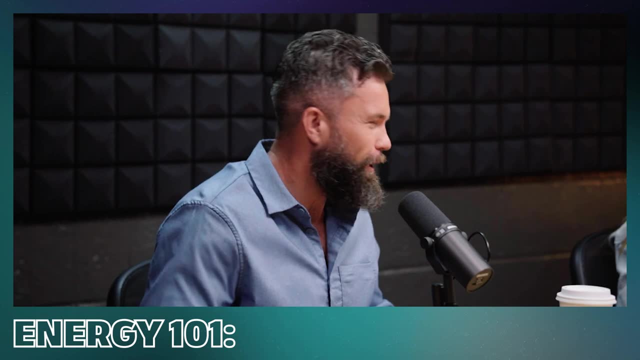 Um, that, to me, is why I podcast is for that exact reason. So to go back and answer your question, like someone comes from whatever California or wherever and says, well, what's oil and gas? Um, and, and what do you guys do? 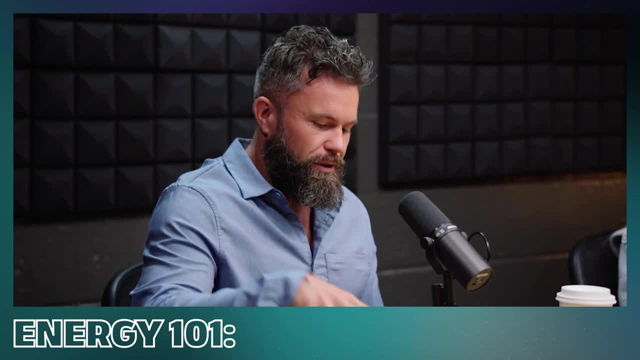 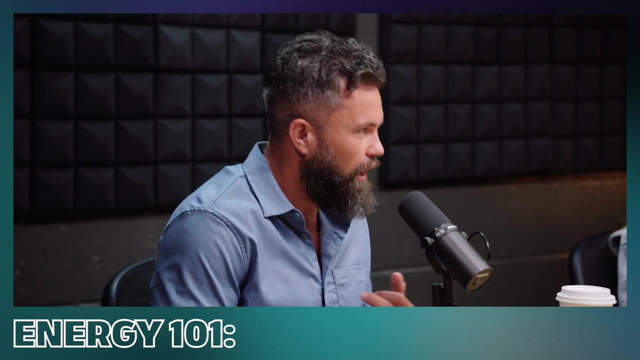 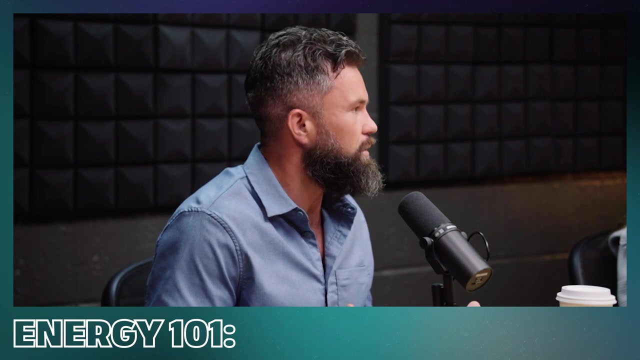 Like ultimately it's. you know you have three parts: you, you, you drill and you, you, you extract stuff from the ground and that stuff helps create energy, It helps create cups, It helps it's. hydrocarbons are the backbone for almost anything that we use. 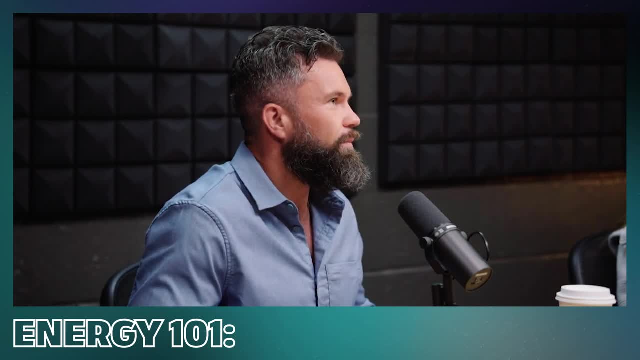 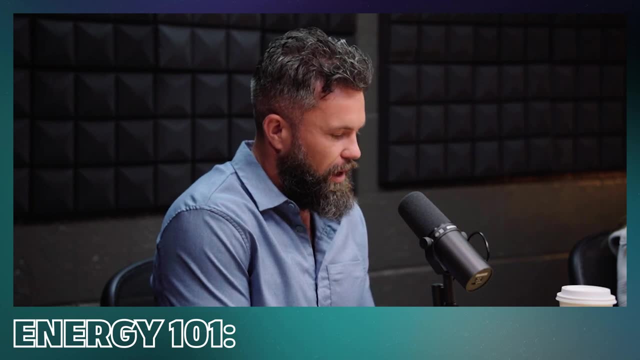 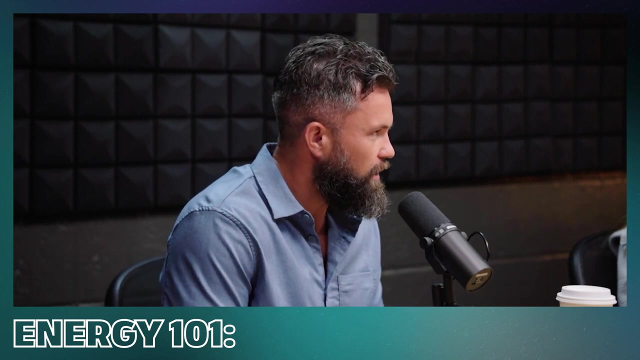 Um, and so that you know. hopefully that's very broad, but I I would. I would start with: like you know, the earth has these minerals and this liquid and this gas that ultimately helps make everything you see around us. 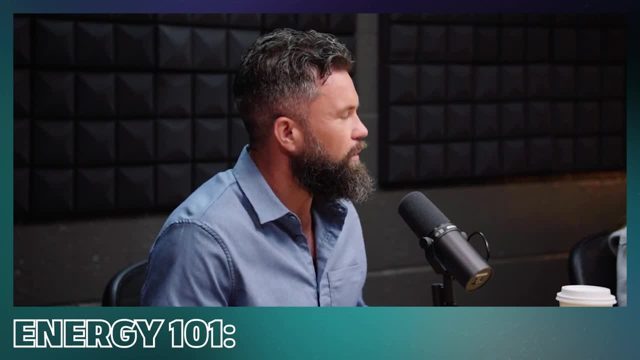 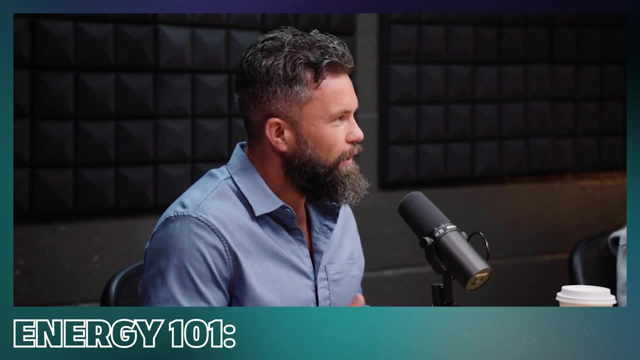 Um, and then it's like: oh, really, Like. well, give me an example, And gasoline is the easiest one, right? Um, you know you, you extract the oil from the ground and and through different processes. 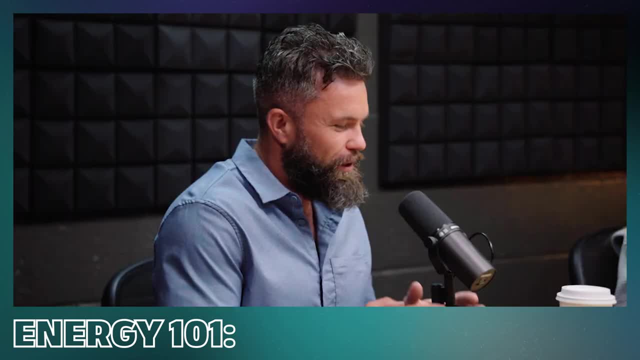 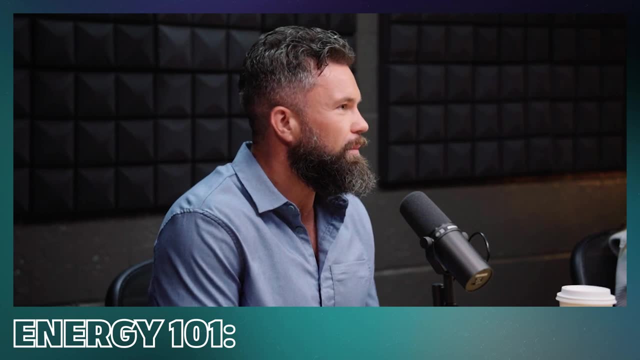 I'm trying to keep it like super generic, through different to through different. uh, there's a process that can you know: essentially separate it and create gasoline for your vehicle. Um, you know that that's the easiest example, but there then there's, there's tons out. 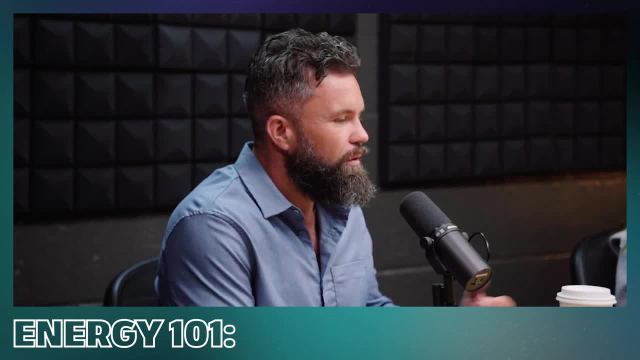 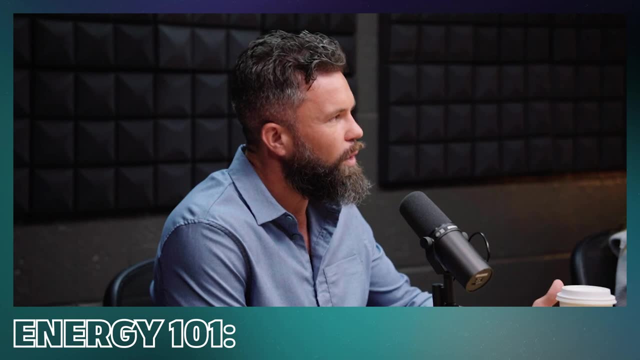 there, Uh, and so when, when you had the interaction with, with this gentleman, were you his? his question was: what is oil and gas, or like, how, or what is you? what do you do? He didn't ask. 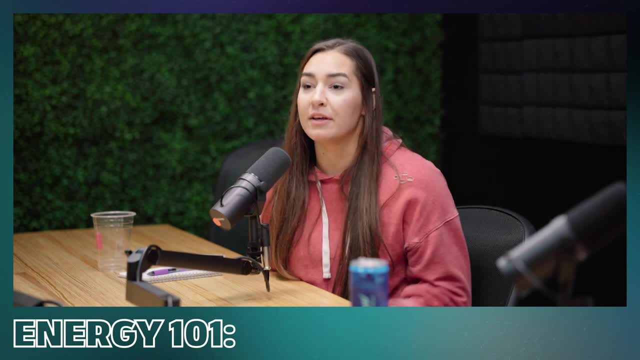 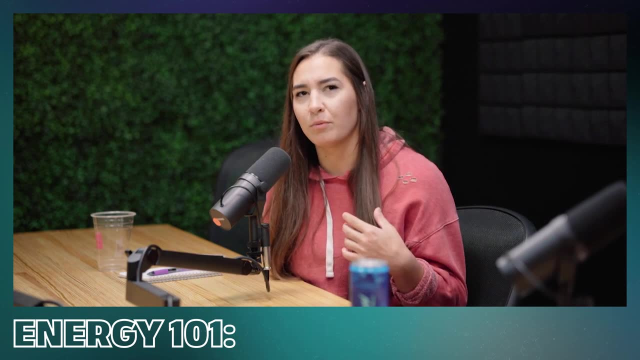 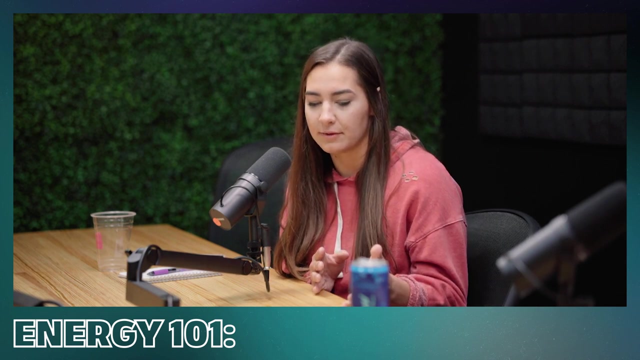 So we were talking about just yeah, what we do, the the basically um industry. Yeah, And I could just tell by the look on his face he was like: like what is oil, oil and gas? Like he didn't, he was. it seemed like he was thinking like, yeah, like I said gasoline. 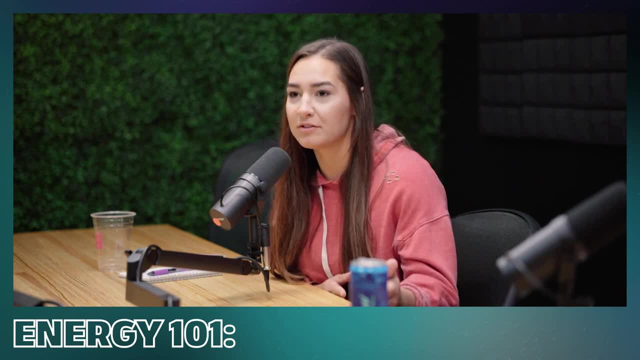 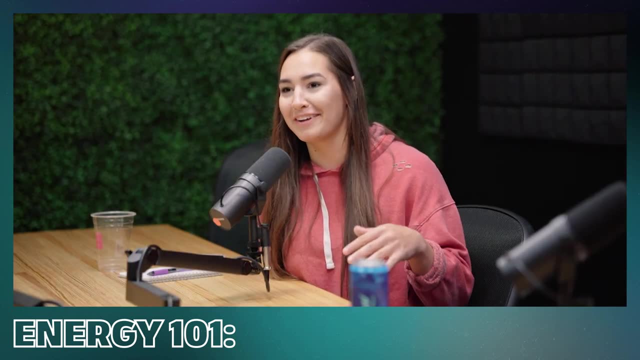 or just um electric companies. So like electricity companies, Right Rather Cause he started talking. He started talking about: uh, how it's crazy here um where you have like a ton of different electricity companies to choose from. 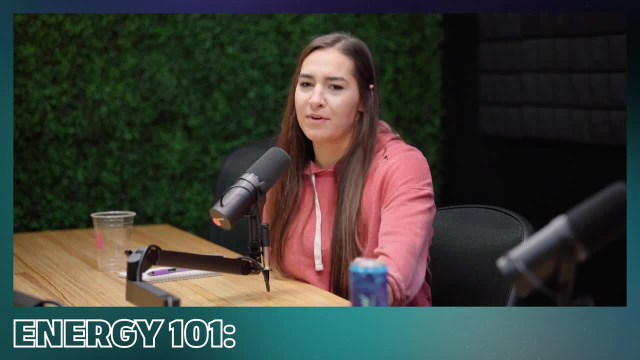 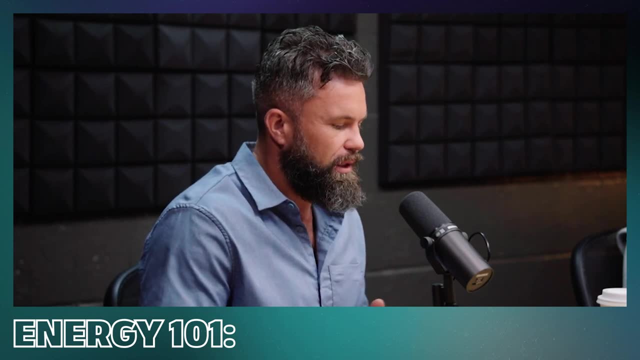 Ah, yeah, So his mind went immediately to that, which is fine, It's all connected, Right, Yeah, Yeah, And so I, I guess in to to like to get a little bit more technical, I guess, like I. 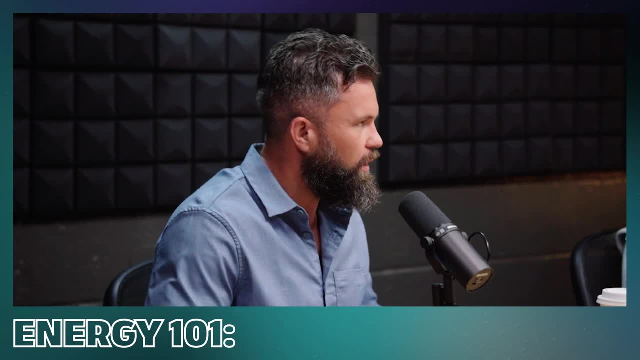 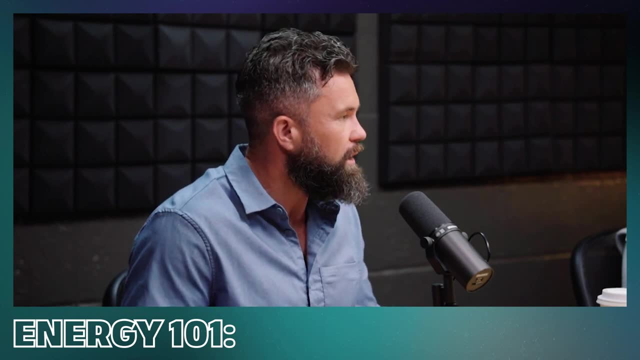 would if someone asked me. I would say: well, there's three main components of of the oil and gas industry. You have the upstream, which is where you everything happens out in the middle of nowhere and you drill and you extract the oil and gas. and you have the midstream, which you 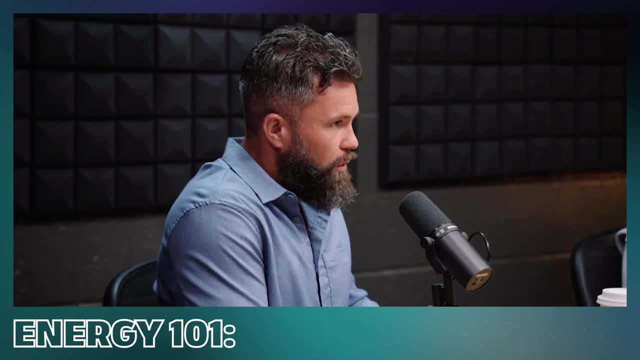 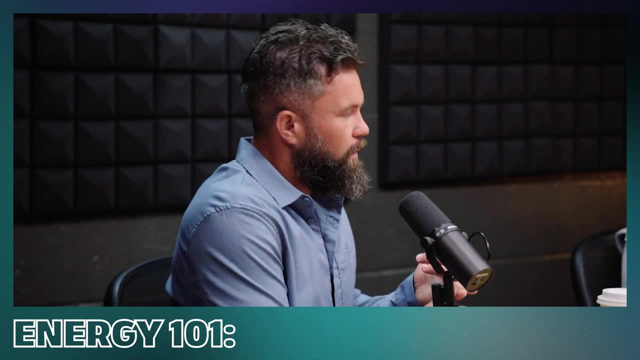 transport that material to these facilities, and then those facilities break up that oil and gas and then sell it to consumers, being, whether it's chemical manufacturers or, you know, electricity companies like- and again, there's a lot more in between, but that's. 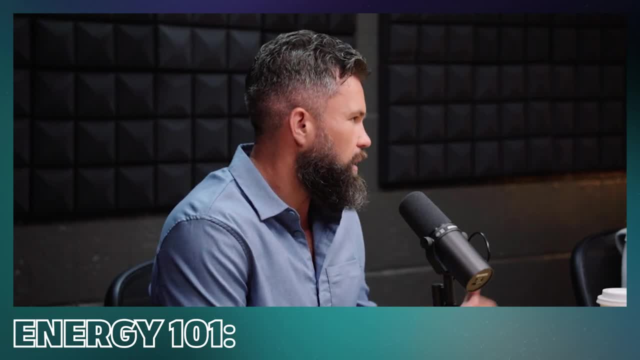 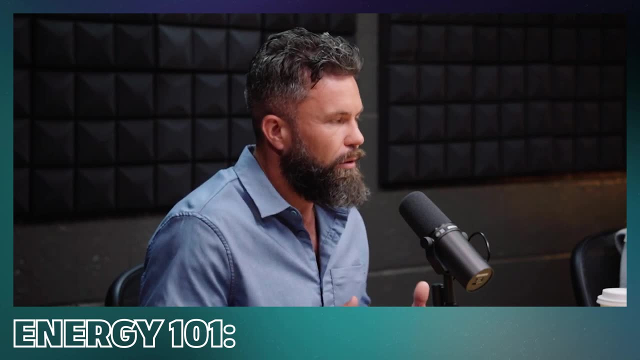 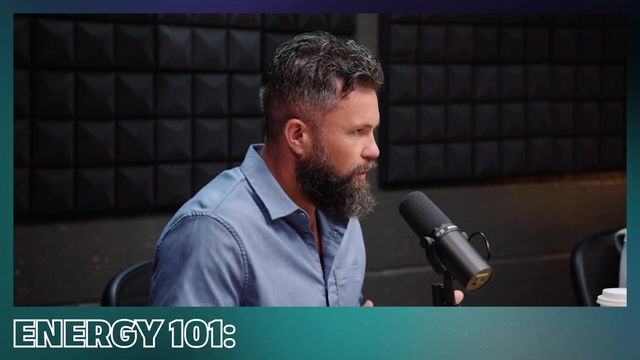 like very high level, how that happens And then, like talking about the utility size is you know, yeah, we're not to get into utility markets and power markets, but ultimately, you know, natural gas, Natural gas is is a big component of how we, you know, create power and there's natural 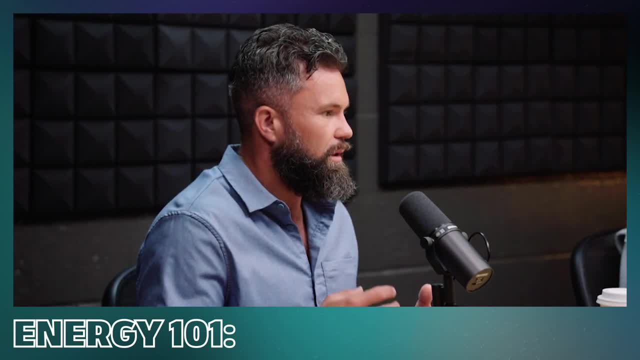 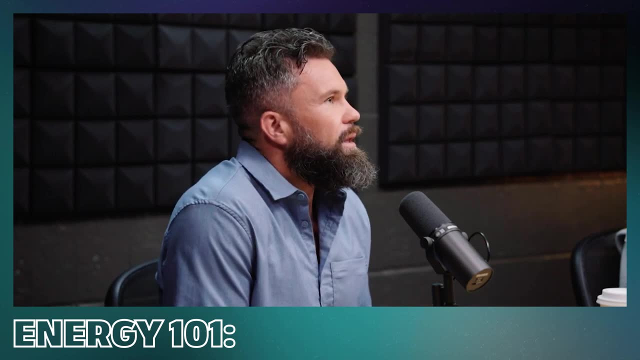 gas process like power plants, And so the gas comes in, it turns a turbine, and then that turbine creates electricity, which then they sell it to the market, and so on and so forth. So but like that's stuff that the average person would have no idea about. 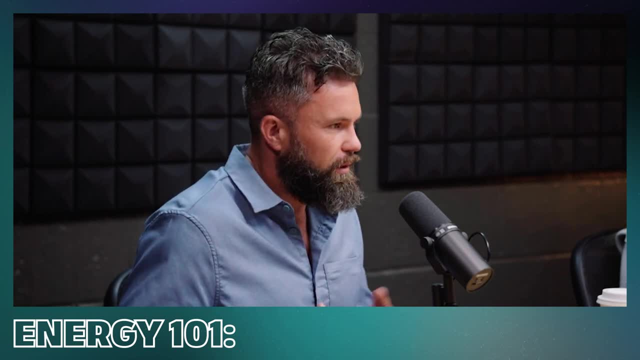 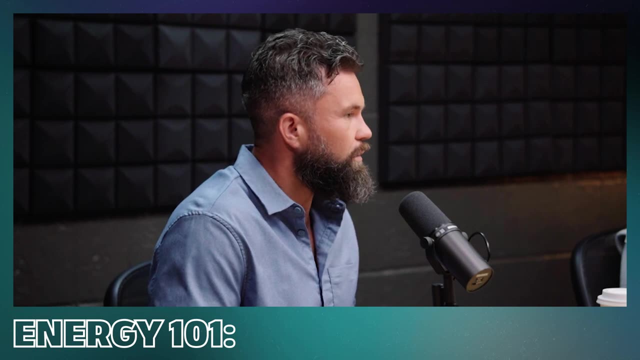 But ultimately, when you you can always reverse, kind of explain it too, is it's like: okay, so you know. do you have a phone? Yes, Okay, How do you charge it? Well, electricity, Well, do you know where that comes from? 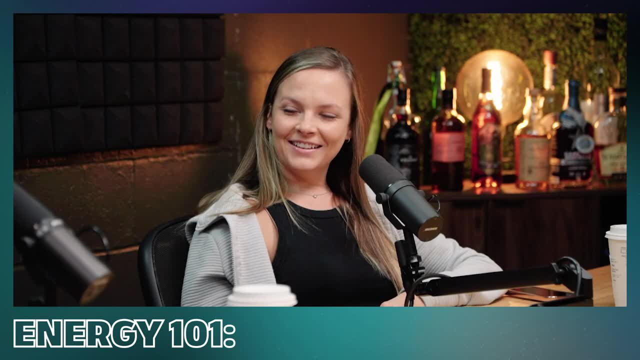 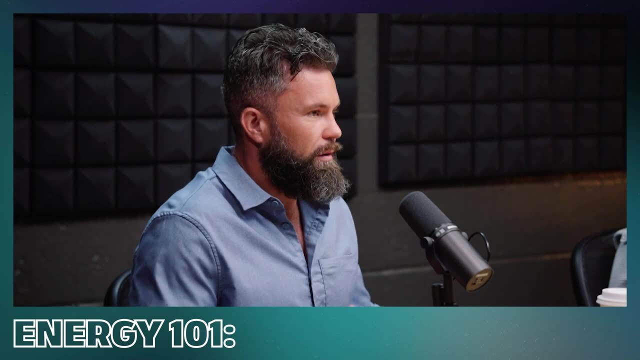 Well, the wall, The wall, Yeah. And then it's like, okay, well, like, there's these plants that create the electricity, and in order for them to create electricity, they need some form of energy. and that energy comes from, you know. it could come from wind, because, ultimately, electricity always comes from turning. 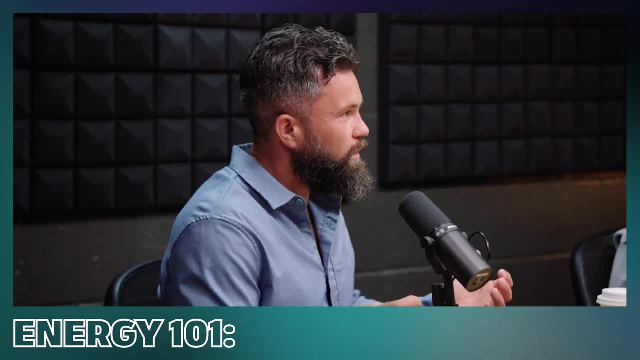 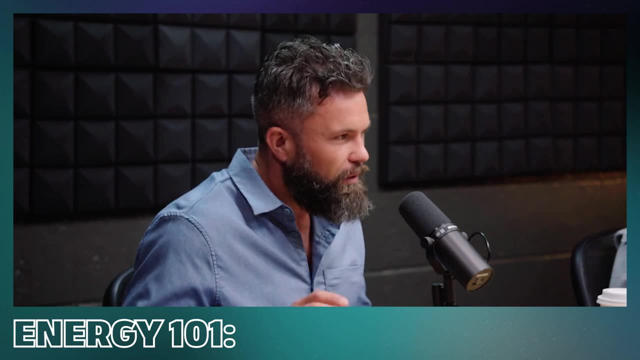 turbines right Like so, whether that's through water, like you have hydroelectricity and you have, you know, wind turns the turbines. nuclear power is kind of different in itself, but that's a lot of times It's like kind of reverse explaining it. 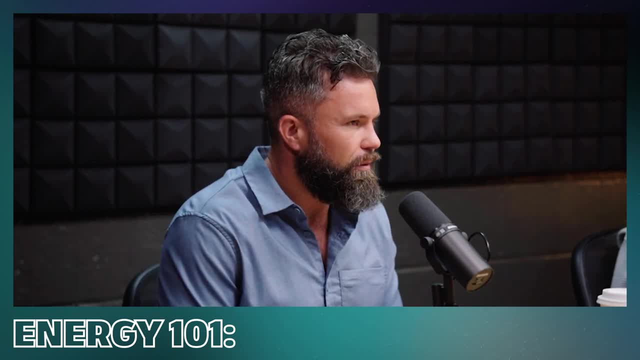 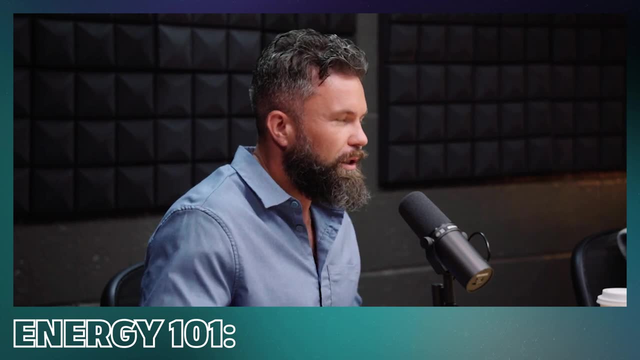 And then like for my daughter- actually, you know, this is a good topic for parents who have kids who are trying to explain energy And like one thing that we've taught our daughter- my son's not quite old enough to digest it. 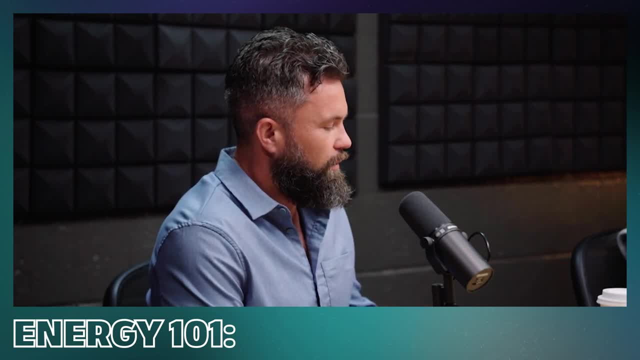 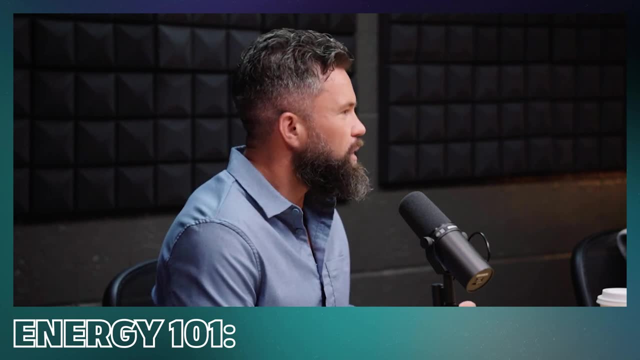 but she knows now is like the critical parts of life are food, water and energy, Like that's what you need, And so she understands where food comes from. She understands water, but the energy one was like you know, and so it was like we. 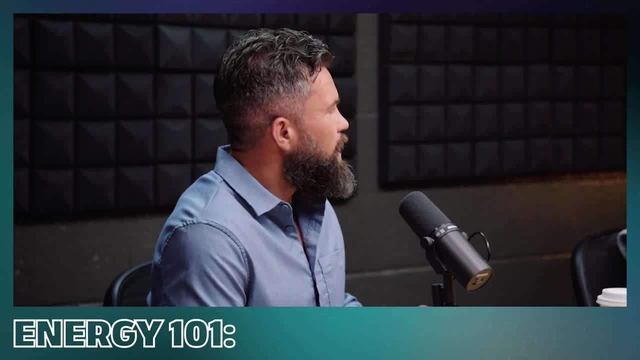 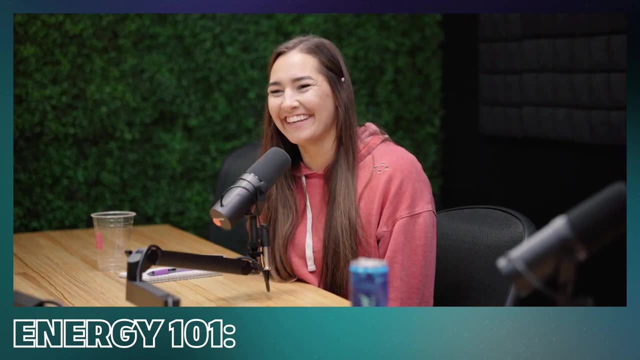 started with the wall. It was like, okay, you have your, your light or whatever. And then, cause she doesn't really know what I do except for work on a computer and talk on the phone, I was like, well, the reason I do that is because blah, blah, blah. 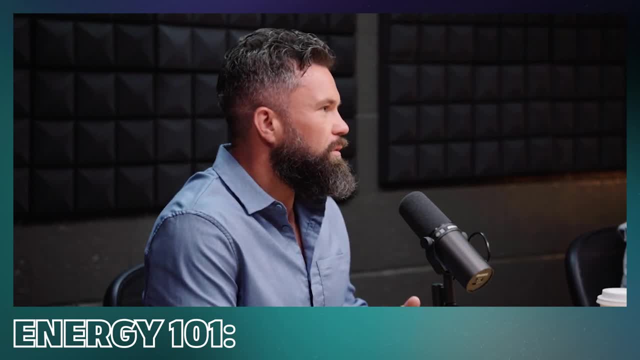 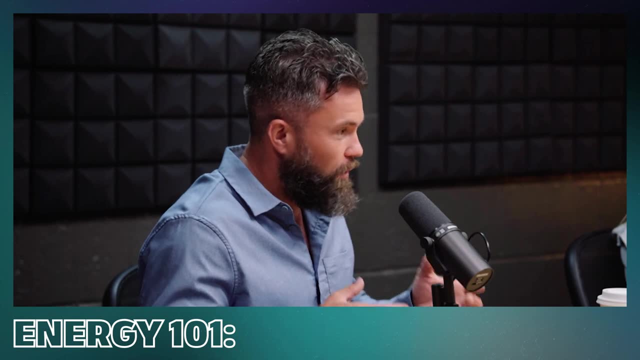 But you know, she understands now that without daddy drilling holes in the ground we wouldn't be able to drive our cars. And I say when I daddy drills the holes and then this stuff comes out of the ground and we put that stuff in the vehicle and she's like, oh wait, that's important. 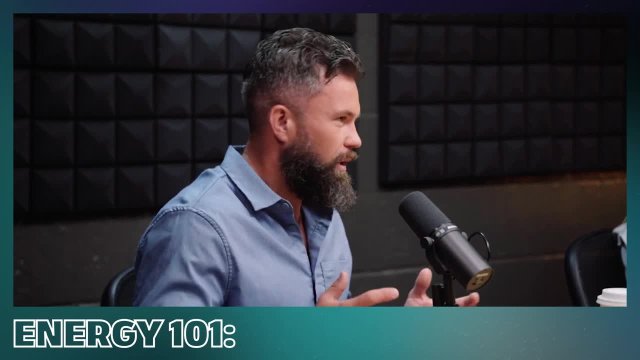 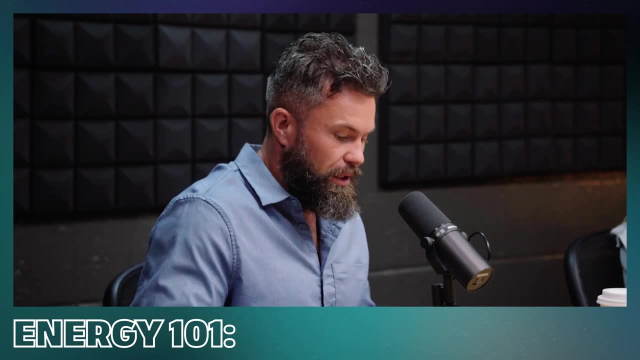 Yes, it is until we go fully EV. But you know, then we explain: okay, well, you need electricity. Well, where is the electricity? You come from? the electricity comes from the wall and there's these big machines that make electricity. but in order to power the machines, you need the stuff that daddy gets. 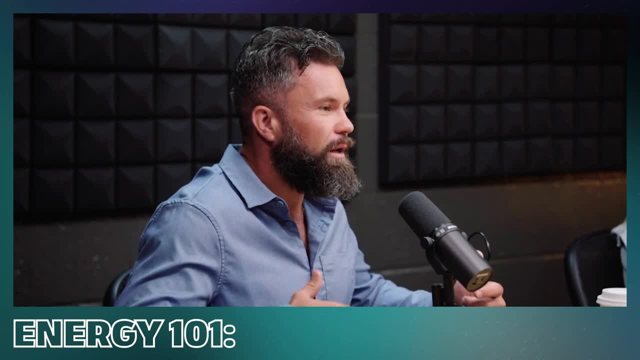 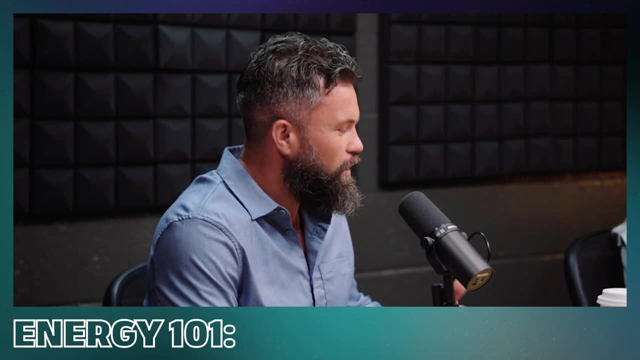 out of the ground And so she's like connecting the dots. and you know, as we evolve we'll explain more of like other technologies. but to like that's if you can explain it to a six year old, hopefully you can explain it to another adult. 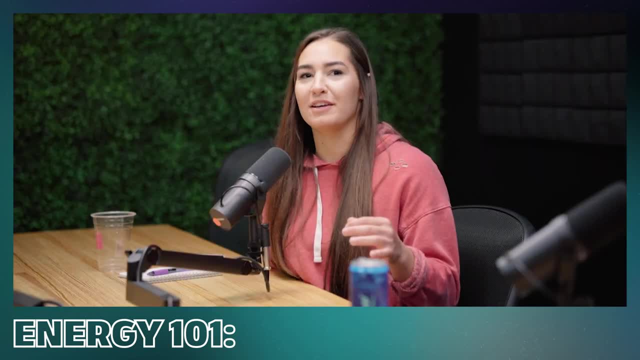 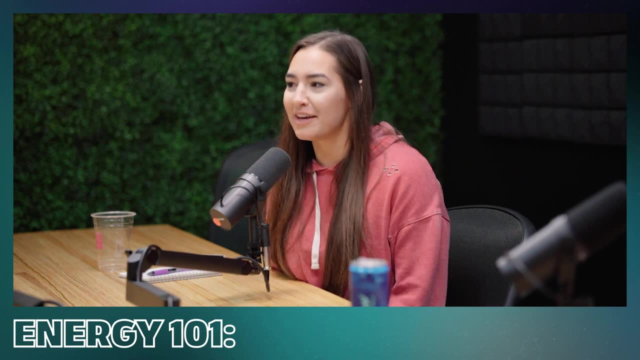 Yeah, I think the hardest part of understanding it is like you can't see it. Like you see your food, you see the plants, that it grows. Not everyone is, um, you know, from Midland Texas. you don't get to see the rigs that. 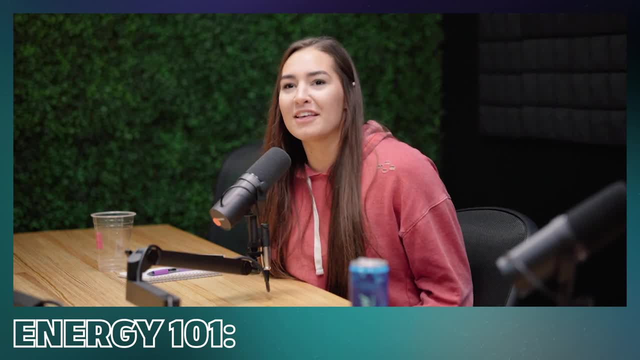 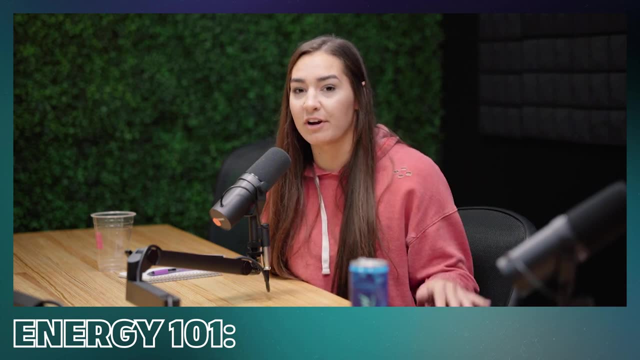 actually drill or the pump jacks that are pumping the oil. So I think that's where it becomes like non-existent to some people who don't see any energy infrastructure at all. Um, and so it's interesting that you brought up like two parts. 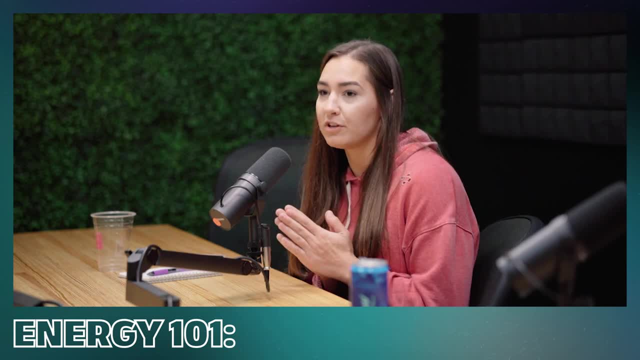 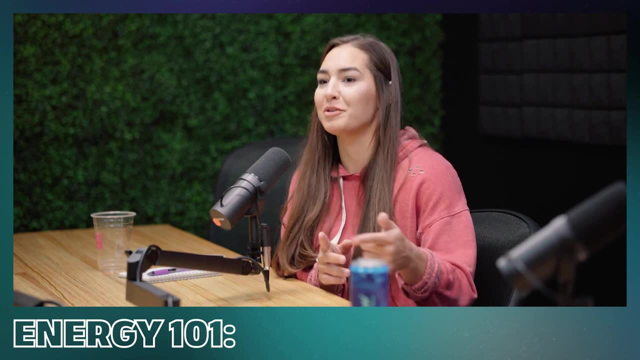 So, yes, we had on our last episode Kay McCall, who she divided up energy into two parts. One was power, Yeah, Which is your turbine, So any wind, exactly what you're saying, Yeah, And the other side of it would be- I can't remember what she called it. 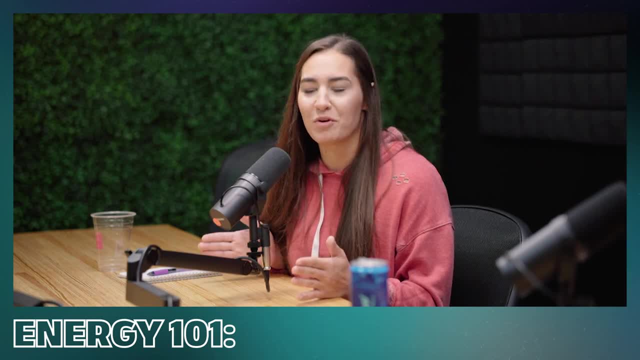 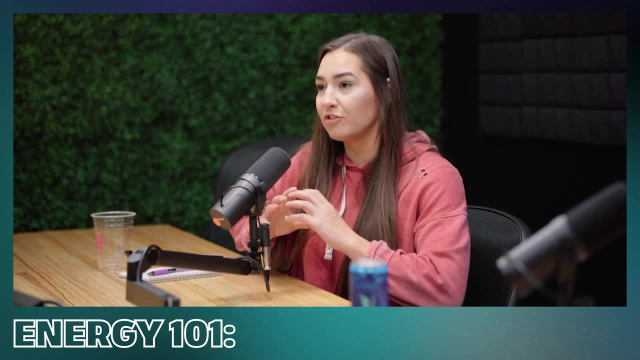 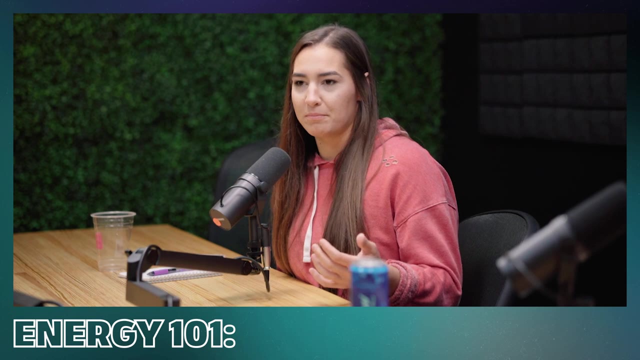 I don't know if y'all remember, but basically oil and gas. like what else do we make from that? Like aside energy, aside from like power generation? Okay, Um, which you kind of already touched on, like we need petroleum to make all the things we. 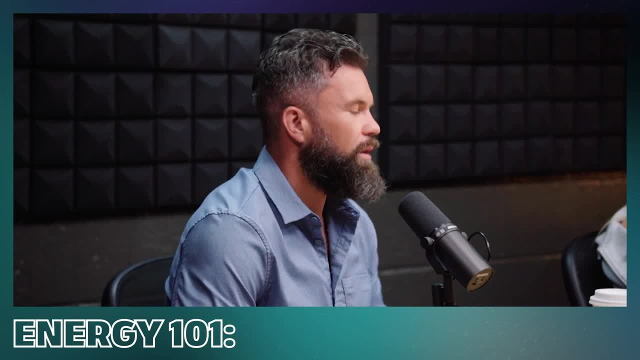 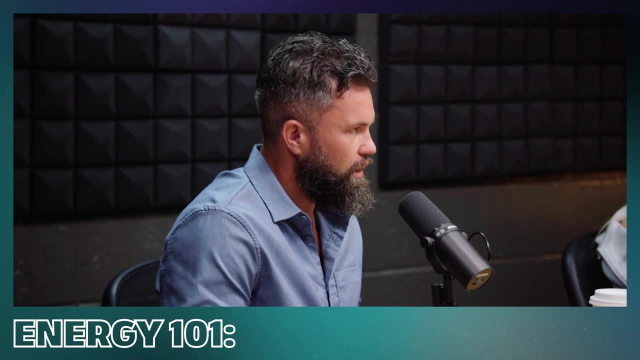 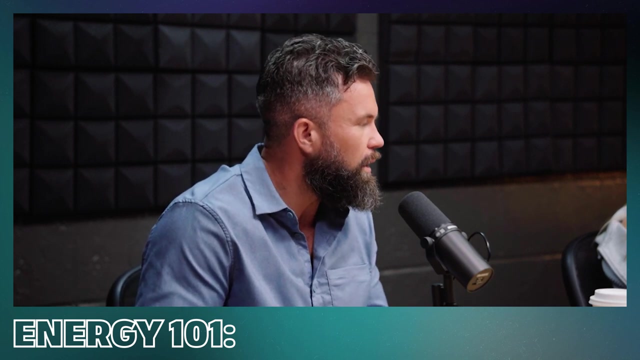 use. Right, There's Yeah, So I mean. so the energy side is. I would consider the energy side of it as like power and electricity. That to me, when I think energy, that's what I think. However, there's another component, the petrochemical side, and the petrochemical side is extremely 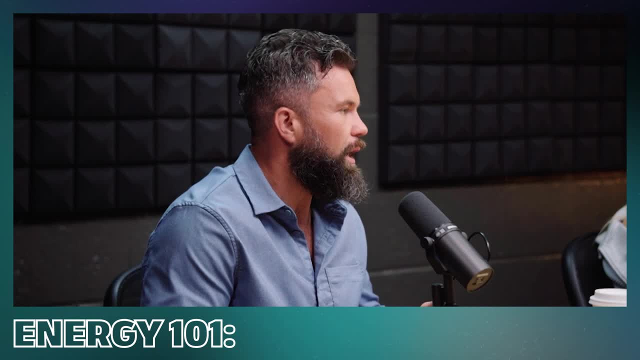 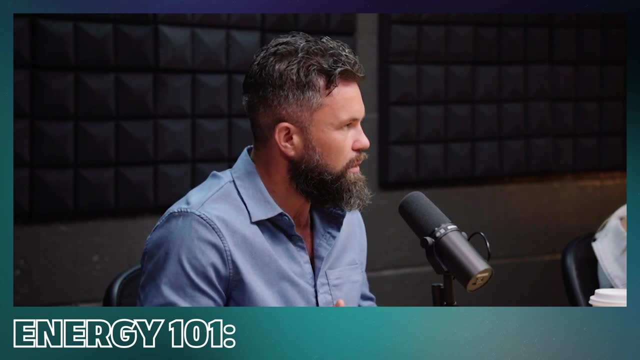 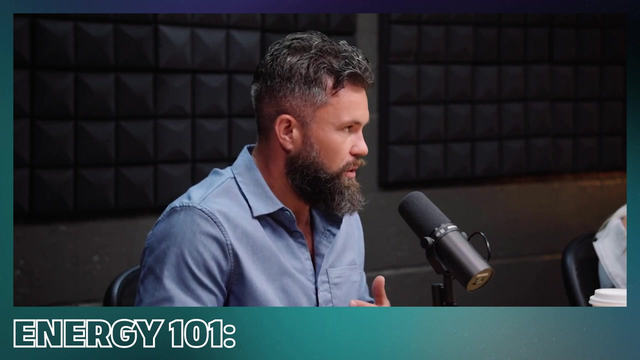 important And that's where I think you're going to see a lot of demand growth on the petrochemical side. Um, you're going to need a lot more of that because you're creating more goods Right As as economies continue to evolve- the demand for energy and demand for just overall stuff. 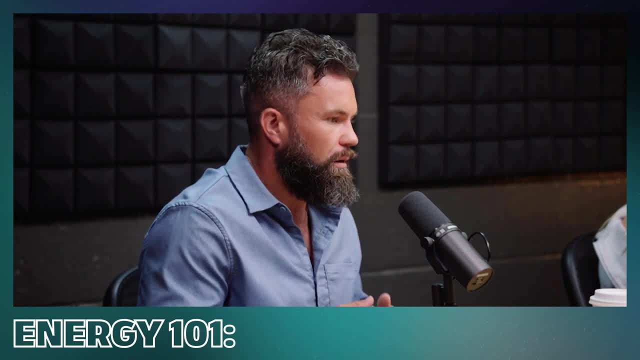 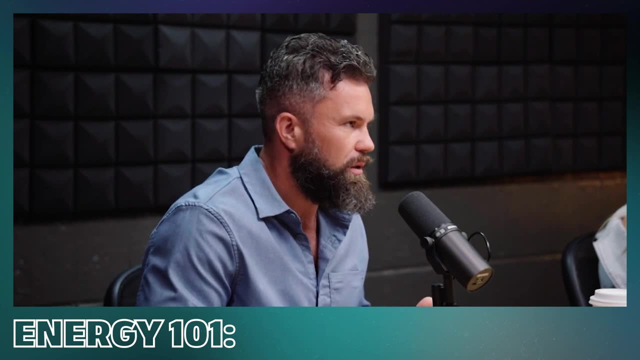 that we see and use every day increases, Um and arguably, like the world's economies are continuing to grow. you know again that's debatable right now but for all extents of purposes you have emerging economies like India and China and stuff that are just continuing to use more stuff. 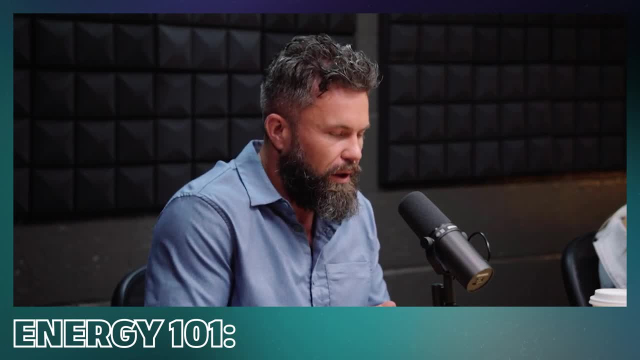 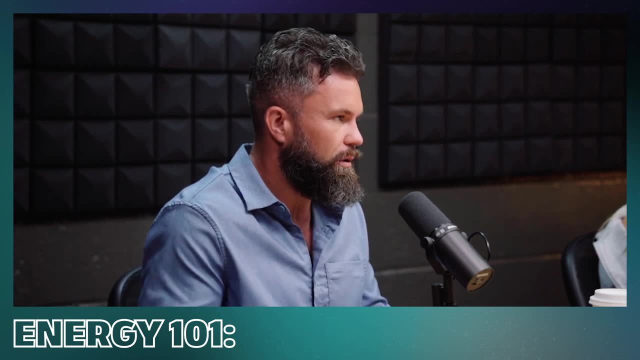 So, in order to create more stuff, you have the other side of of the energy industry that helps. Uh, you have the other side of the energy industry that helps create feedstock for a lot of, and feedstock are like materials. So when you extract oil and gas, there's byproducts. after you separate it through heat and other 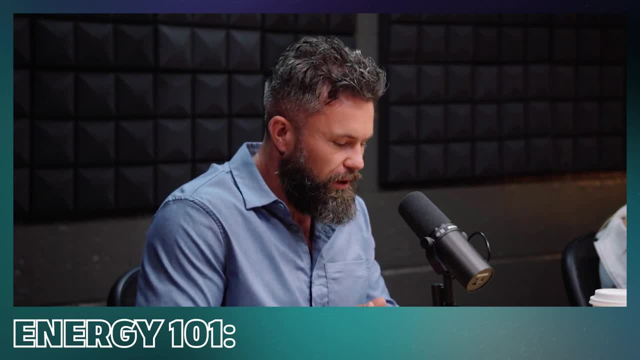 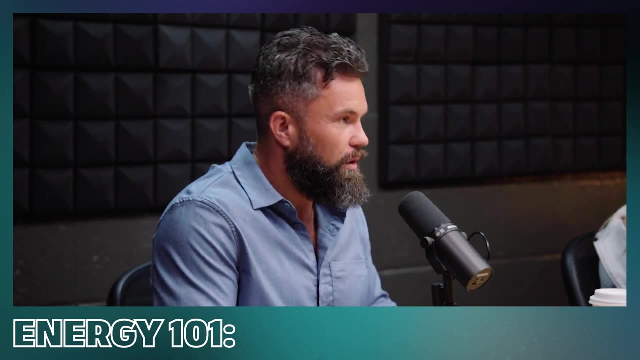 forms of doing that. But again, in in gen, speaking in very generalities- you have when you extract stuff out of the ground. you can use some of that to use to to create electricity, And then you can use a lot of that for whether it be fertilizer, whether it be, you know. 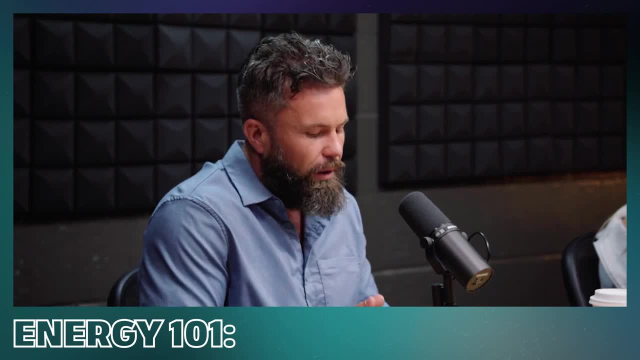 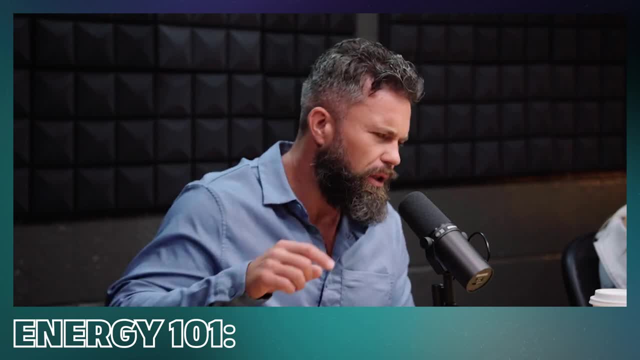 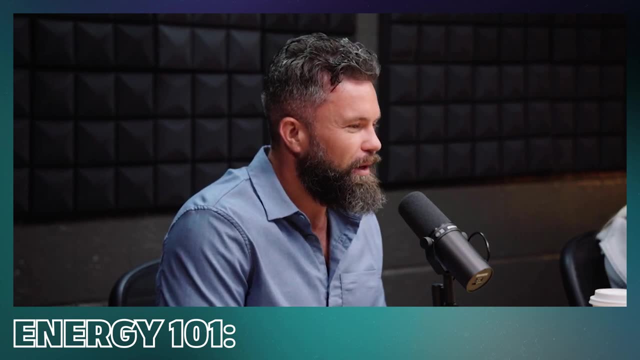 you can break it down further and anyone who's listening is probably like: well, yeah, but this, yeah, but yeah, like i know everyone you know, like, take it easy. um, i'm trying to keep it very simple. um, i think that on that point, that is where, um, the industry really lacks, like they like to. 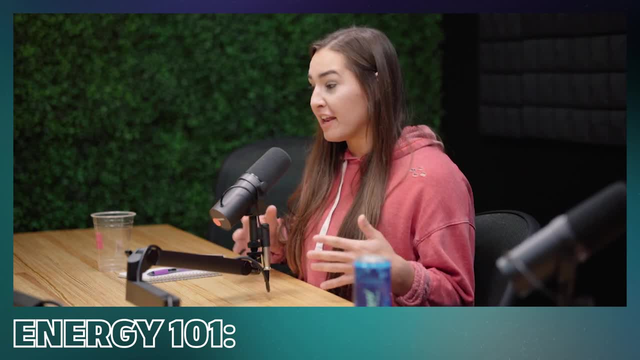 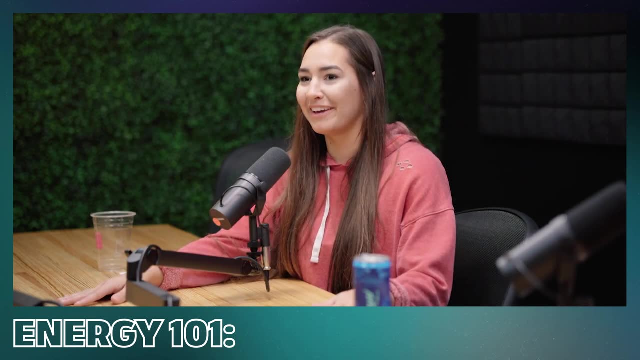 over, complicate the way they explain things because it is very in-depth and technical. but you can't you. if you were to tell me all the technical stuff, i'd be like yeah, okay, bye, yeah, but yeah, yeah, it's interest, so you have to keep it high level. so you do. you notice it like? 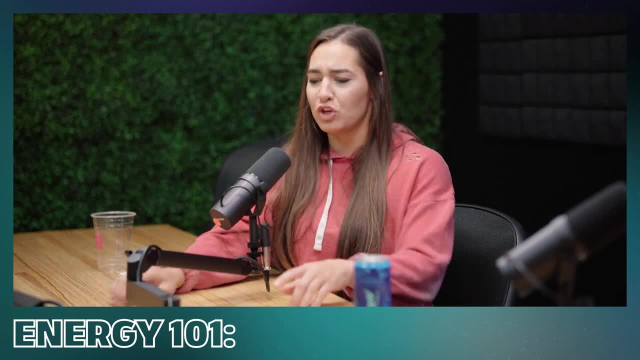 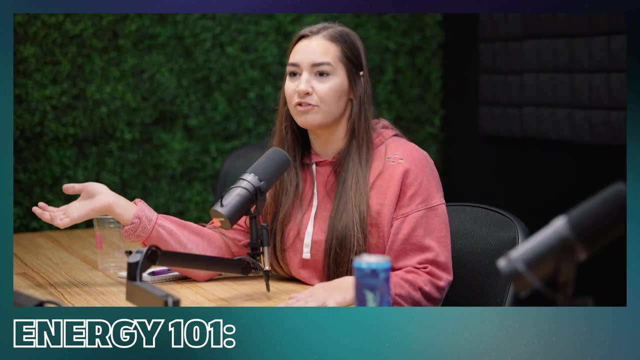 on tiktok, colin will make an explainer video and they, like you mess up this, like actually it's this and it's like that's not the point and that it doesn't matter to people outside of the industry and that's ultimately who we need to talk to, right, yeah, and and like whether it's you know. 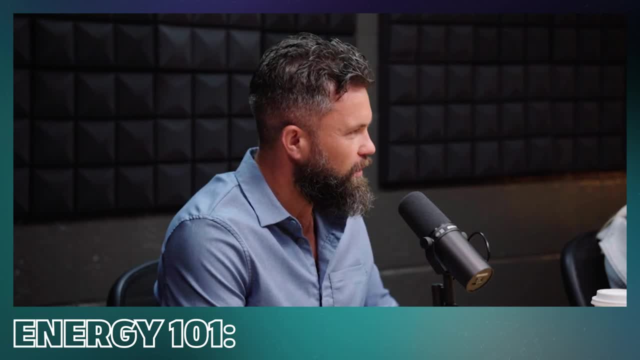 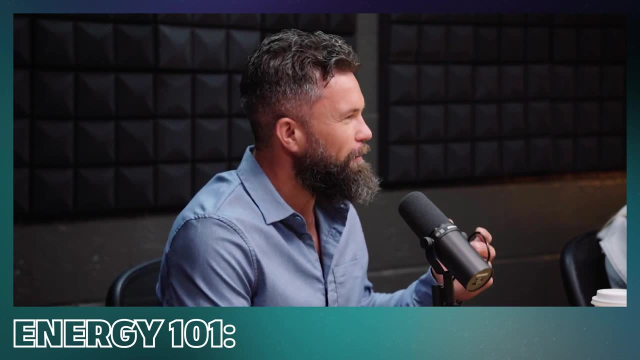 because, again, everyone claims to be an expert. like you know, tiktok is a great example, i so i started this little tiktok account which i go on there and i just like speak my mind, like if i think it's something, i'll go on there, i'll say it, and whether it's like 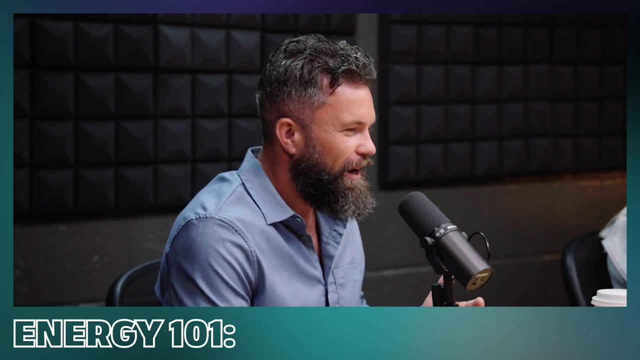 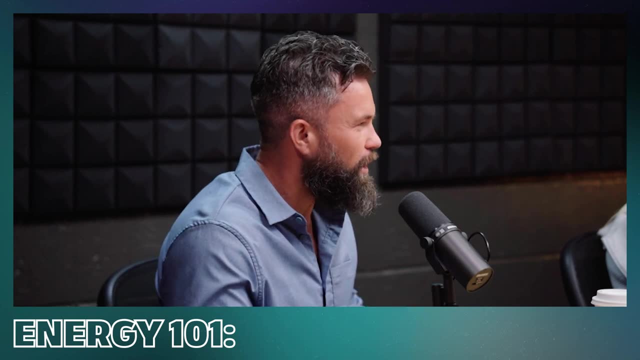 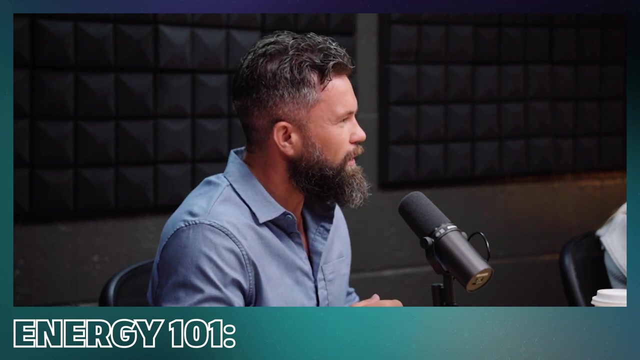 talking about oil and gas, markets, sales, anything, and i was in. this is the funniest thing. so i was in, i was in colorado and uh, i was in frisco, colorado, so up in the mountains, and like for 14 chicken wings was like 27 or something, and so i. so, of course, i was like, oh, that's crazy, i take. 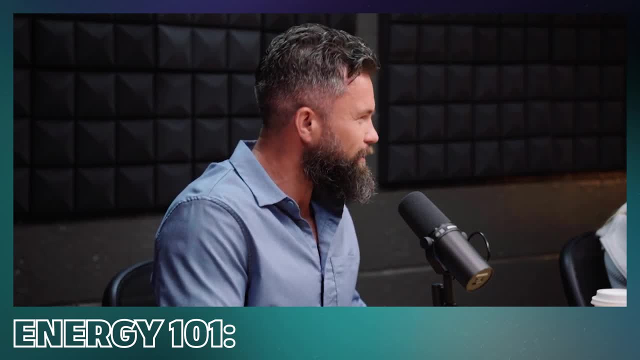 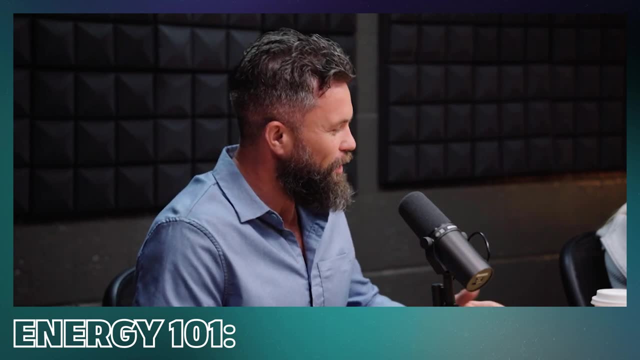 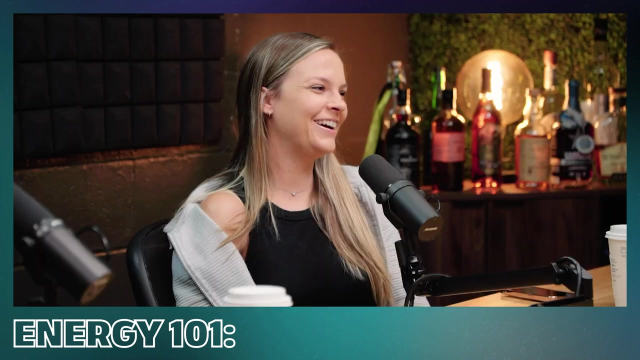 out my phone. i'm like do a tiktok thing. i'm like 27 for chicken wings- are you fucking kidding me? and like just kind of joking. and then i i was not expecting this, but like so many people went on there and were like thanks, biden, like biden this and that. like everyone like started getting so mad at like 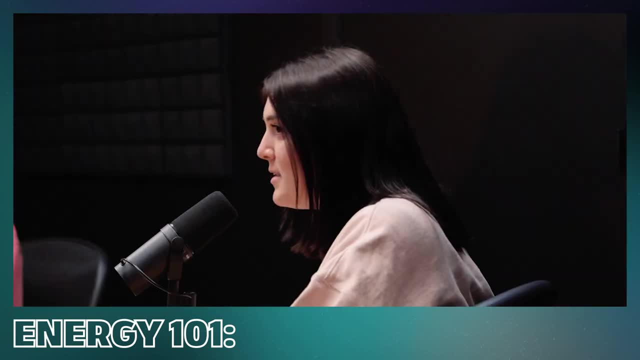 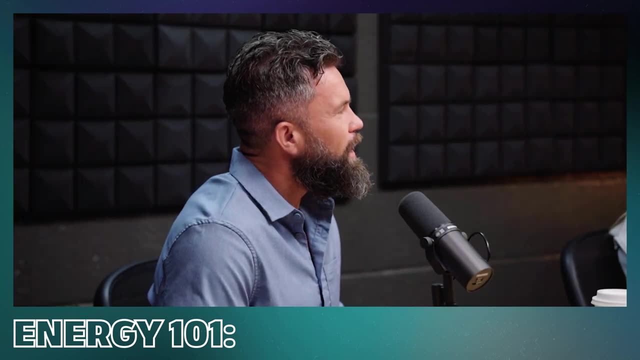 biden over this post and i was like, okay, like, the comment section on tiktok is wild. yeah, that's where all the juice is right. yeah, so, but so then i? so then i started replying and i was like, well, i have a hard time thinking that, like biden is single-handedly causing chickflation, that's what. 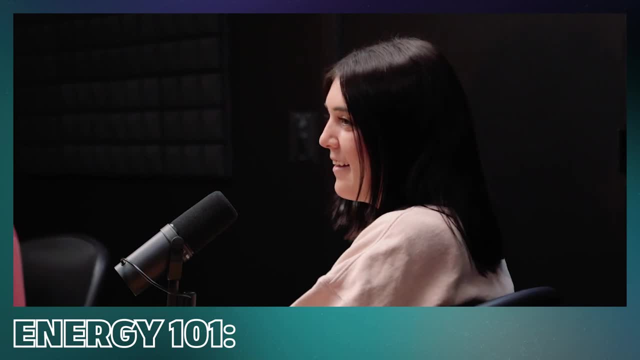 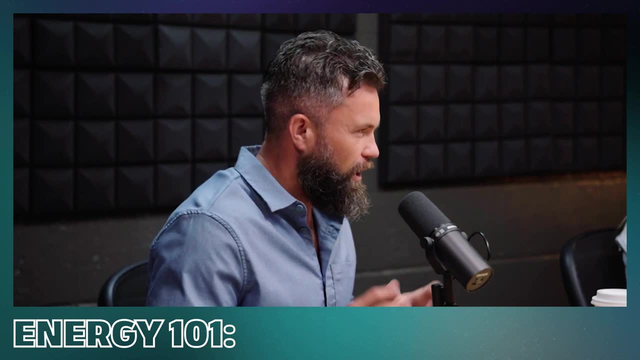 i was calling it and so i mean yeah, and so then i like made another post. i'm like okay, like to clear things up, like yeah, i get it, like everyone is is an economist now and you know, everyone understands inflation and everyone's an expert. but like, let's consider supply and demand here. 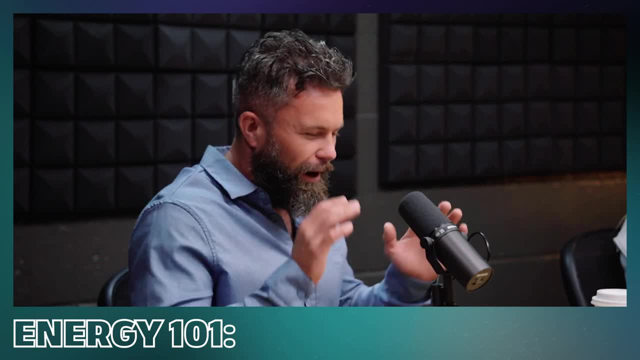 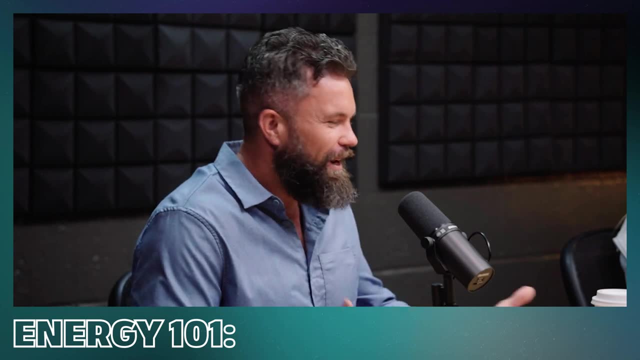 and then everyone was like no, but this and that. and then i was like okay, i need to stop. so i like totally stopped responding. but to the point of everyone's an expert, is this like yeah, and like man calling for doing that, like he's talking about like random components and different things within. 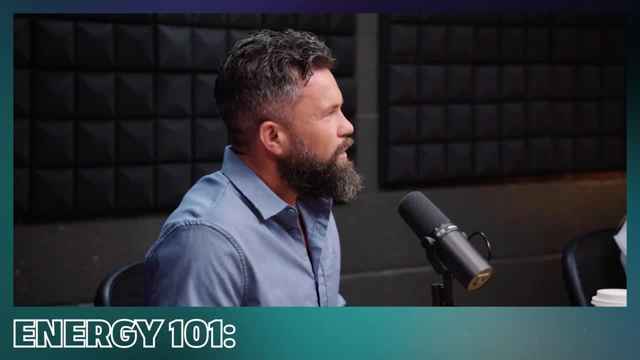 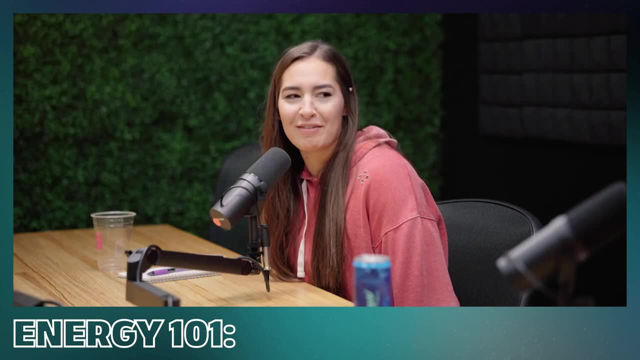 and then like educating people and to go on there, and then like try- and it's a term down here everyone i guess knows, but i learned this recently out: whataburger, somebody is that? have you heard that? i've never heard that. oh okay, well, when, like when you go, like you know, one uppers, yeah, like i'm. 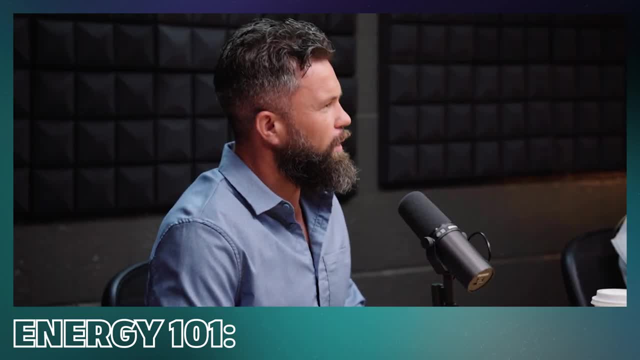 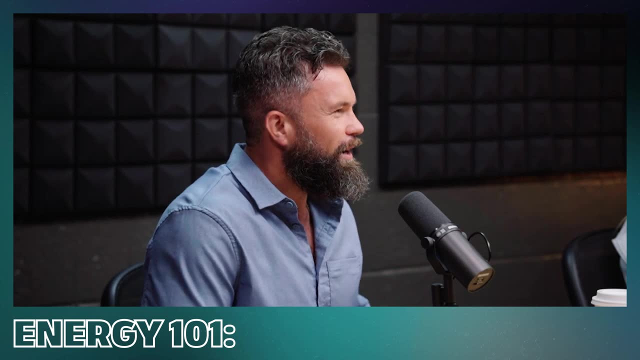 gonna one up you. it's like if you went to a concert, well, the concert i went to was way better, like you should have been the one i was at. well, yeah, everyone like seems to think that, like their comments or what they know is that much smarter, um, but ultimately it's like it doesn't matter. 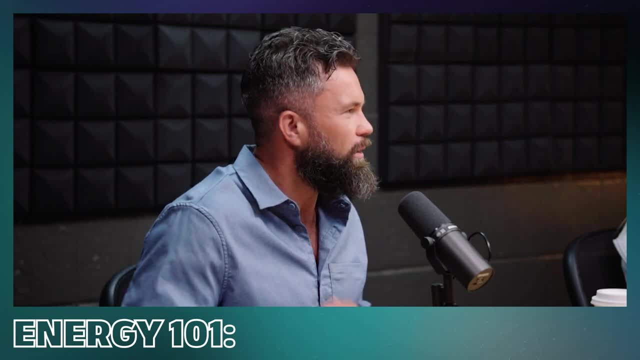 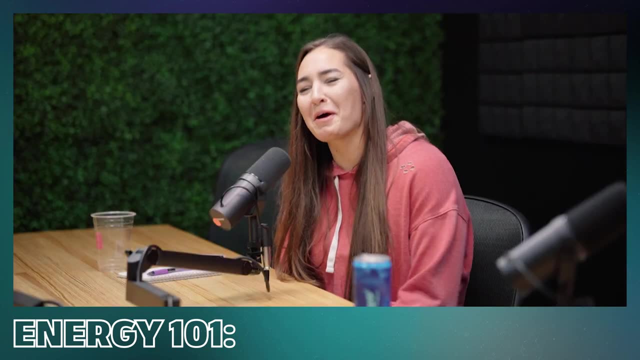 like the fact that, like, unless it was like completely off scales, like if colin was talking about like a wind turbine that you used to drill oil and gas for, i'd be like okay, like maybe you can correct course here, but like to get into the nuances and the details, it's like he's not trying. 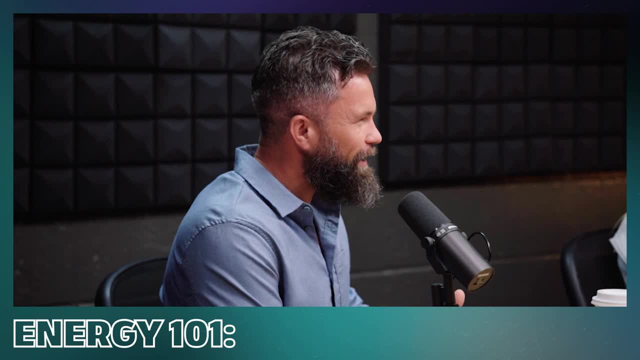 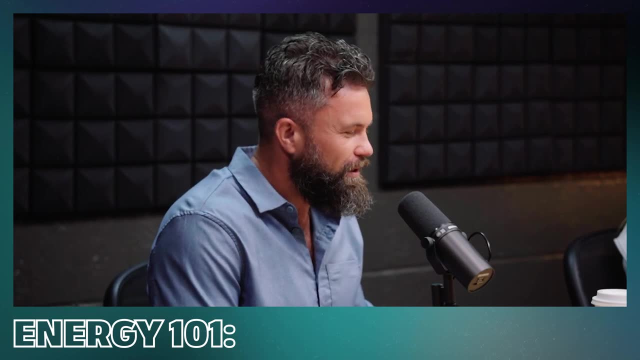 to teach a like a graduate level engineering course. he's trying to help people who don't understand the industry and like, so let's not get caught up in the, in the semantics here. um, but yeah, it's, it's, it's crazy and, to keep it high level, it's again that that is a great point is. 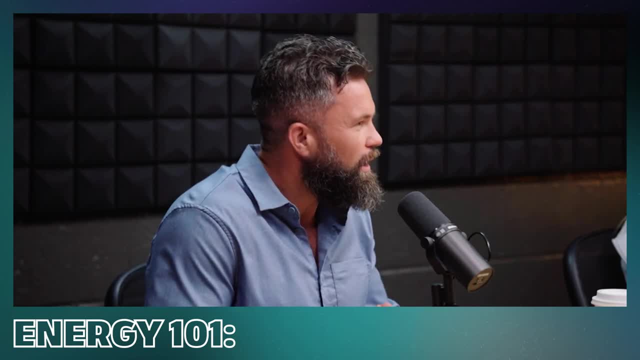 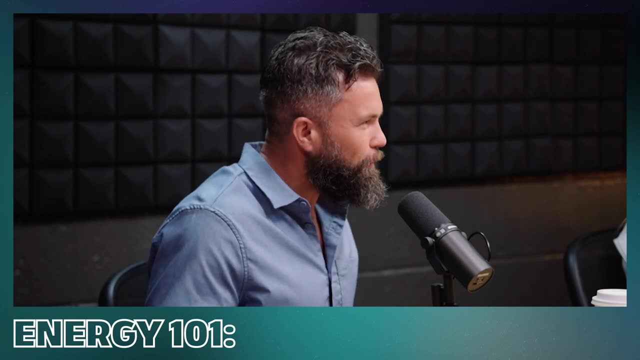 we have a hard time in oil and gas explaining what we do, um. but then you have all these scientists and engineers been like i'm gonna show you how smart i am. it's like no one gives a shit. they just want to understand what's going on like. can you not simplify it please? yeah, yeah on that. 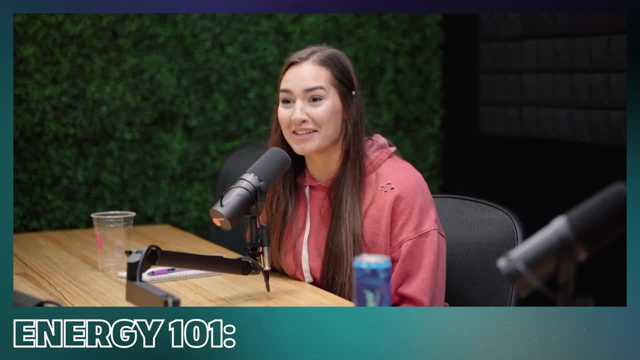 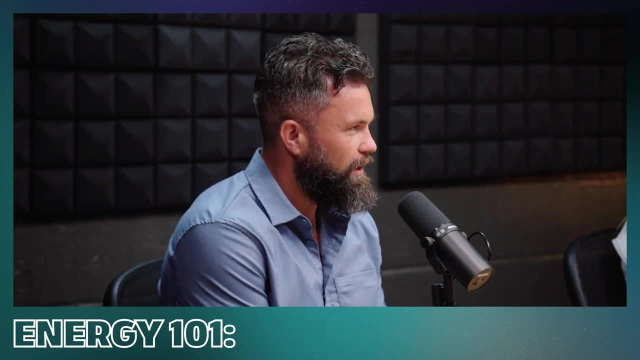 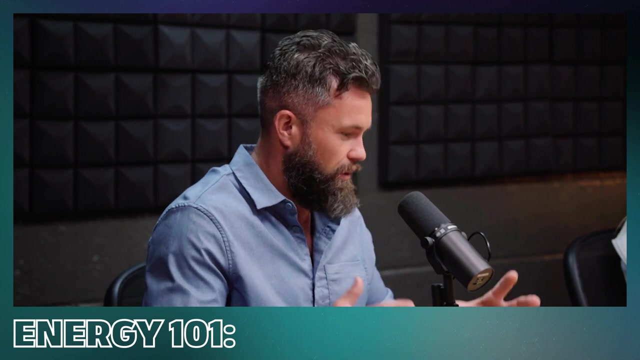 note. gonna like do a little test. can you simplify what you do to us? uh, yeah, so when you drill for oil and gas, i'm gonna assume people understand what drilling is. that's fine, okay. so you, yeah, you have this big machine that sits on the on the dirt and it drills down to get to the pool of oil and 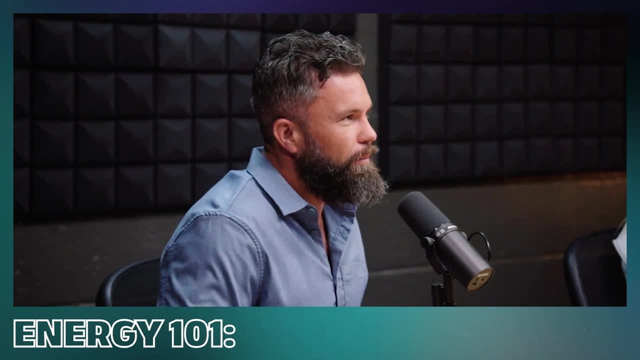 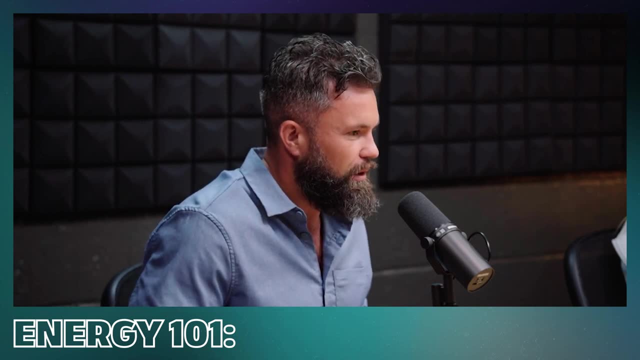 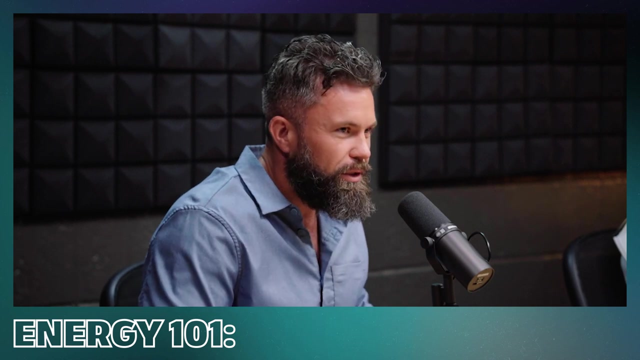 then it just gushes everywhere. right, like that's okay, so, but in order to get there, you need a fluid that is pumped down to where you can. if you're in a like that's good, let's go to the beach. everyone close your eyes when you're digging to get to china, right at the beach, because everyone knows. 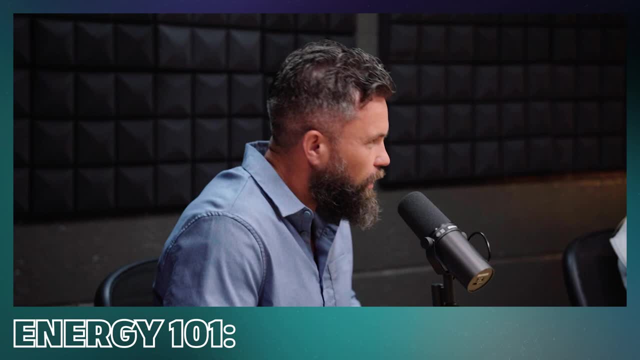 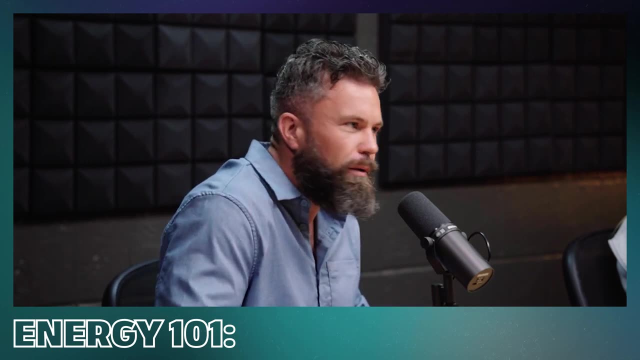 if you dig the beach, you're gonna die from that. you're really losing your 가지. that's a lot of even up. you can get to china. what happens when you start digging? what happens? the sand gets wet, yeah, and then what happens? starts to fall in right like you dig, the more. i've never done that. 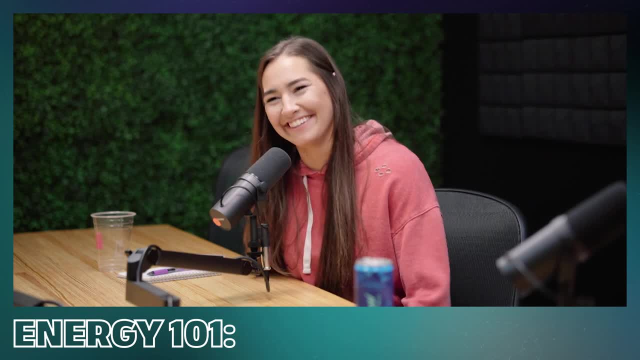 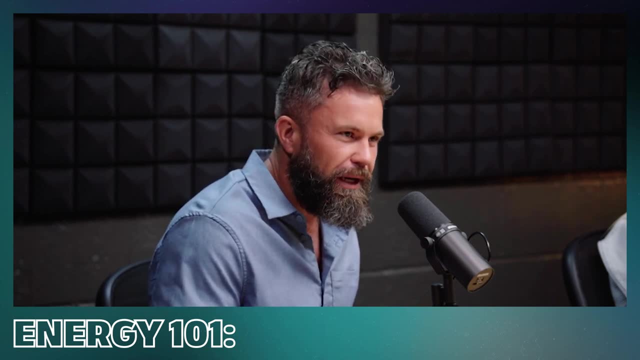 i'm like, i'm like what happened? i was just at the beach and i'm like what happened? so so you dig down. then all of a sudden, you get down there and and then the the sand wants to fall in and you're like, well, i can't see china yet. so you keep digging and just china never appears. but if actually, side note- if you dig deep enough here in texas to get to where you can dig to china, you won't actually get to china, i thought, anywhere in the world. if you dig deep enough, you just somehow end up in china. but apparently not. i've never heard that. no, okay, well, maybe that's. 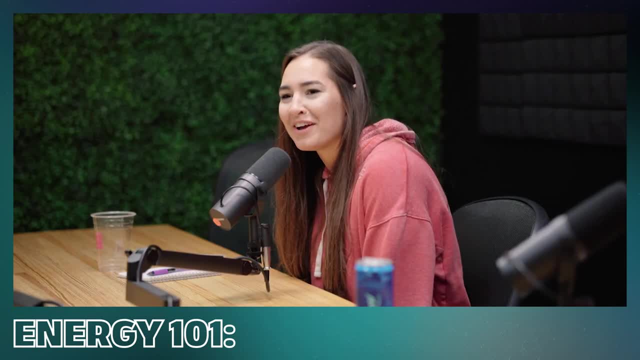 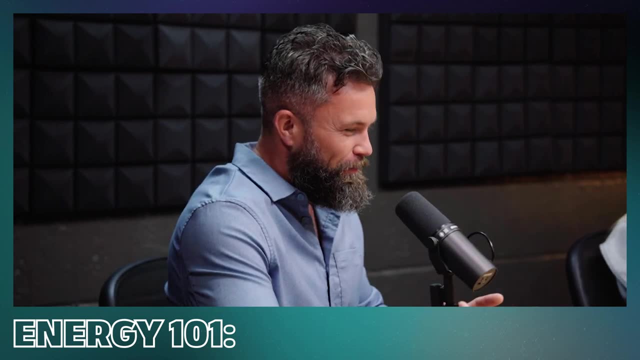 a canadian thing. no, i've heard that. okay, thank you, i'm not that crazy. it's not actually true. right, no, you're right, yeah, no, these are the questions that are not dumb. yes, if you dig deep enough right here in houston, texas, i don't think you'll end up in china- uh, although it'd be funny. 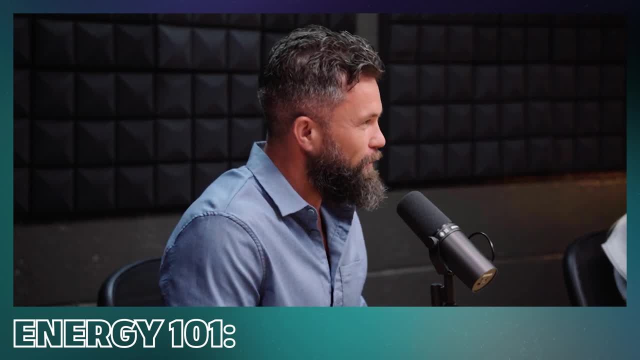 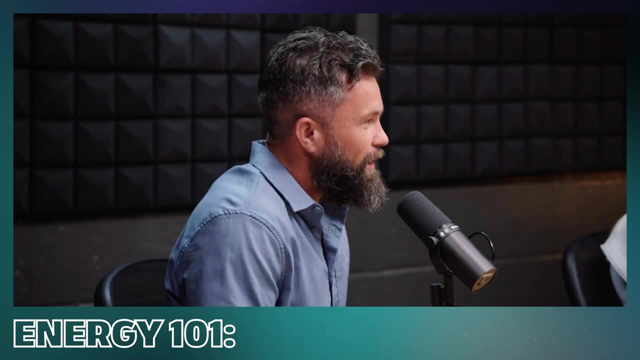 if you did. but i firmly believe that, growing up in british columbia, if i dug deep enough i would get to china. but i soon found out that if you dig deep enough, what happens is the dirt and the sand falls back in on itself. so how would you get that sand and dirt from falling in how you would well? 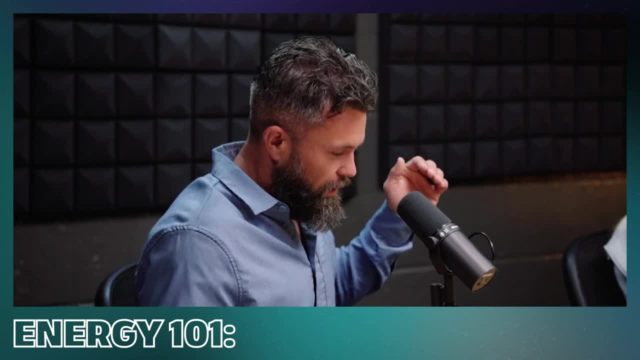 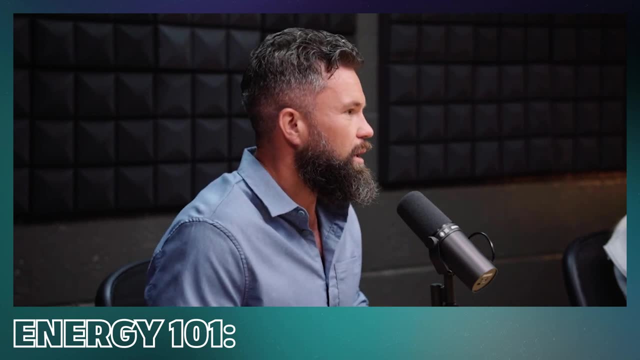 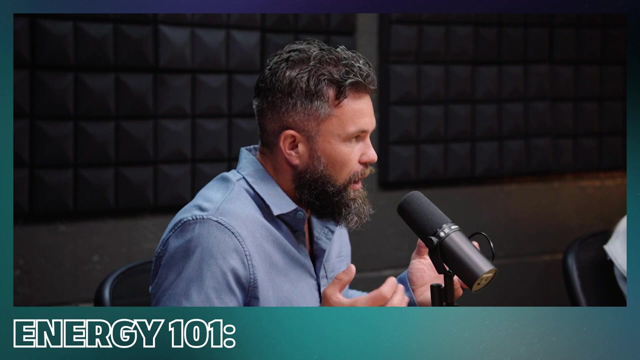 what i do is i provide drilling fluid, so i i provide chemicals in engineering on site, meaning at the rig, and we add chemicals to the fluid that gets pumped to make sure that all that rock and dirt can get lifted out of the ground so you can keep. 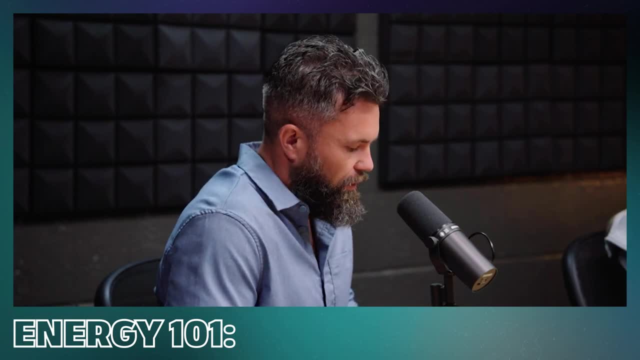 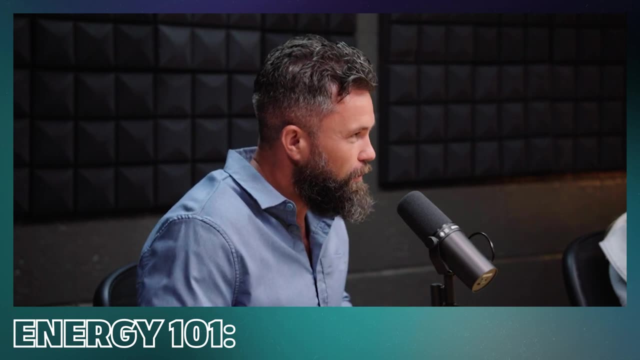 digging deeper, because if you just, like i say, if you kept digging now, if if your hand somehow had something that could like pump fluid and like kick and spray all that dirt everywhere, you might get to china. yeah, like at the end of your fingers, if you could shoot more, more water down. 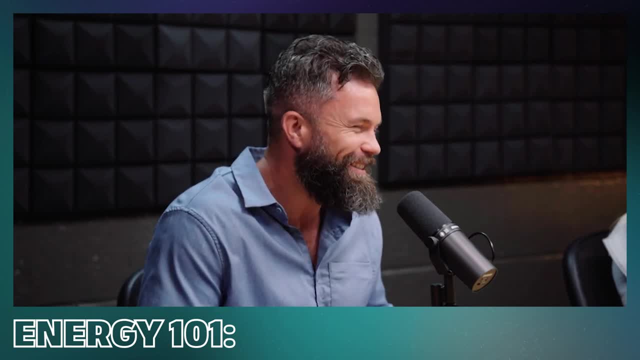 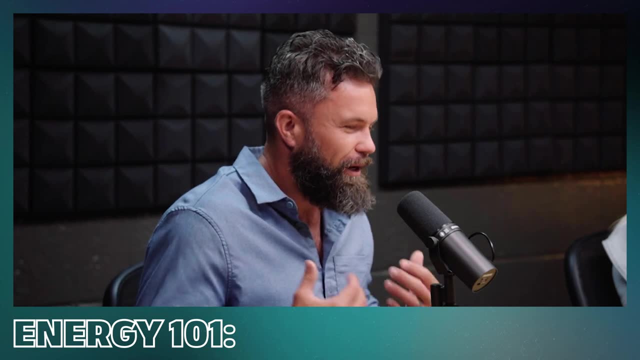 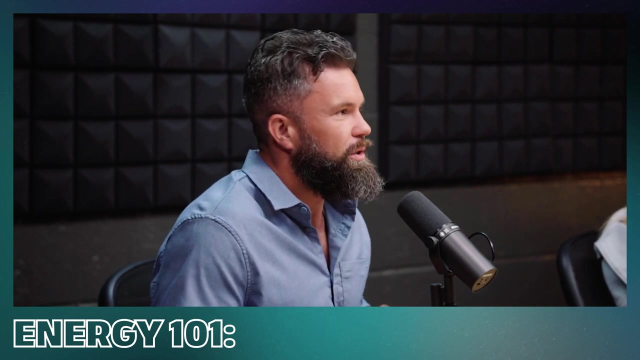 there you might be able to get deep enough to china, so so again. so, if you're digging- uh, you know, on a rig you're digging and you're drilling- um, i help provide fluid to where you can continue to dig, and and what happens is, as you get deeper, there's there's this phenomenon called. 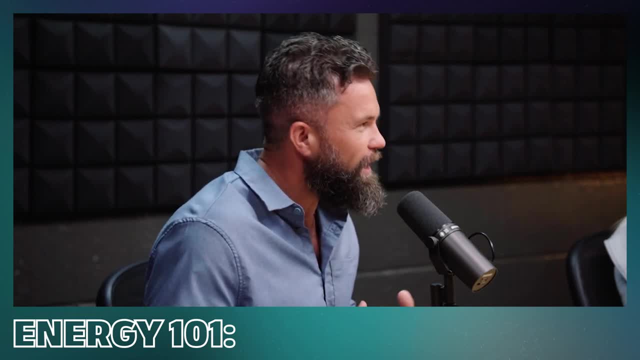 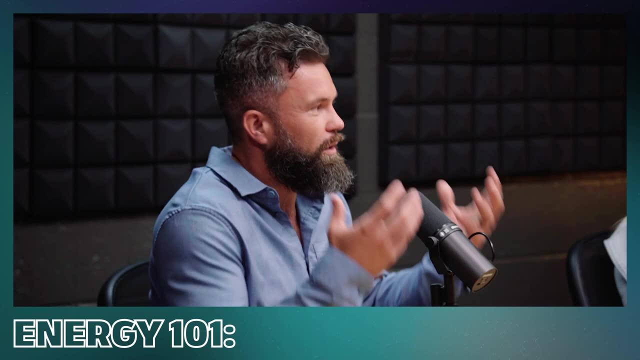 reservoir pressure. okay, and what that is is, as you dig deeper, the pressure one it wants to cave in, like the, and then that's how, ultimately, oil and gas gets pushed out of the ground- is because there's pressure. when you dig deep, there's pressure. now, everyone's not. well, what about? 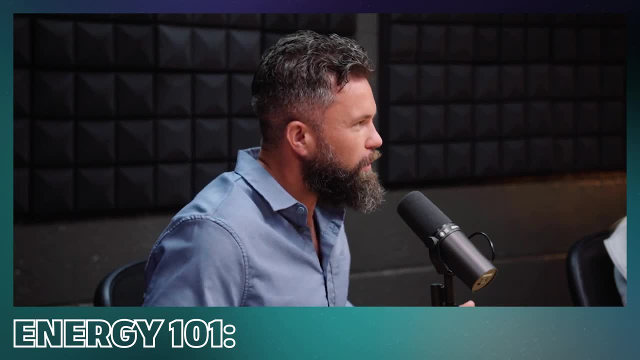 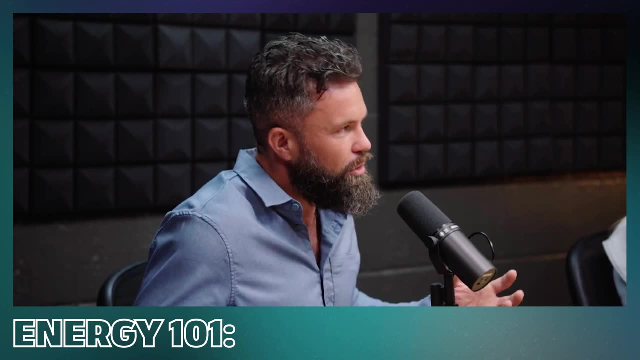 conventionals and sometimes it's depleted. yeah, yeah, yeah, whatever. but ultimately, the deeper you get, the more pressure there is. okay, so, but in, but in the end of the day you're digging deeper and as you're drilling you don't want all that pressure to shoot, uh, like fluid and gas back at. 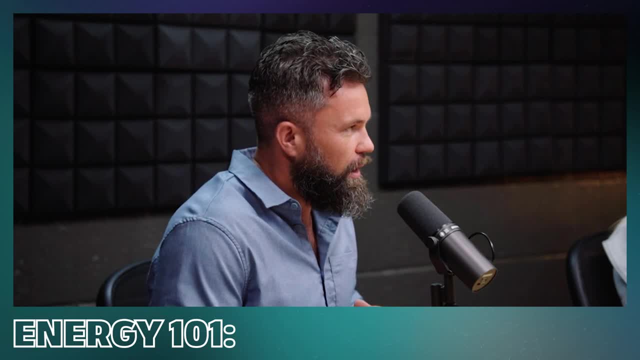 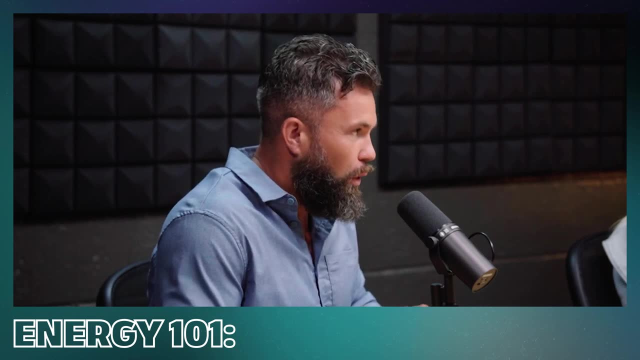 you because it's very dangerous. so the fluid that i provide has a certain density, and by that i mean it's heavy. so when you did, when you drill, it helps keep the hole open to where you don't have gas and oil shooting back at you, because you don't want that. you only want that when you're ready to. 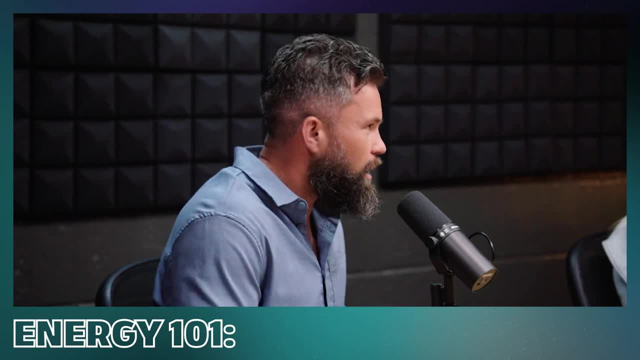 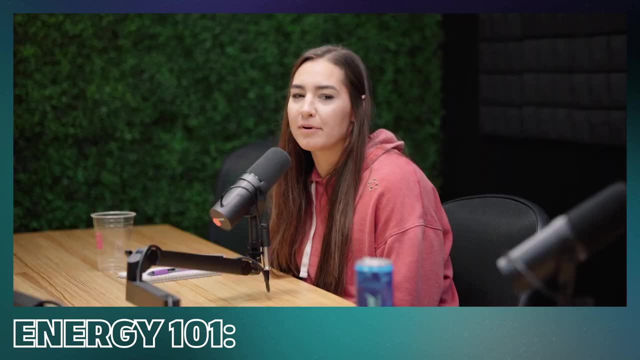 actually extract the oil and the gas, but as you're drilling to get there, you want to hold it back so that you don't have uh issues. so that's also part of it. suppresses and keeps the hole open. yeah, it keeps the hole open. so you 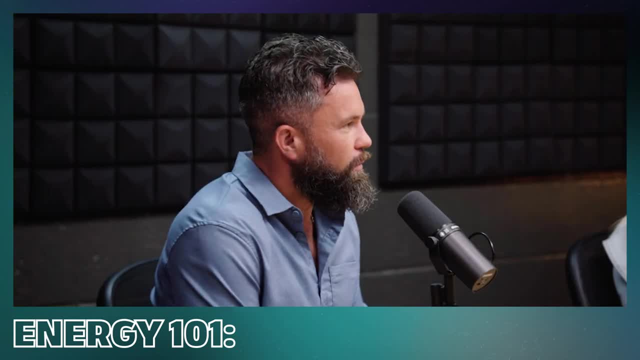 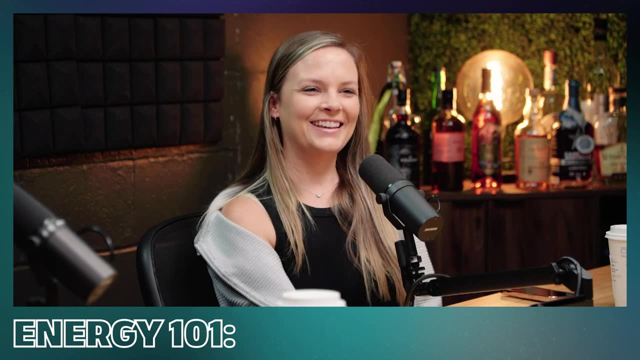 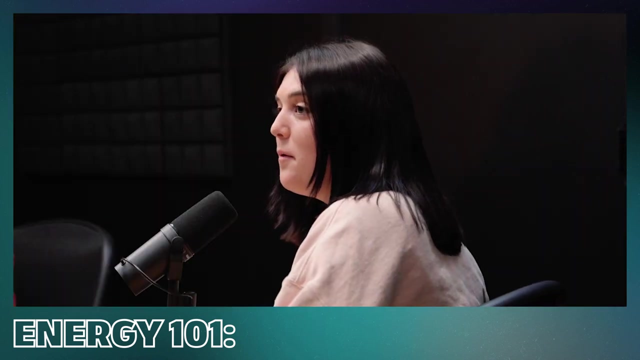 can drill to to pleasure island, which is the, which is the reservoir, which is the oil and the gas. yeah, the gold is, yeah. yeah, where the black gold is, yeah, yeah, okay, that makes sense to me. do y'all have any questions about it? no, but we're gonna go into rapid fire. are you ready? yes, wow, so i 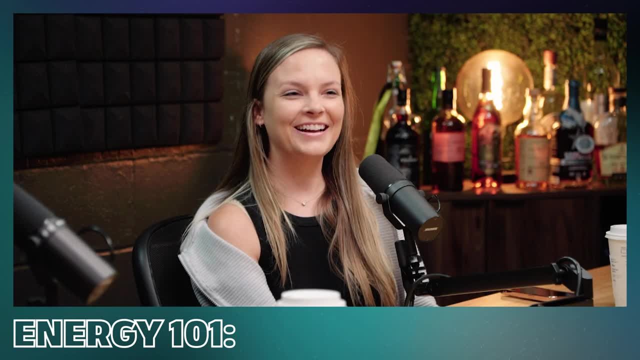 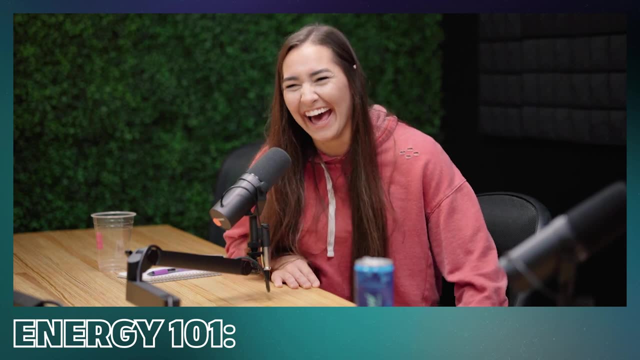 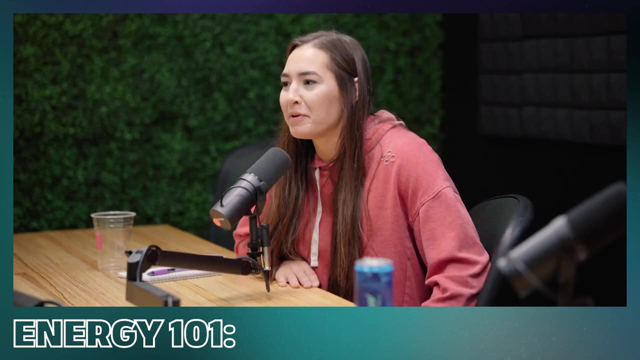 no questions. i explained that perfectly. i don't know if i did. the company i work for is probably like: do we should? you should probably, and we're questioning the. we probably don't even know if you said anything wrong, especially going all the way to china right now. we haven't dug to china yet, but if we do, 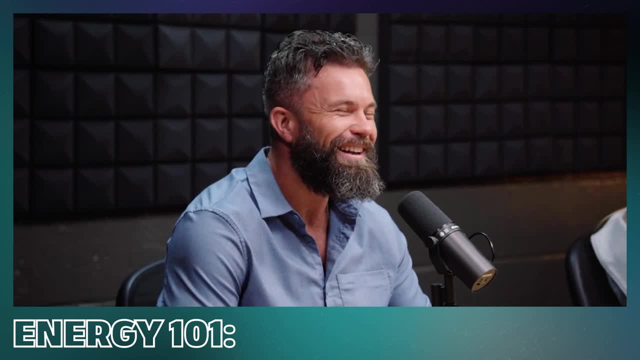 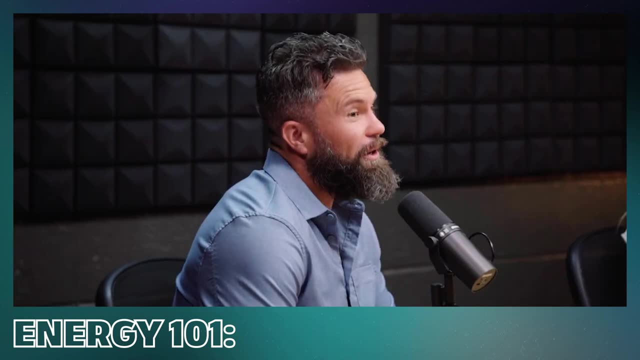 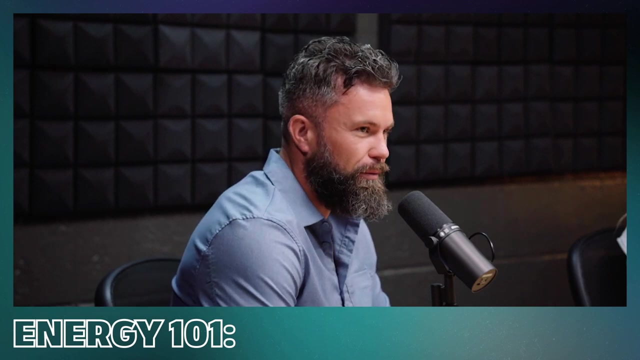 i'll be the one to provide the fluid for it. all right, here we go. okay, what is the number one misconception about the energy industry? the energy, or what is the number one misconception about the energy industry? oil and gas, or oil and gas? okay, um that we're all out to ruin the earth and make as much money as 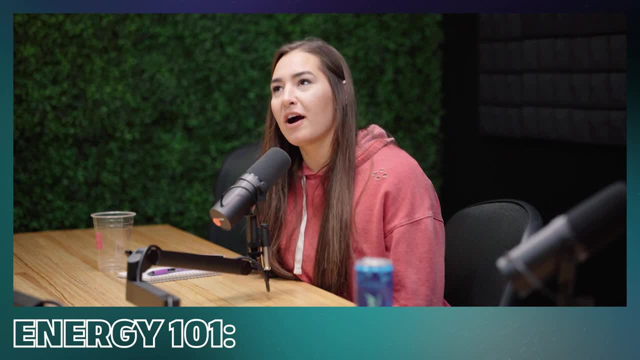 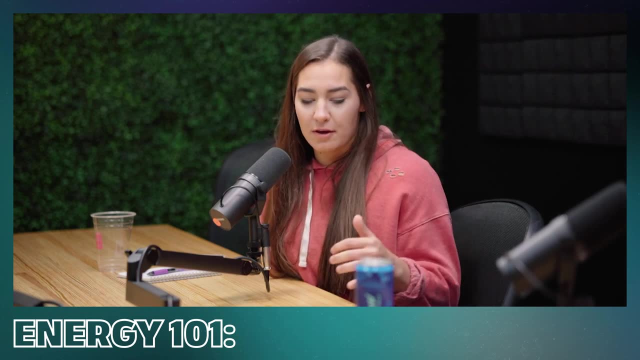 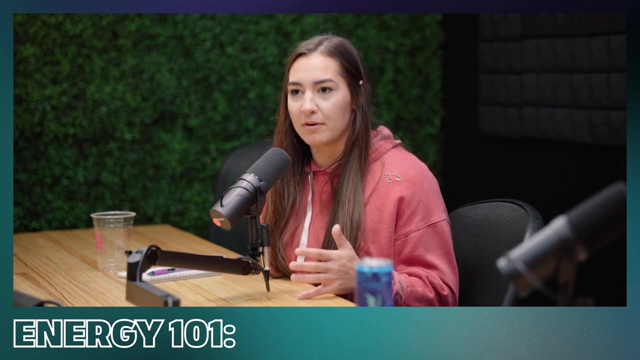 humanly possible. so would you say that, because i kind of believe this, that i think, um, people in the industry- it's like the environment is more top of mind than anyone else- like i think that we are doing a good job of trying to minimize, yeah, like our effect on, and i think that's. 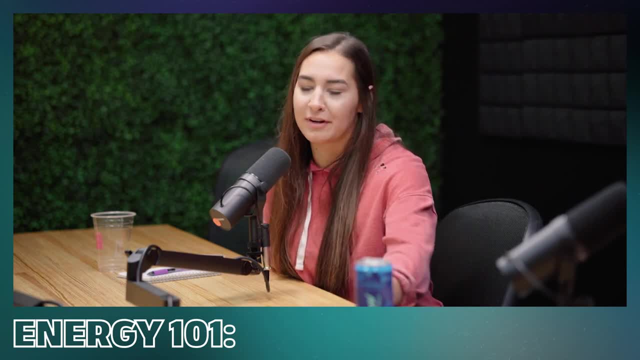 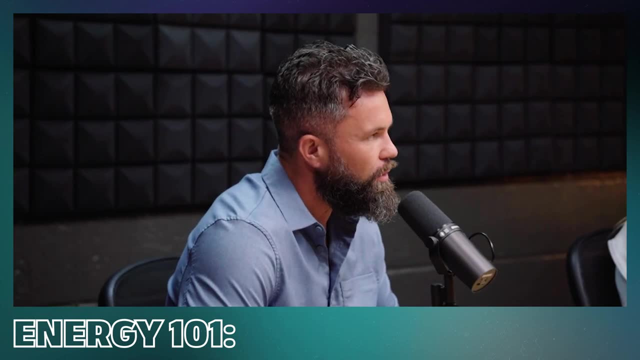 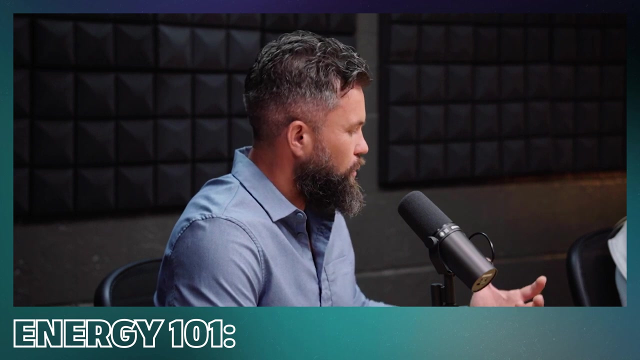 top of mind for oil and gas companies more than anyone else. would you say that? i would say that and and again. i, you know i'm somewhat biased because i don't have exposure to other industries who do operate in remote areas that ultimately, do you know, dig dirt and take forest away. 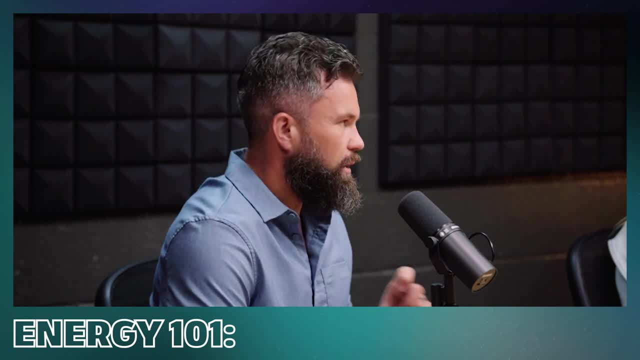 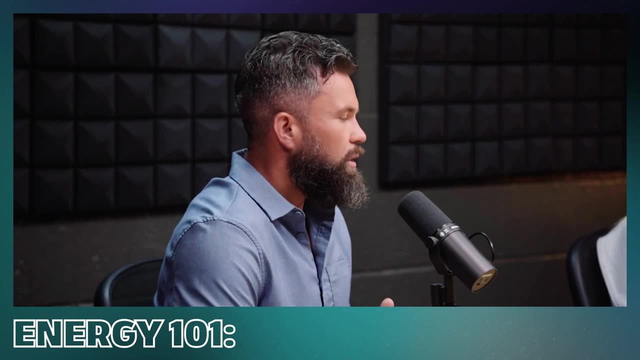 and everything else. however, if you look at land reclamation, especially up in canada, when, when an oil and gas company or an energy company goes and does their work you're not going to be able to, they are responsible for leaving that basically area or that land in better or in the same or 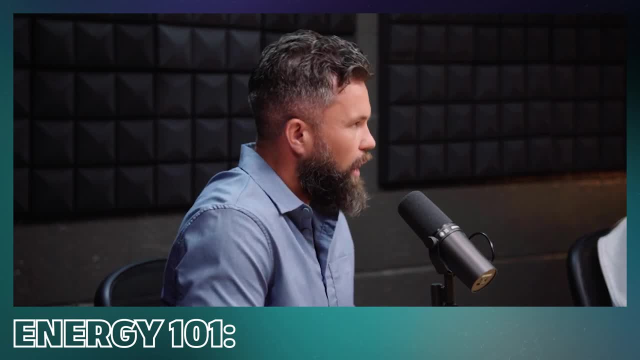 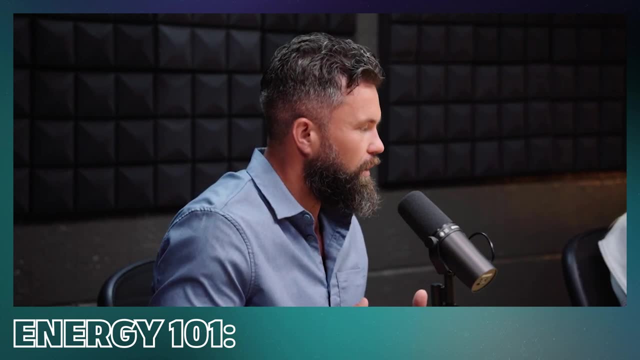 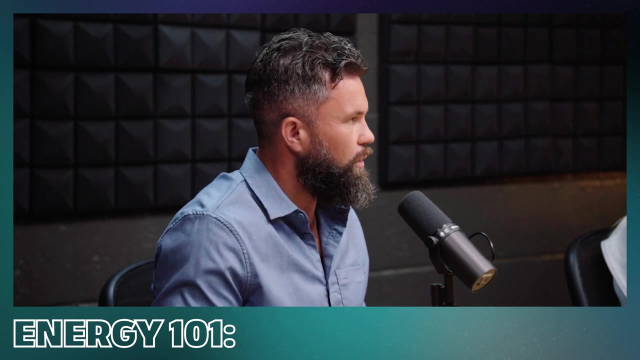 better condition than what they left there when they got there. yeah, so, yes, it is a lot of oil now, granted, it depends on the, on the company, right? like a lot of these huge companies, like they have a bullseye on their backs if anything happens, and they're the ones you know. you're not, you're not. 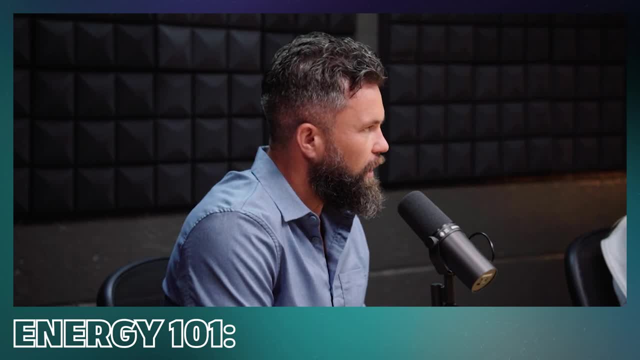 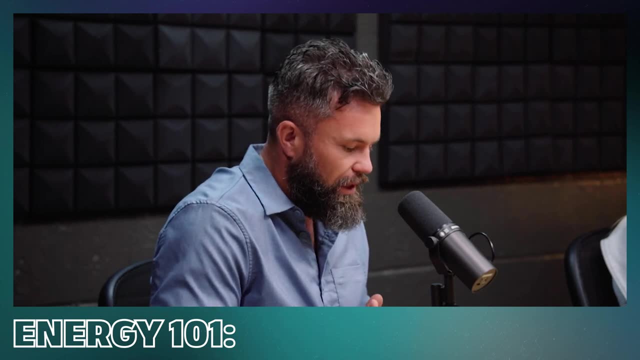 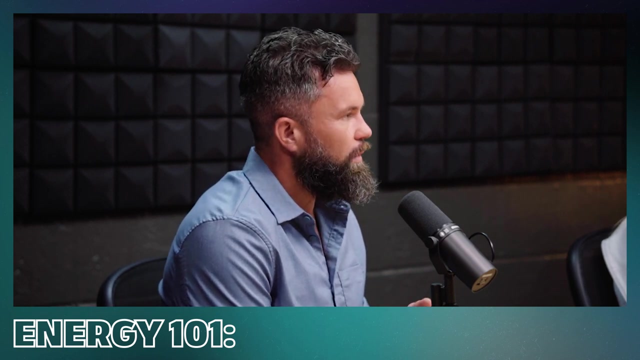 looking at all these small mom and pops that you know if all of a sudden they burn a rig down like you're going to hear about it, but if, like an exxon or a chevron does it like, then it's severe. but i can say this: through time- and i've been in oil and gas since 2004- is the emphasis on environmental. 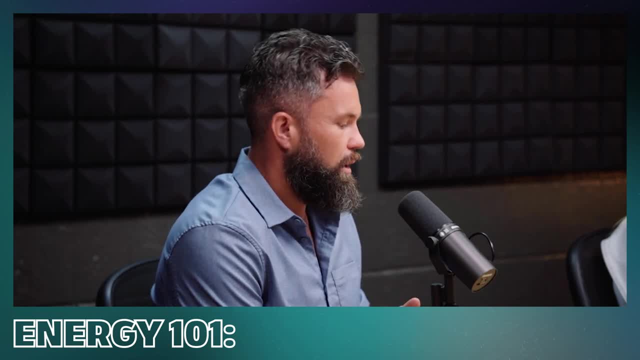 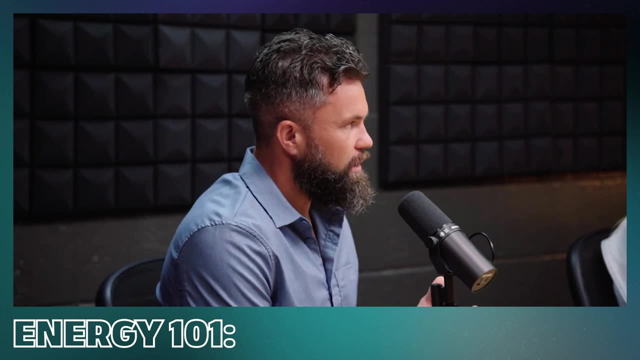 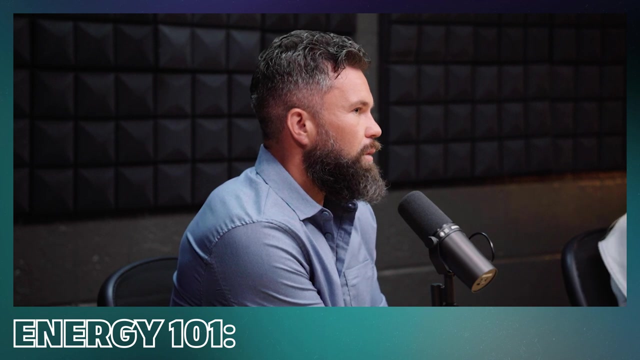 protection, land reclamation, making sure that they protect groundwater- there they have spent more money in r&d on making sure that they minimize the effects on the environment. then i would imagine a lot of other industries. um, you know, and one of the biggest things right now is is the methane, the. you know the flaring that's. 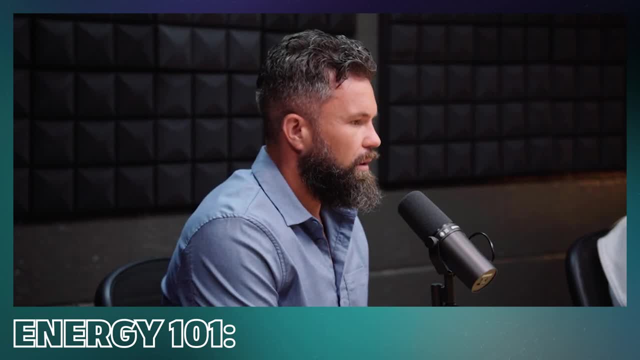 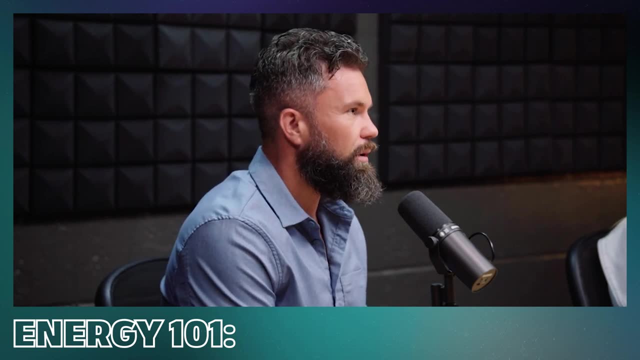 a huge topic of discussion and there's a lot of companies out there that are trying to come up with technologies to minimize that and find ways. well, now, with gas at almost ten dollars per- i mean btu that's- people are finding ways to try and get it to market, to sell it. but for a while gas was. 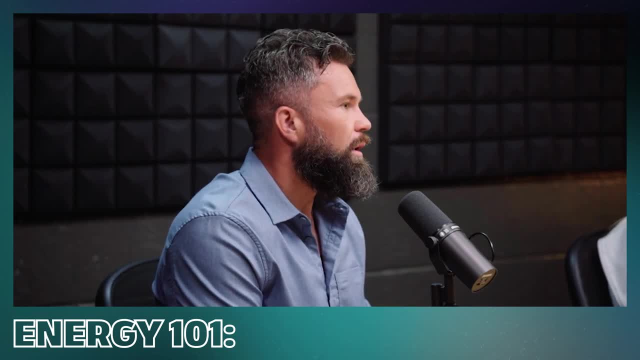 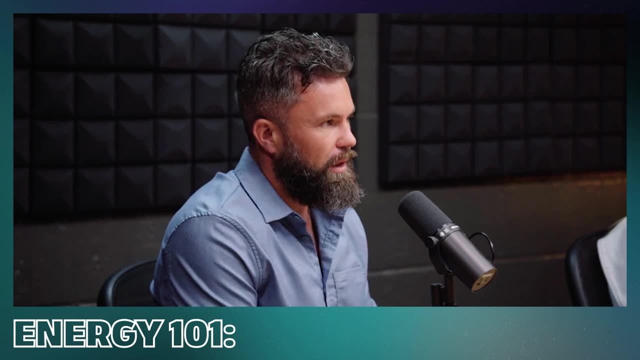 cheap and no one knew what to do with it, so they just let it, they just flared it and so but, but. but now there's a lot of you know policy and a lot of mandates in place to say, okay, we got to minimize flaring and a lot of companies are spending a lot. 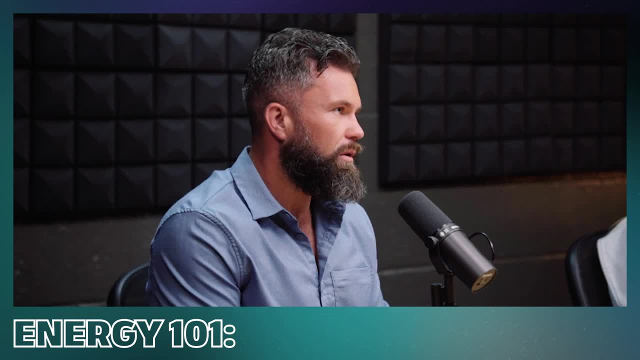 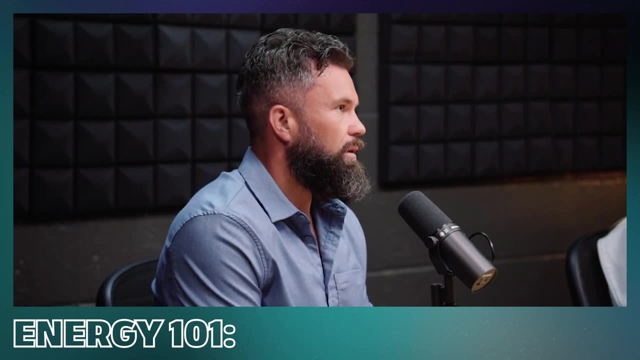 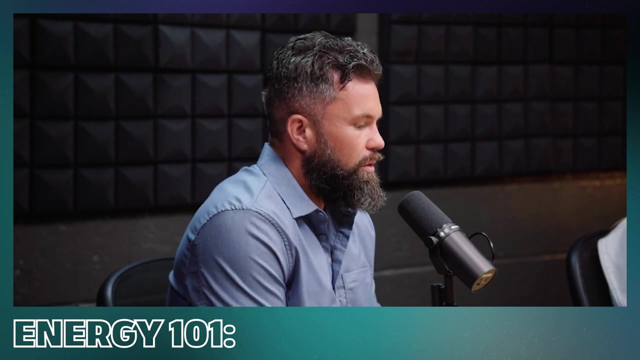 of money and time figuring out how to do that, and so yeah, there's. i mean, especially here in the us and in canada, like the, the environmental aspect of our industry is is extremely important, and a lot of companies like they spend a lot of time and effort trying to minimize that, and so, but you, 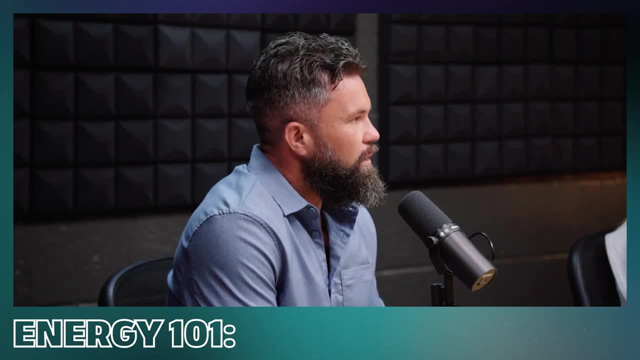 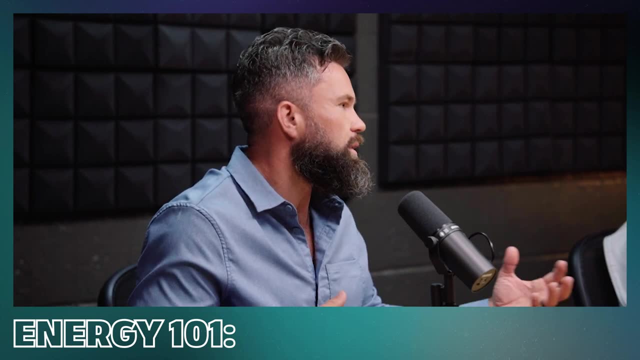 don't see that right, like it's a lot of companies that are trying to minimize that and so, but you're kind of behind closed doors and they do it and you know people can plug their iPhones into the wall and it doesn't really mean anything, it's. you know what I mean. so it's again to your point. is: 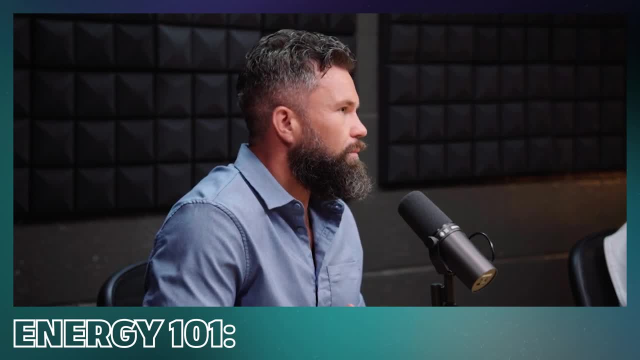 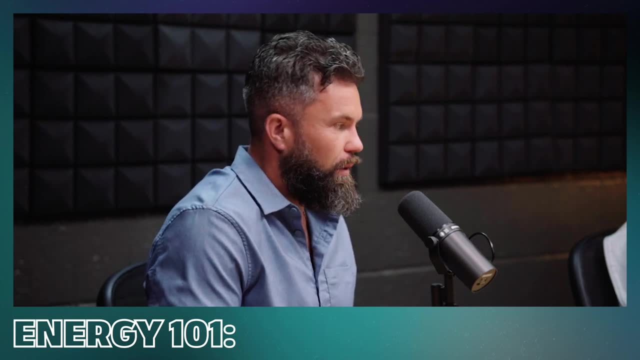 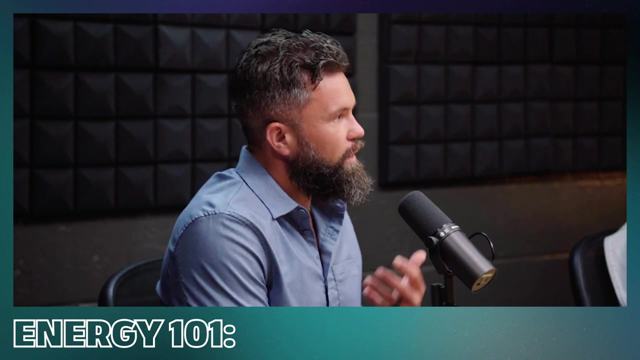 it's like you can't see them when they're doing that. yeah, um, but it all adds up, at the end of the day, to where the US is producing in a way that's much safer and environmentally friendly than a lot of other parts of the world. um, and I've seen it and I've experienced it, and I've 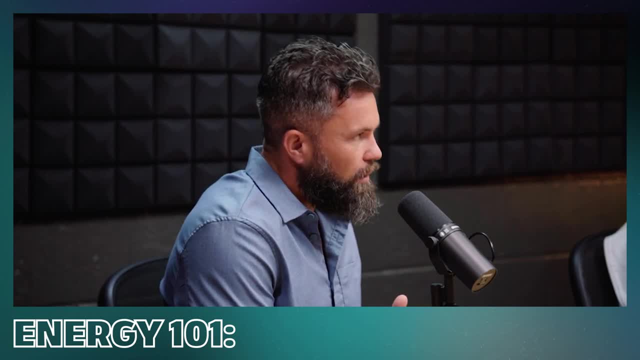 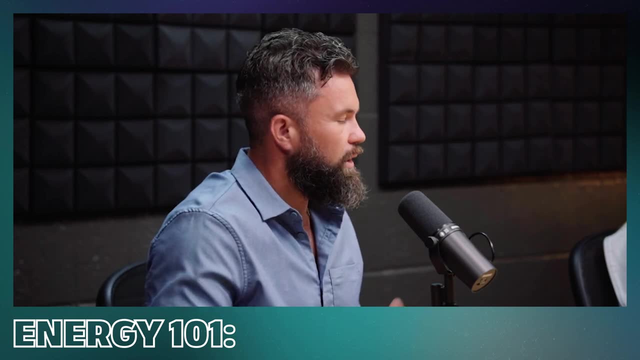 been in meetings and talking about, like you know, reducing the amount of water they use. they're reducing the amount of people that are on the road driving. um, those are just like a few of like tons of other things, but there's these little things that make people can grasp is like oh. 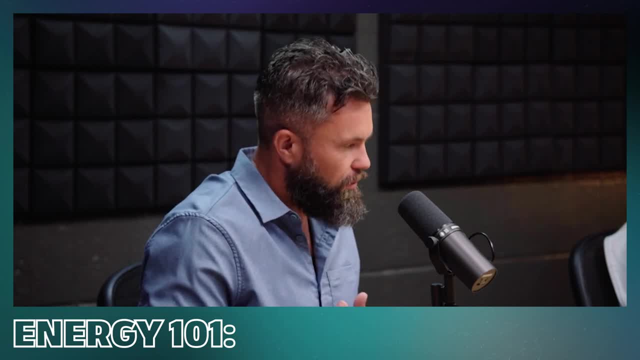 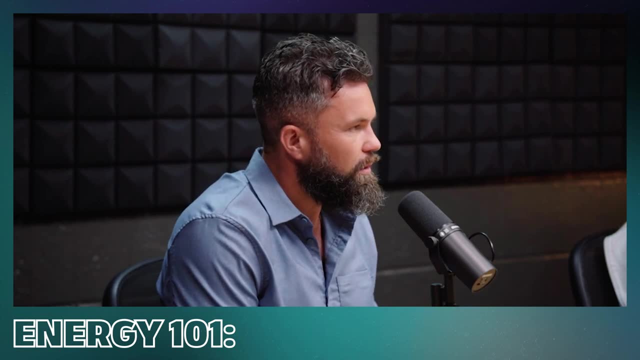 they're, you know, because when you frack a well, it uses a ton of water. well, they're everyone's trying to reduce the amount of water we use because you know it's somewhat finite. so, um, but yes, oil and gas companies. I mean, it's crazy. 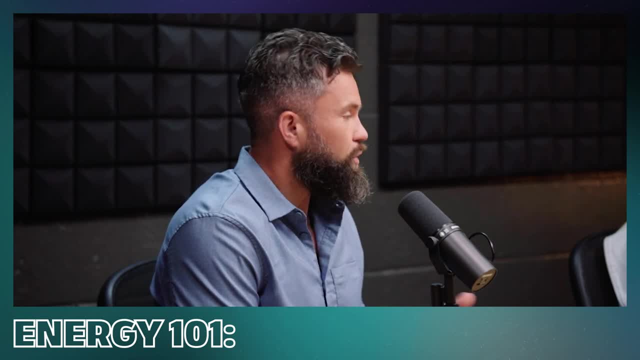 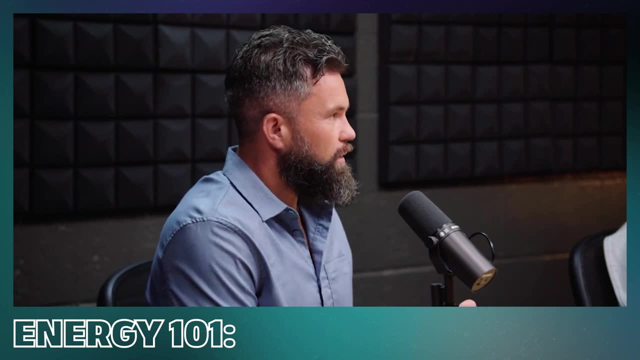 to see how much money and time they put into that, because you know investors want it right now. if you're an investor, you want to invest in companies that have the- you know the environment, um, like they have the. if you're in, if you're on the investment side, most companies want to invest. 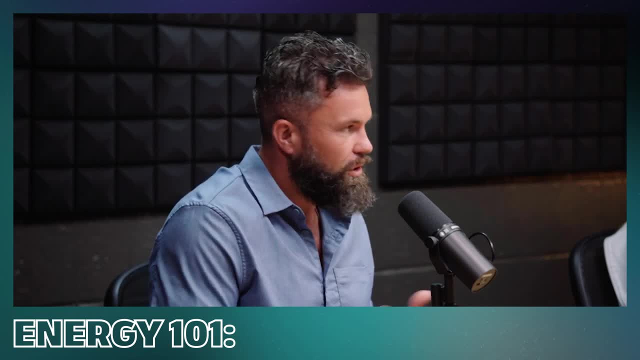 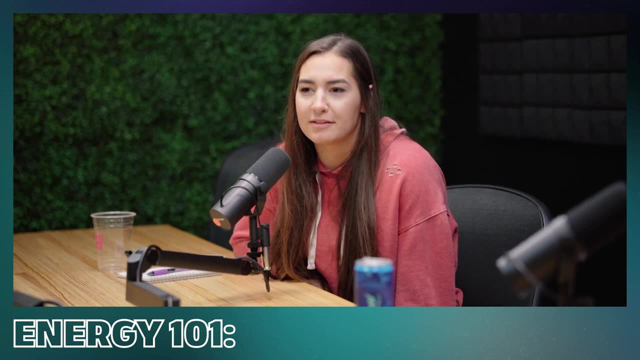 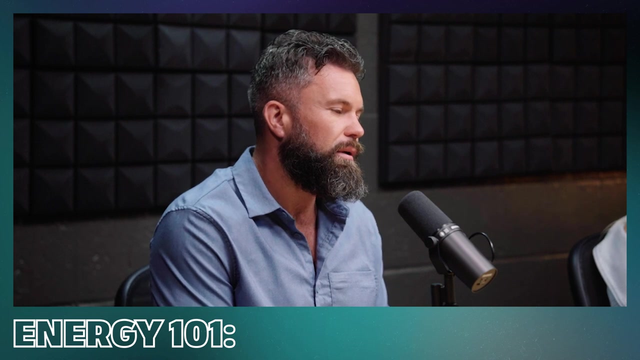 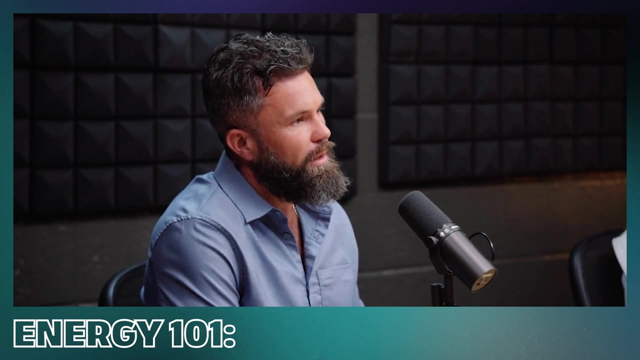 in companies that have, uh, like good ESG metrics, environmental, like friendly, and, yeah, they also think it increases efficiency in some aspects. yeah, um it, it does. um again, I can't, I wouldn't. I don't have enough experience on the operator side to say if they operate more sustainably and they have a better ESG, sort of certain ESG standards or 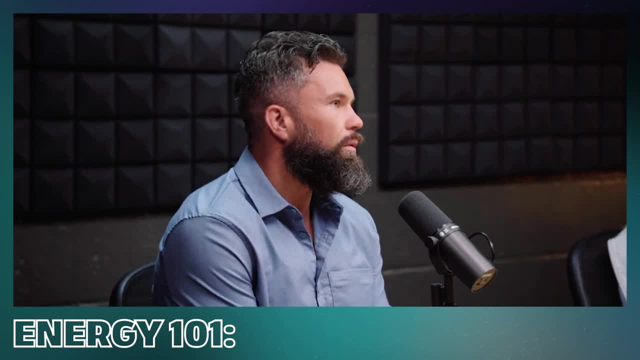 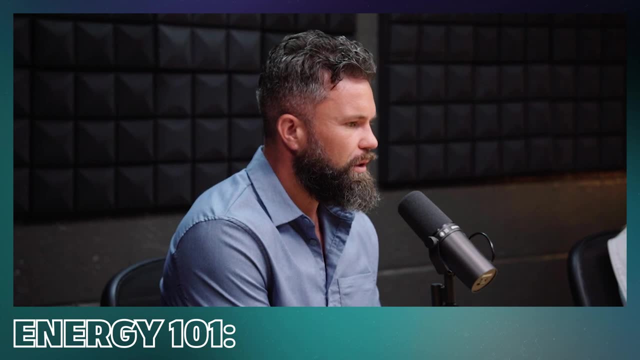 environmental standards that they operate more efficiently. I I don't know that per se. um, I wouldn't want to come out here and say, yeah, if, if companies have a good environmental standards, they're going to operate more efficiently, but it's more efficient for the entire ecosystem to. 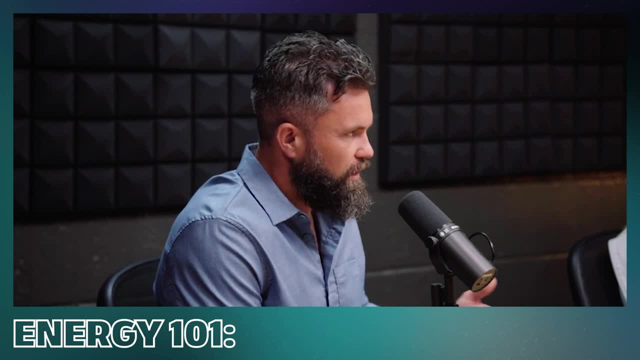 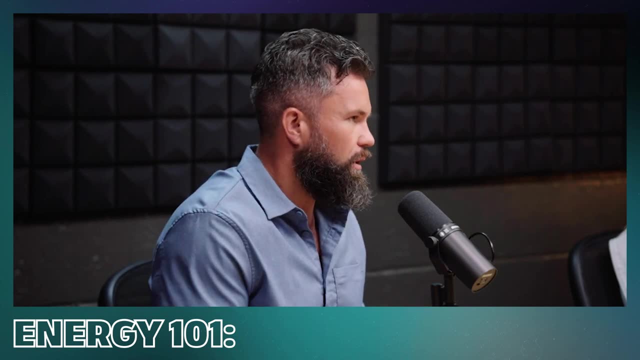 operate more efficiently, because they're going to have a better ESG and they're going to have a because, ultimately then, investors are going to want to invest in companies that do operate in a good manner. um, to where then? yeah, it's. if we can produce more here in the US, then that obviously. 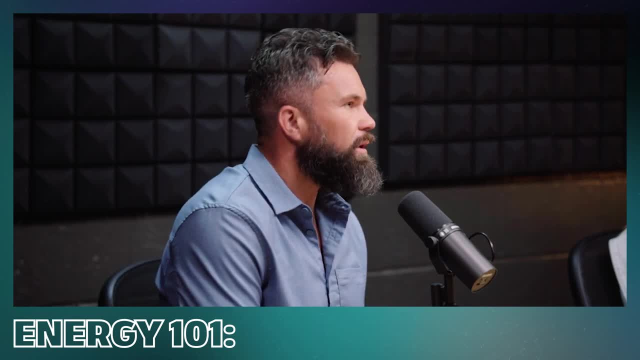 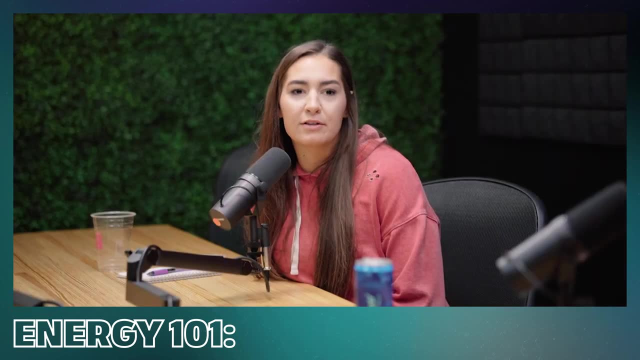 that that would be much better. so anyway that, yeah it's. it'd be hard to make that parallel. I didn't mean to uh, hijack your rapid fire, but I do want to plug in. so we are doing a vlog series with Presidio Petroleum and they we just this week released an episode- um, and it's all about. 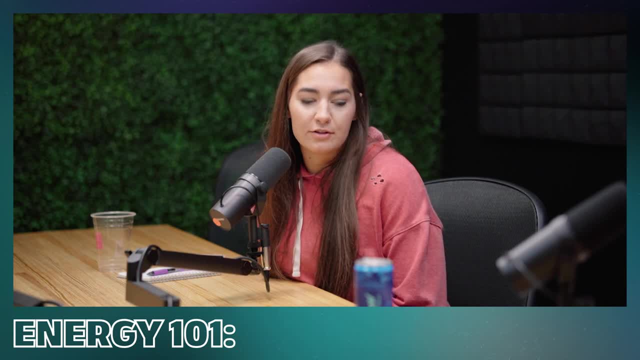 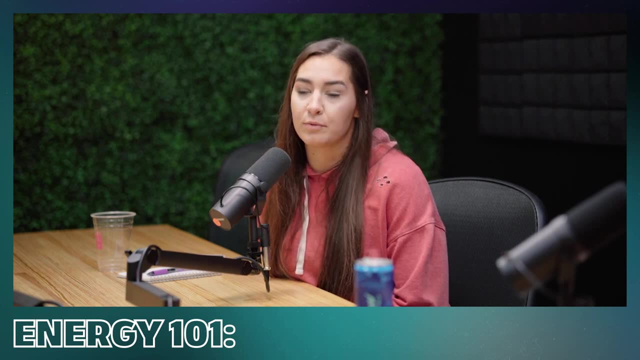 lowering emissions, um, and their operations. so I found it very, very interesting, and I think that other people would too. it's just their take on it as an oil and gas company is very interesting. that's kind of why I had kind of some conclusions. but yeah, it could be just them, but I hope, like 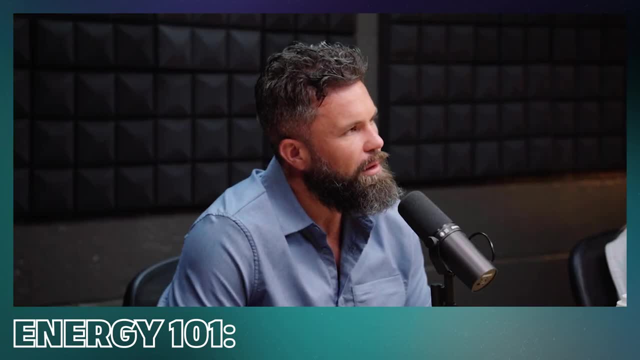 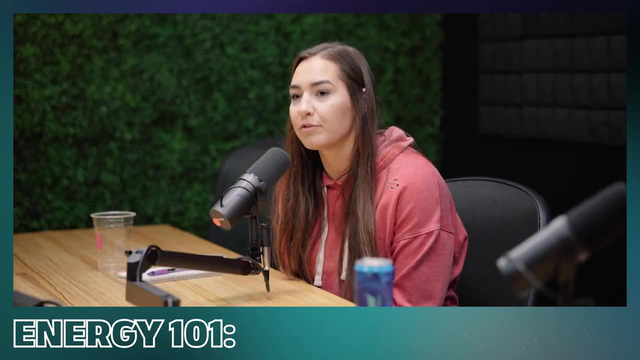 they're the future and others will follow. yeah, yeah, no, I, I mean that would be something I need to do more research on, on that as well. but and what was the operator's name? Presidio, Presidio, Petroleum, nice, no, good for them. that's awesome. yeah, all right. yeah, um, we kind of touched. 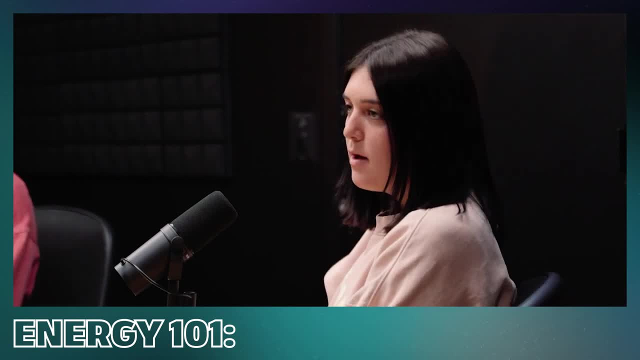 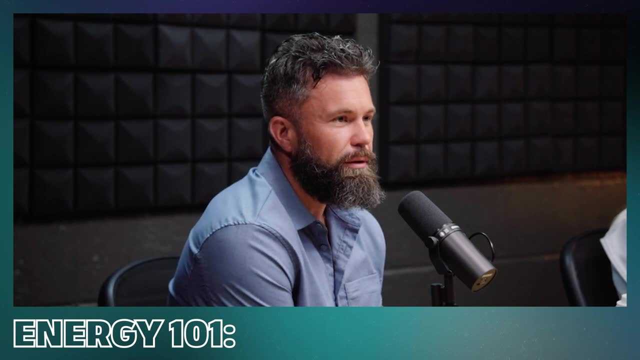 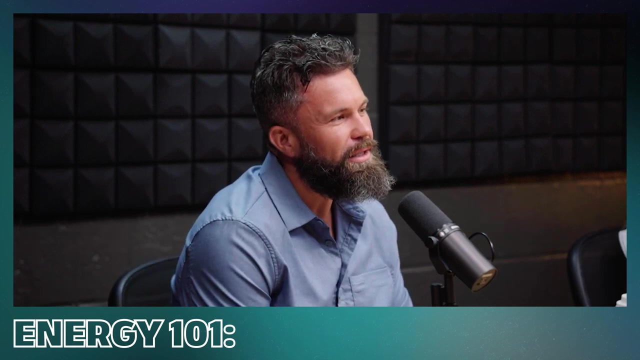 based on this one. but why should I like someone that doesn't know anything about the oil and gas industry or the energy industry? why should I care? um, you shouldn't? no, I'm just kidding. yeah, don't worry about it. um, I just make our lives easier. yeah, it'll be there, just keep paying. 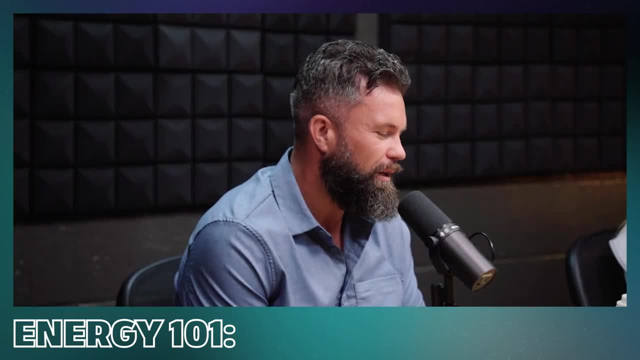 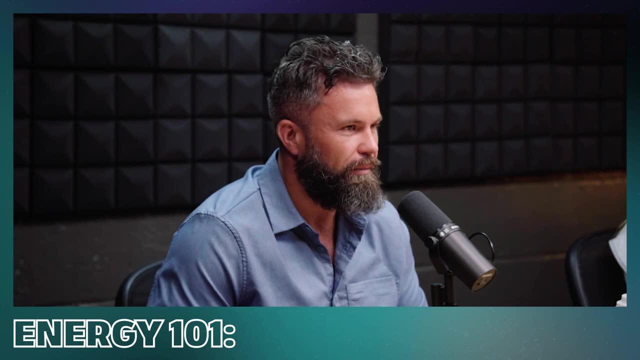 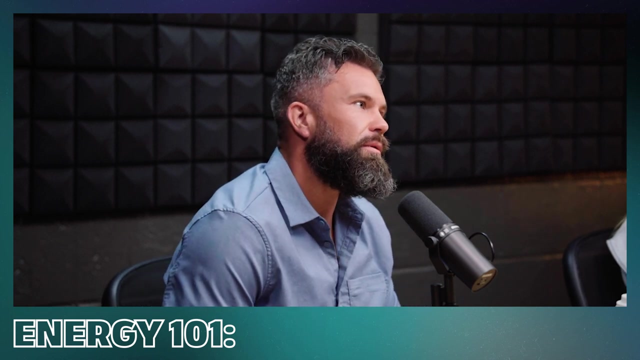 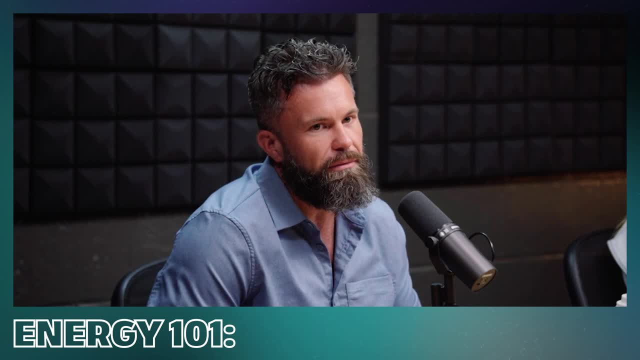 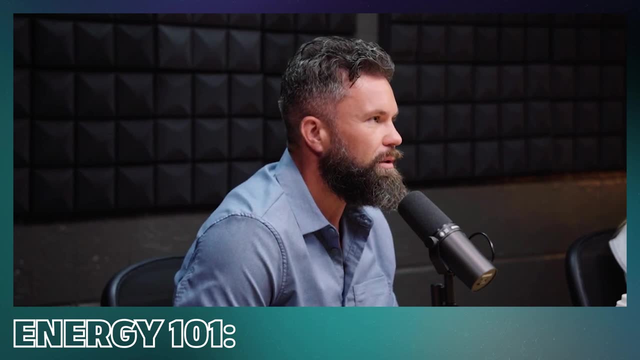 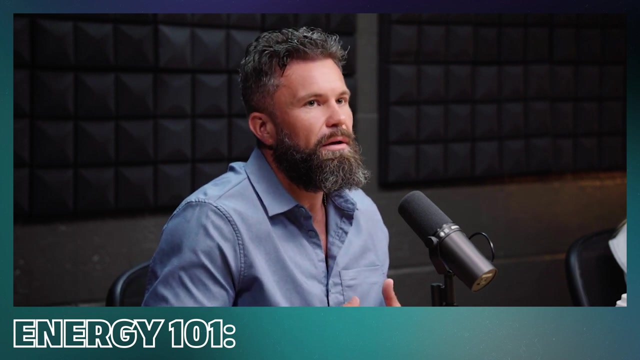 people can be educated. they can make sort of educated decisions. right, knowledge is power. yeah, that's exactly, and so I think it just comes down to having a better understanding and and it helps guide your decision making, um, whether that's conserving, like so, for someone like yourself and- and I- and I know this because 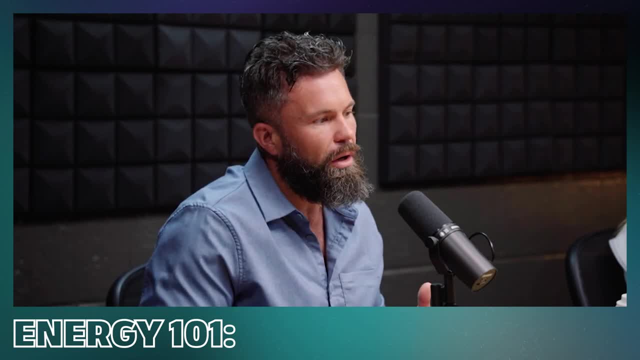 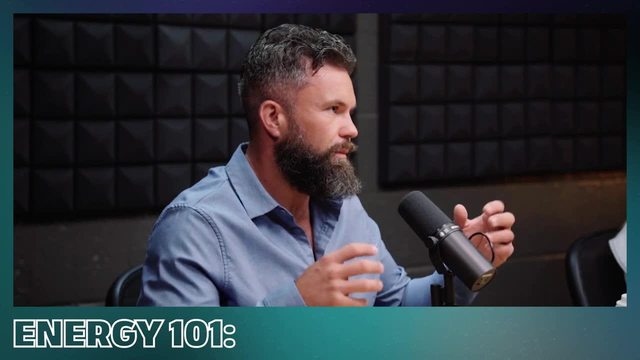 I've spoken to people that you're in their 20s. they make a lot of their buying decisions based off of company values. so you know, whether you're you're going to the store and if you see a you know a shirt that like, oh we, you know, we, you know a portion of our proceeds goes to whatever. 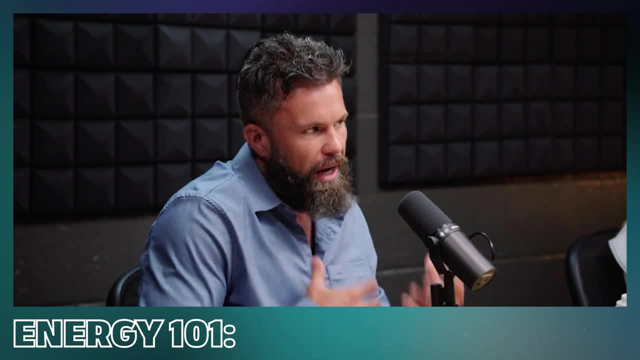 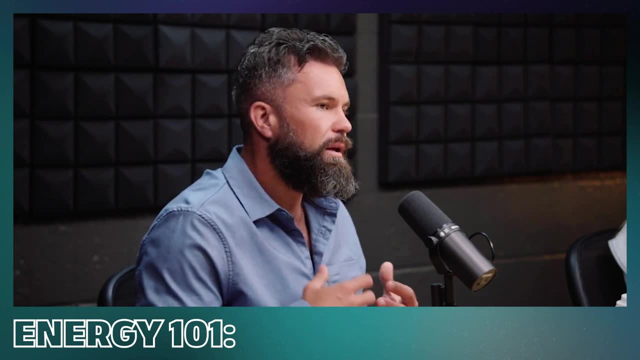 environmental company versus no one. like the behavior of consumers right now is like I want to buy stuff that I align with the industry. I want to buy stuff that I align with the. this company values. so yeah, and so if you have an understanding of like energy and oil and gas, 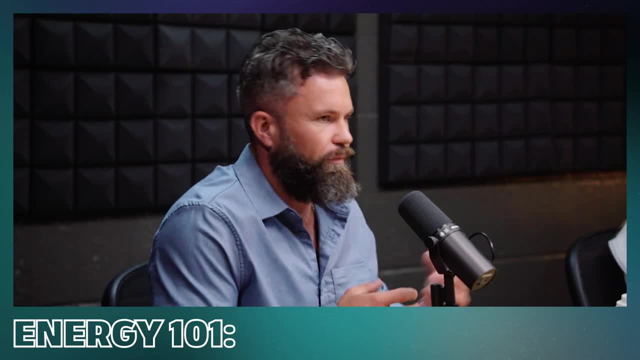 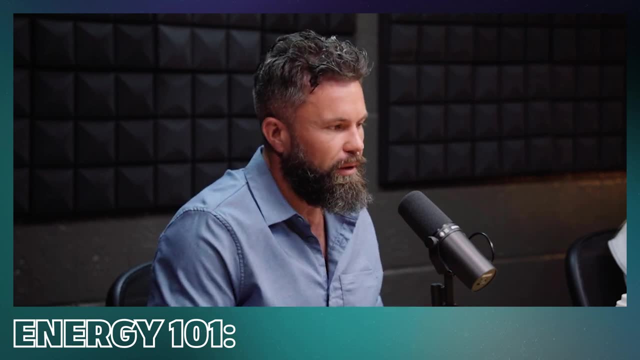 it might help you make better buying decisions, not like t-shirts, but, yeah, um, it helps you understand why your, why your electricity bill is probably going to be double. um, I don't know if you pay your electricity bill, but I lived in New York and, uh, I, yeah, I got a big understanding. 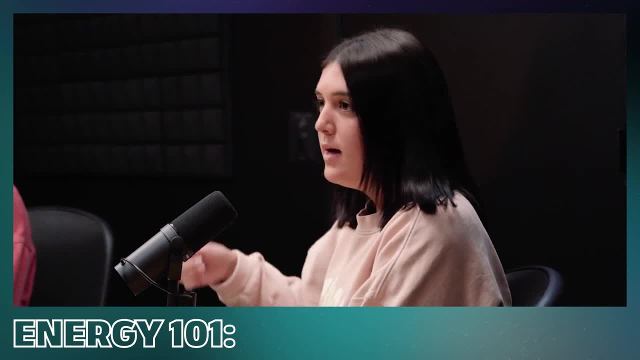 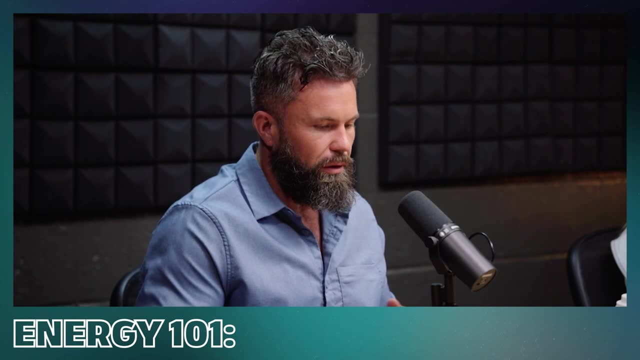 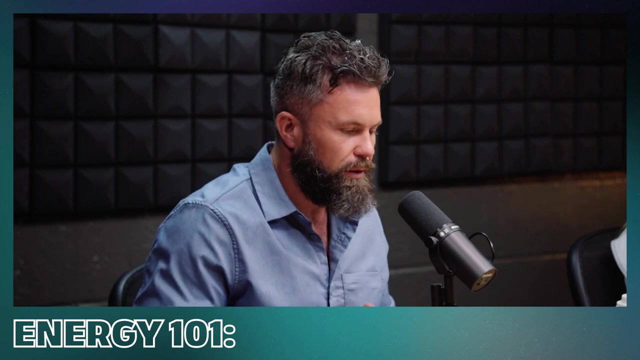 every month when I my con ed bill is coming in, I'm like, okay, why in the summer price is getting higher, you know, yeah, so here on a macro level, it allows you okay. so, ultimately, whoever our administration is, whether it's, you know, blue, green, red, purple, whatever, um, well, there's only two here in the US, but uh, so it allows you to. 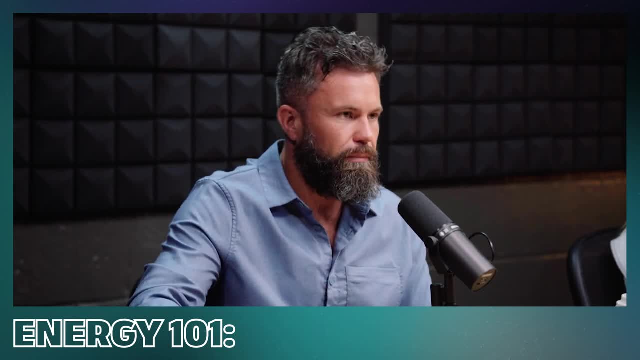 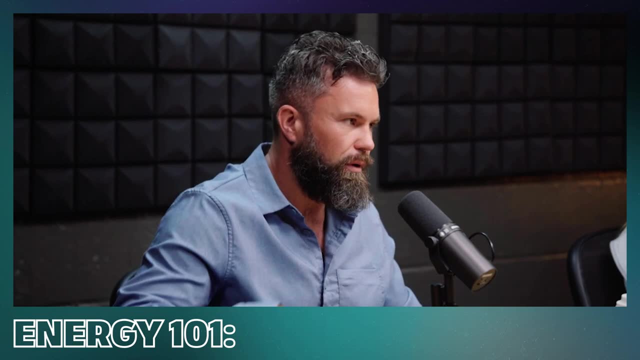 make better decisions when you're voting for, and it allows you to understand policy, and I think that's where, ultimately, if you have an understanding of energy, a lot of when people, when the president voting, comes up, a lot of their initiatives are energy policy and energy security, and so if you 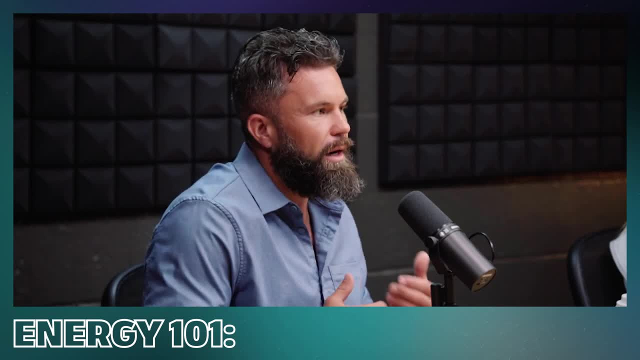 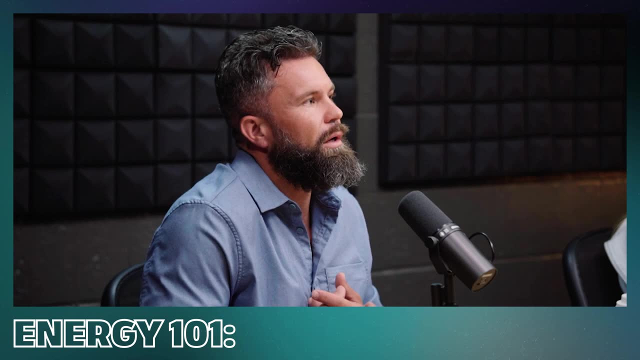 at least have some kind of understanding of energy, you're going to be able to make better decisions, some basic understanding of that. then it might help you justify why you're voting for somebody. um, not to make it political, but ultimately, if you vote for someone who, let's just say, is like we want, 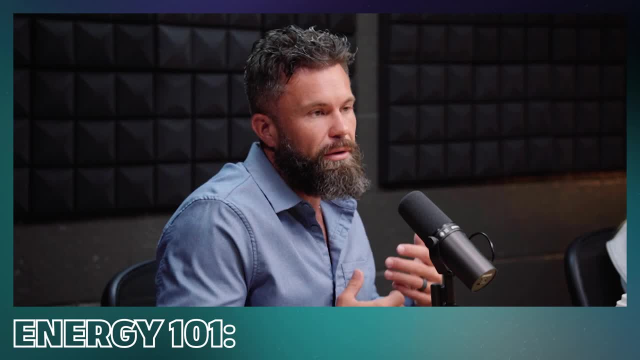 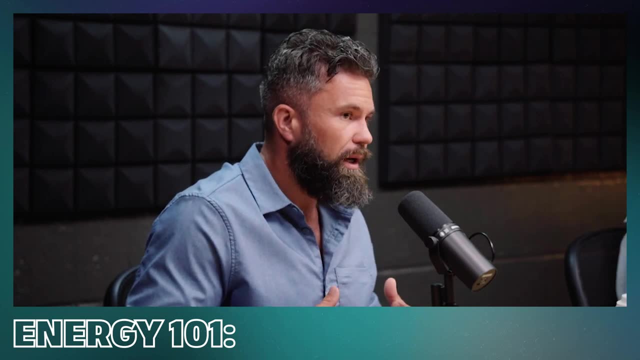 to stop oil and gas production period. well, at least then understand that your electricity and all your energy prices are going to go up. on top of that, we're still going to use that oil and gas. so if we can't produce it, where are we going to get it from? oh, we're going to depend on people. 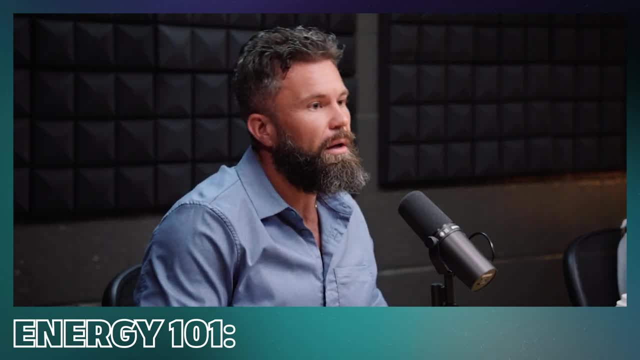 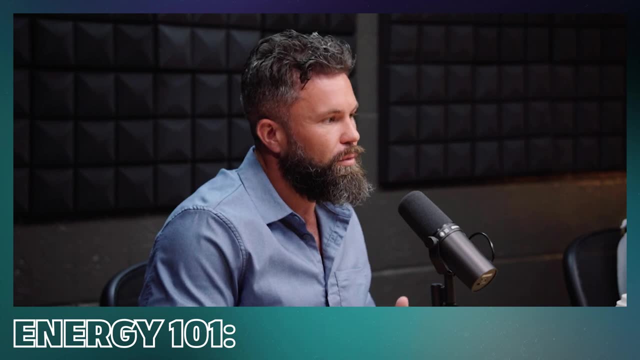 from overseas and if we do that, then we're giving up our energy security, and I'm not going to go into energy security, but that's a good sort of topic to google is: what is energy security? and so that was one thing in our former administration- was like energy independence. 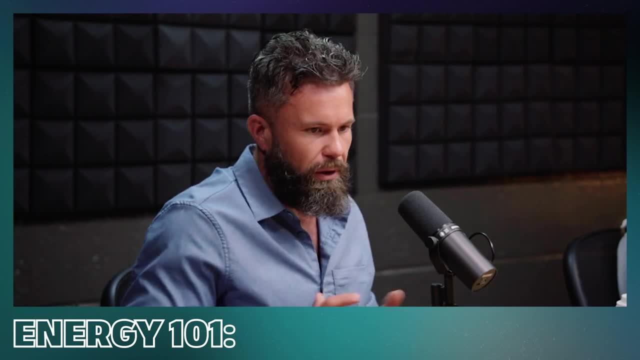 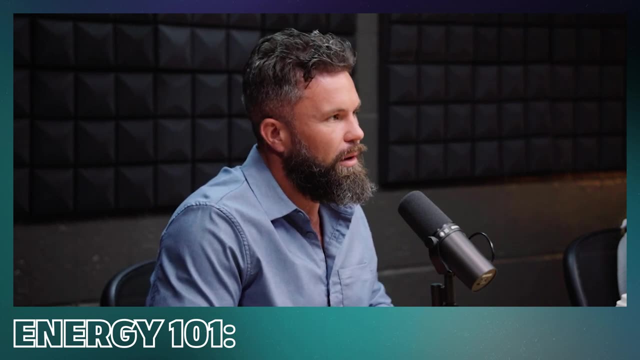 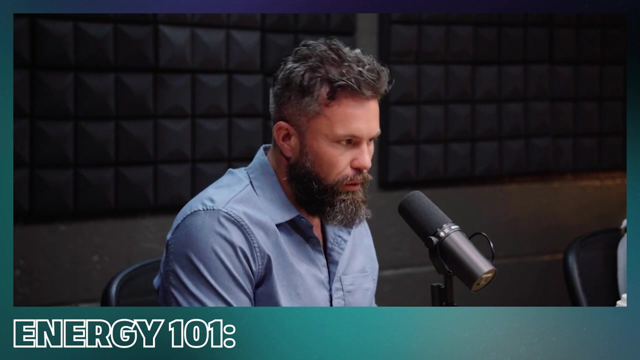 um, you know again, no one's perfect. I'm not blue, I'm not red, I'm more purple than anything. however, there there is something to be said about having a degree of energy independence, because that also increases our energy security, and wars have been happening for years over money and power. 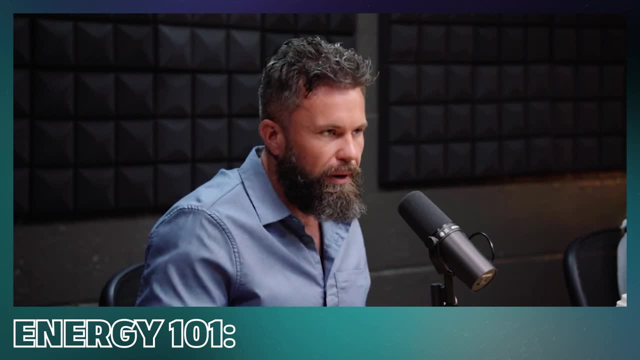 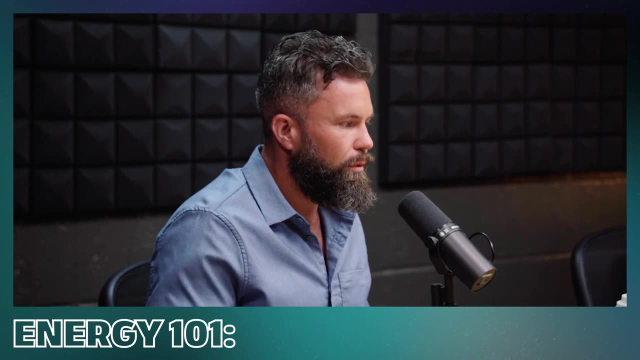 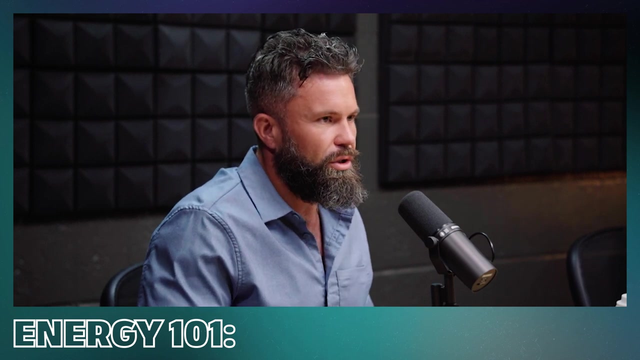 and oil, and so it all ties together and it impacts us, whether we want to admit it or not. um, it's again, it's again. like you said, the more knowledgeable you are, the more you have an understanding of how it all ties together. you can ultimately make better decisions, and more educated decisions, than just off like. 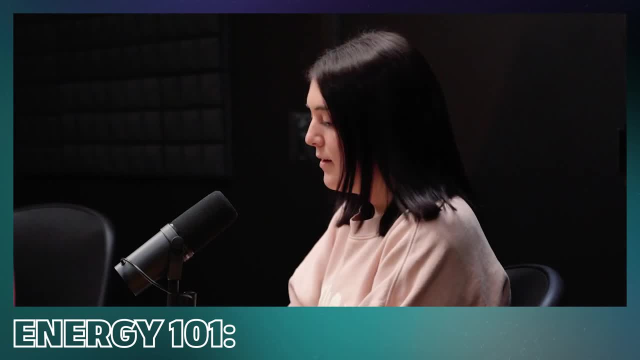 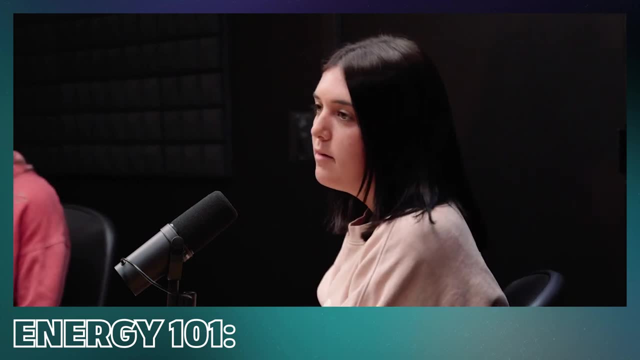 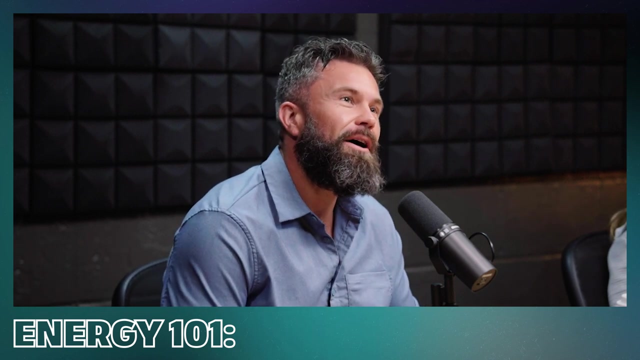 emotion or headlines that we see every day. yeah, yeah, that's a really good answer. um, our last one, that's my favorite one. what is your most embarrassing story in your career? my most embarrassing story in my career, oh, that's a good one. let's see: oh, this is a good one, uh, and then after this, I do have to bounce. 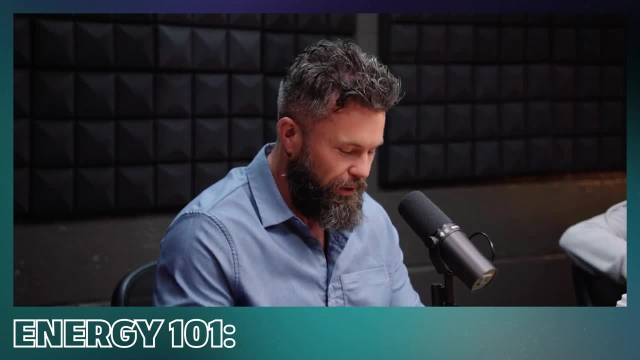 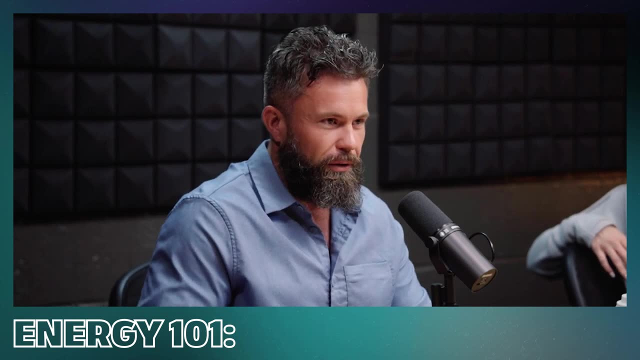 ladies. but so I started. so I was when I graduated high school. I didn't know what I wanted to do, so I started working drilling rigs. so then I went from being a city boy who enjoyed, you know, the finer things of life- partying, ladies, all that stuff- as an 18 year old. well, I went from that to going to 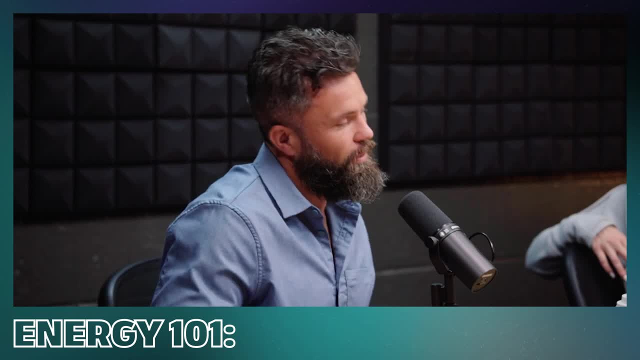 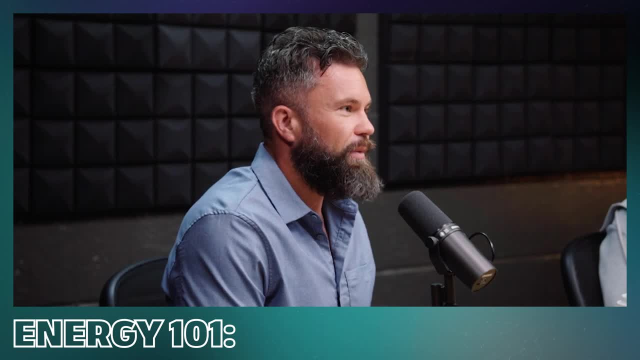 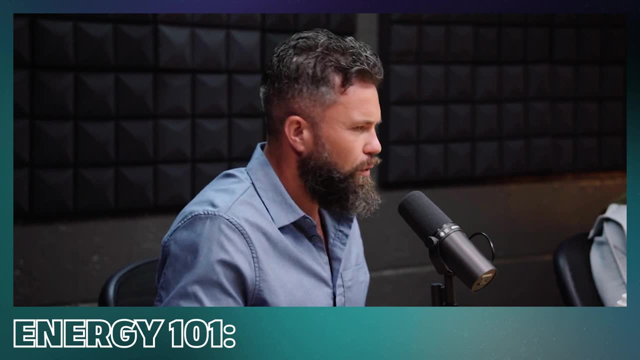 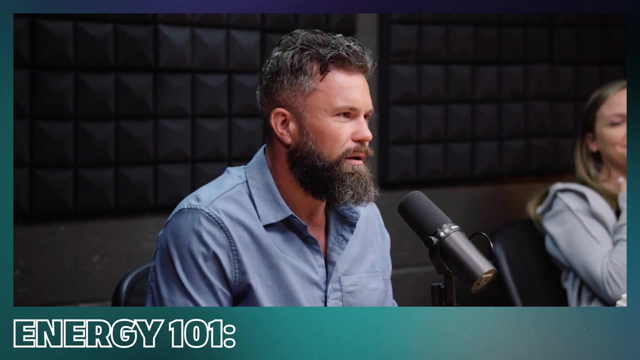 crews. that means that you don't really get days off, um. and so when that was happening, so I got onto the rig and I was like, so yeah, this this two week on, two week off thing, and they're like: nobody like you're out here until we tell you you can go home. and I was like but I thought, oh, okay. 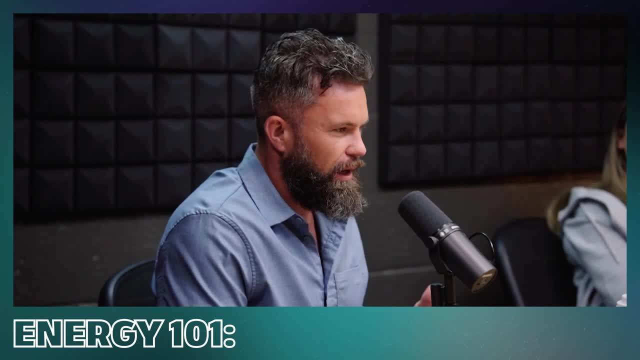 never mind. so anyway, um, we're gonna rig. and it had been like three weeks and I was like I really want to go home, like, oh my god, I'm gonna go home, and I was like I'm gonna go home. and I was like I'm gonna. 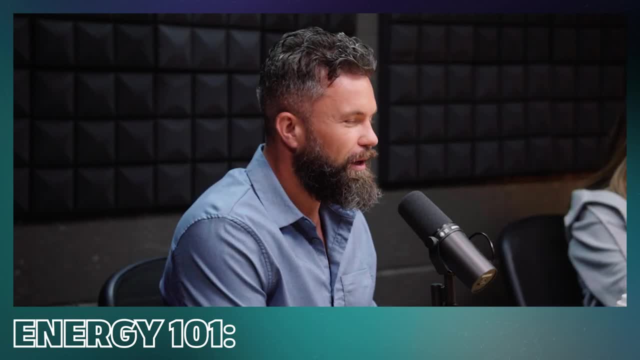 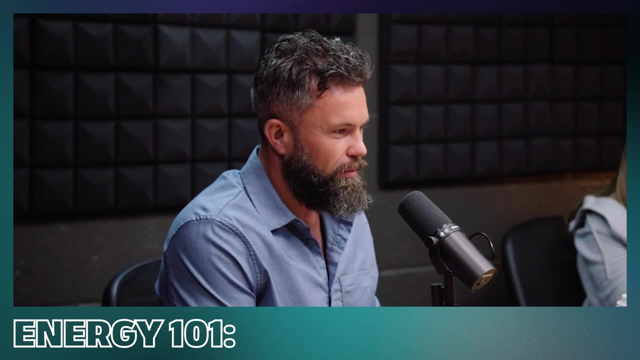 I went from being at home like comfort of my parents' house to now working on a drilling rig And I don't know when I'm going home. This sucks. I hated it And I was a lease hand and part of my job on a day-to-day basis was cleaning the like the rigs, toilets and like the bathrooms And in. 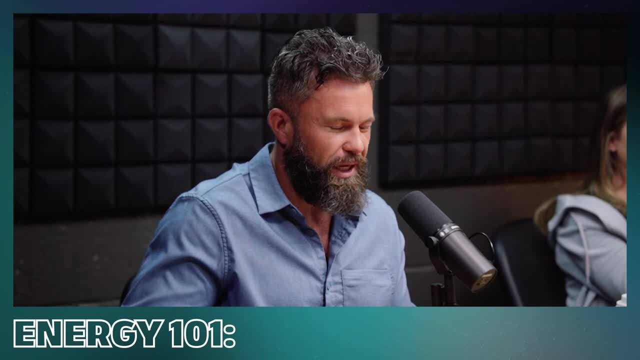 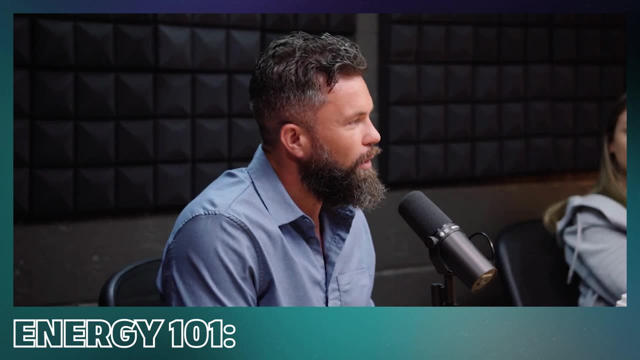 Canada: the trailer, the tool pushers trailer and the tool pushers kind of like the boss on the rig. Well, anyway, at the end of his trailer was the bathroom. So one day I was cleaning the bathroom and I was trying to figure out like how I could get home, Um, and I was like, well, wait, you know. 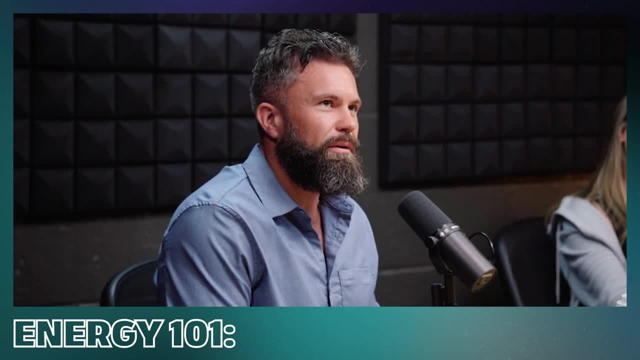 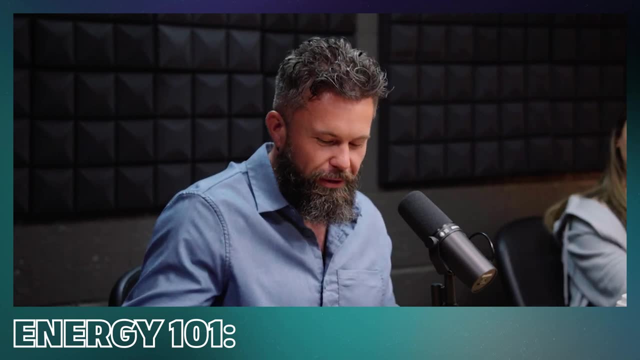 like I have, you know, a wedding coming up and I was like, okay, So, but I was too embarrassed to go into the to the my boss's trailer through the front door. but from the bathroom to the door, um, or from, like, the bathroom that I was cleaning, there was a door to his office. 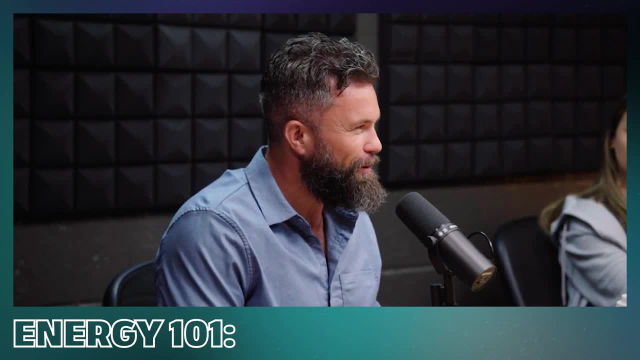 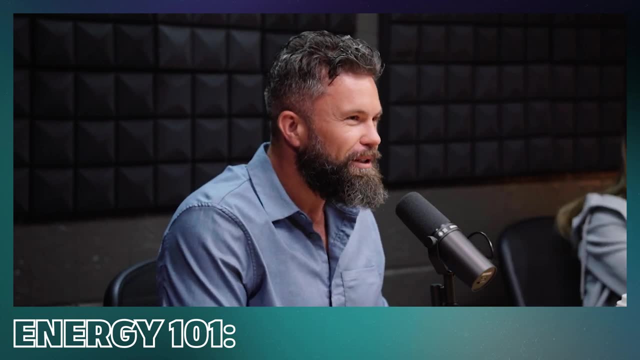 and I heard him in there on the phone, And so I waited in the bathroom until he was done on the phone. Then I knocked on the door and his name was Daryl And he was like hello. I was like Hey, Daryl, this is Justin. I'm cleaning the bathroom right now. I was wondering if you had 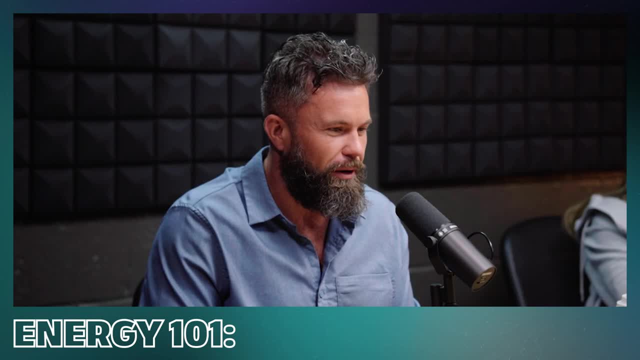 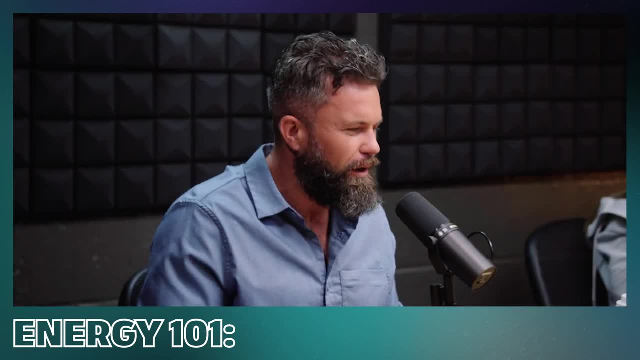 know, And so he opened the door and he's like: you're the first person that's ever done. He's like: what do you want? Like well, uh, I haven't been home in my. I have a wedding coming up and 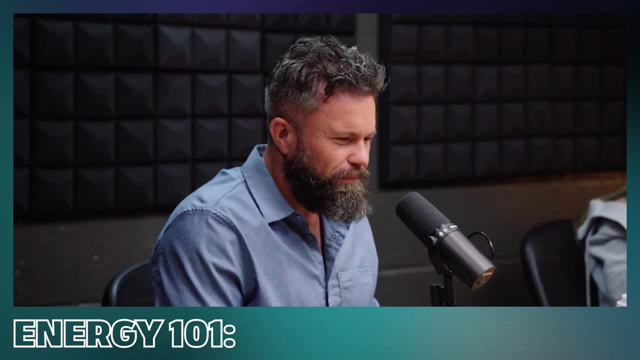 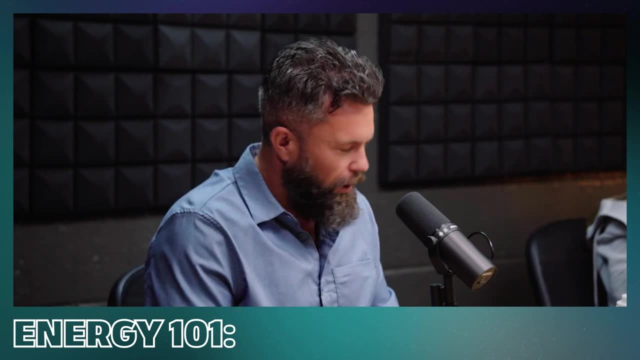 I was wondering if I could be home. uh, for you know, I gave him a date and, uh, he didn't give me an answer. but that was like looking back, if, if I was like a boss and some kid like was. 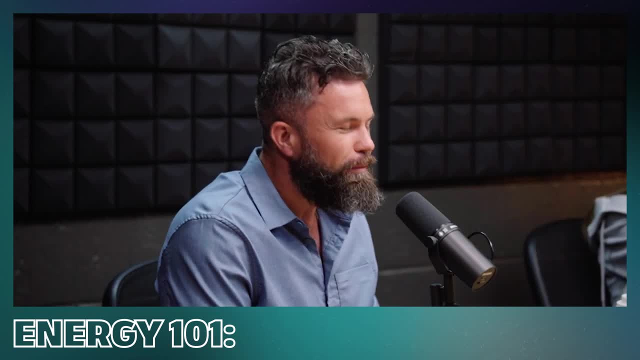 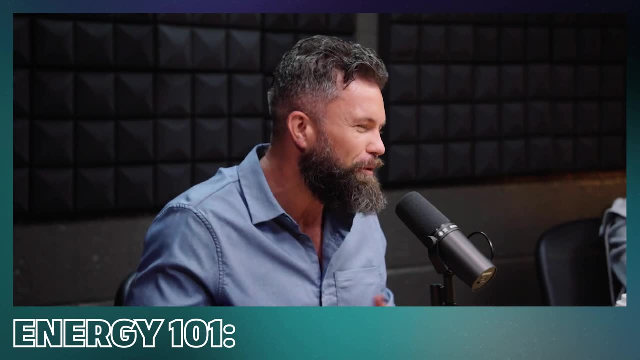 cleaning the bathroom and knocked on the door to ask for days off, I would have probably ran him off. I've been like: don't ever ask me for days off while you're cleaning the bathroom. That's just so awkward, And so it's. it's not really that embarrassing, but it's like in looking back at. 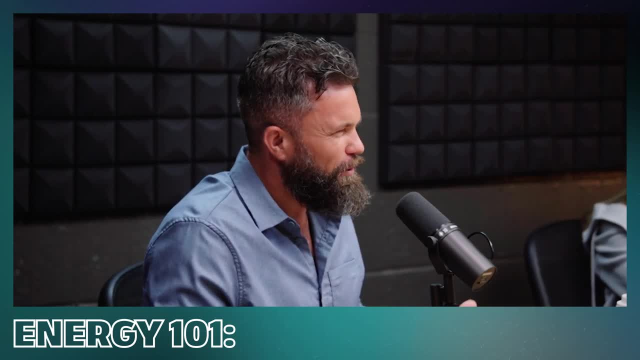 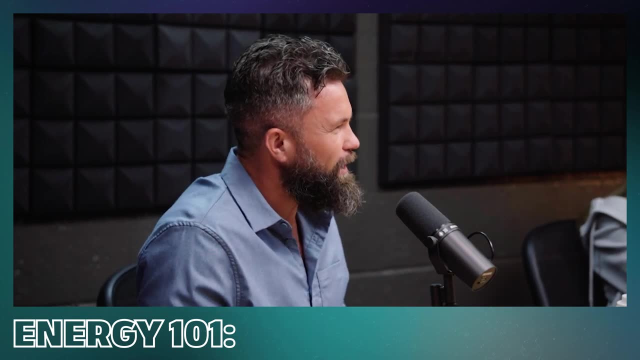 it like I was. I didn't know how to approach my boss And so, yeah, I was sitting there with like a scrub brush and like like gloves and stuff, like cleaning the bathroom, asking for time off, like looking back, like I wasn't embarrassed at the time. but now I'm like, wow, that was. 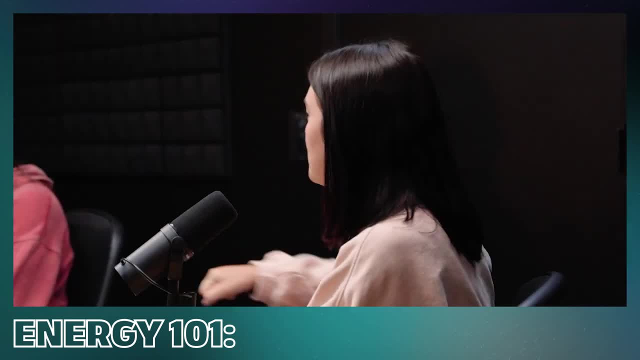 extremely embarrassing. I don't know why I thought of that. I'm sure there's scrubbing the toilet, Hey boss. by the way, can I uh go home tomorrow? Yeah, Like, can I? yeah, can I. 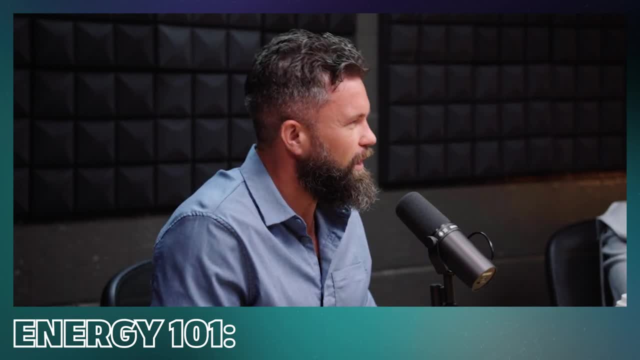 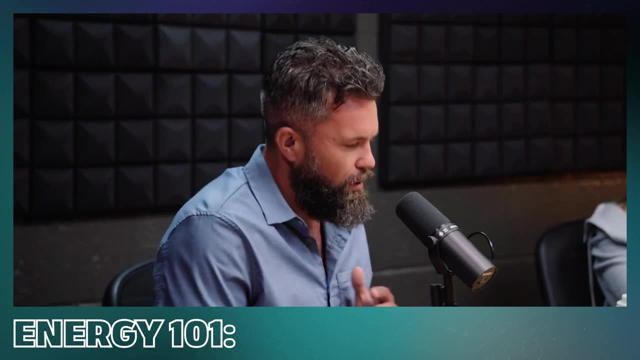 can I have some days off? And the crappy thing is like he never gave me an answer for like two weeks, So he kept like dragging it along and I was like God dang. And then he finally was like okay, He's like look, yes, you can, you can go home for these dates, but then you got to come. 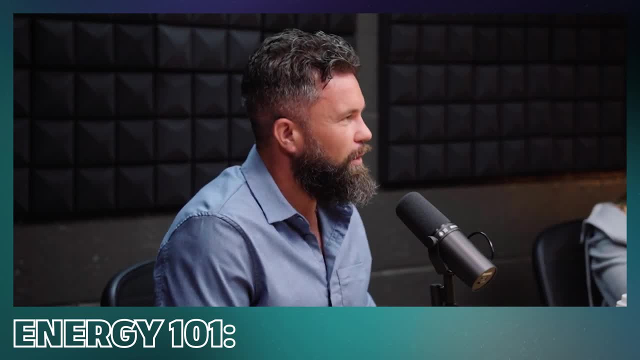 back. you know these dates And he's like, but if you ever asked me for time off from the bathroom again, you might as well not come back. And I was like, okay, noted. Yeah, I'll come in through the. 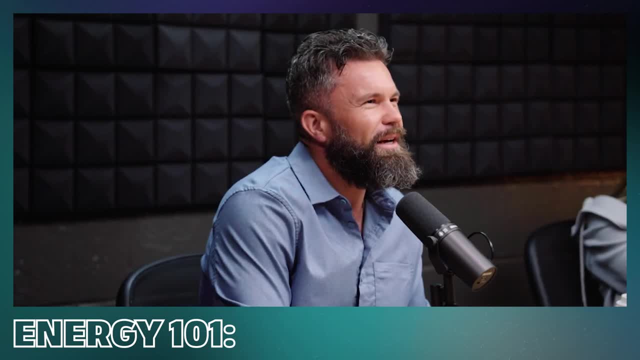 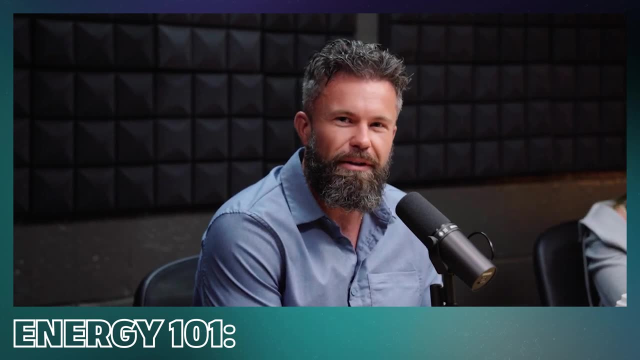 front door instead of through the bathroom door. Yeah, Yeah, So that was the normal thing. I'm sure he's probably this dumb kid, but yeah, Um, that's. I don't know if that's the most embarrassing, but I'm embarrassed to like describe that, So I don't really get that. 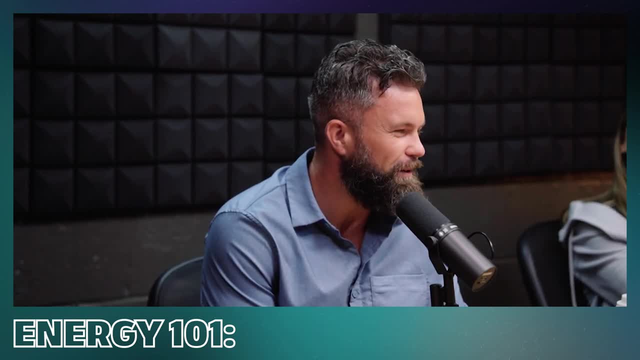 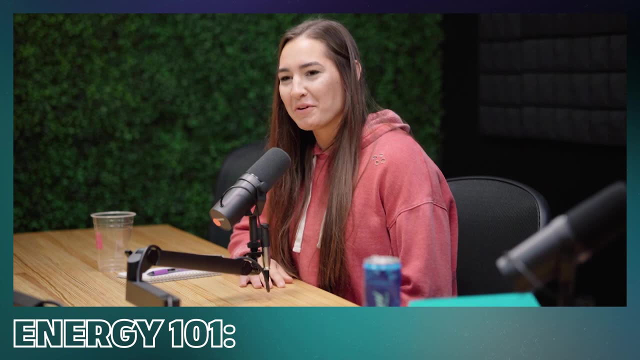 much, but yeah, that was a highlight of my career for sure. Yeah, Yeah, Well cool. Thanks for coming on. I know you have a meeting to run too, No worries, This has been fun. You ladies are crushing it and I'm super pumped to see how this evolves. and, like I said, evolve or die right. 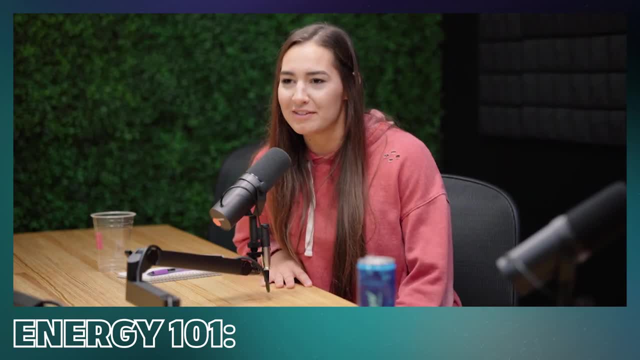 Yeah, exactly Yeah. We'll have you on when we know a little bit more and you can talk to us more in depth. Yeah, no worries, I hope I did an okay job. It's again, it's, I'm working on. 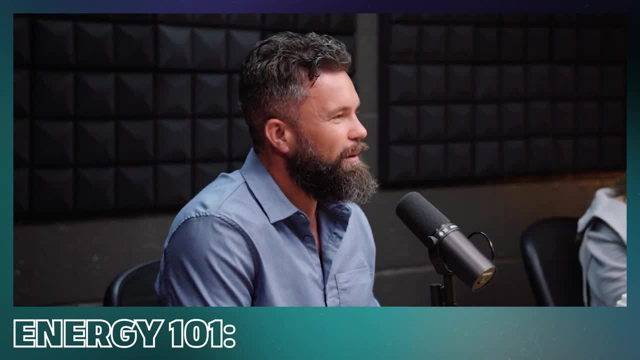 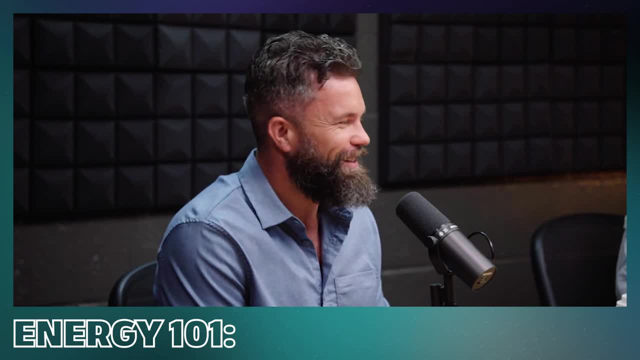 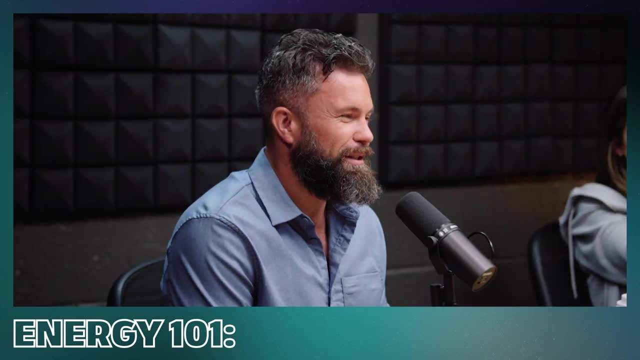 idea: Awesome. Well, thank you Justin. Yeah, you're welcome. Thank you guys. Should we plug your podcast? Oh, sure, Our non-existent followers, You guys are going to have lots. I'll make sure my mom subscribes, Thank you, Yeah, We got one subscriber Our moms are Yeah, Yeah, No, my mom's. 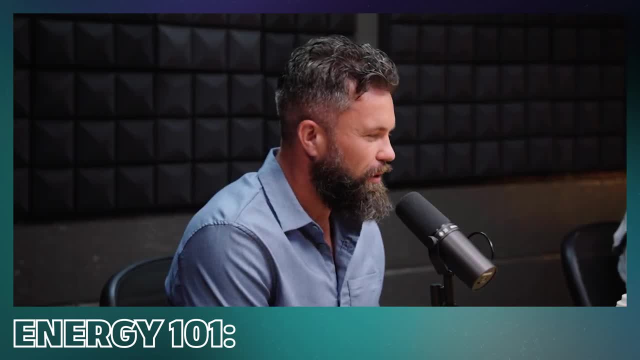 always like I listened to your podcast again, I was like, yeah, So yeah, if you want to, so again I have a podcast: wicked energy with JG. You can find it on all directories, Um, and it focuses. 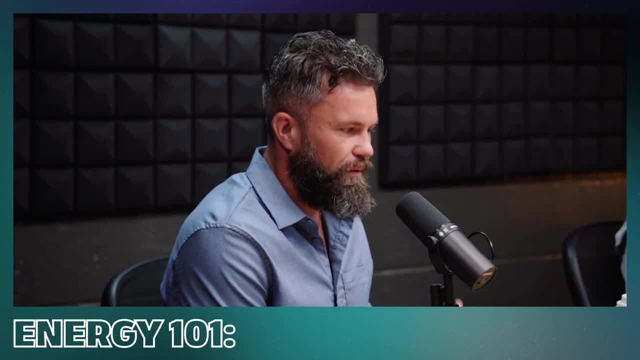 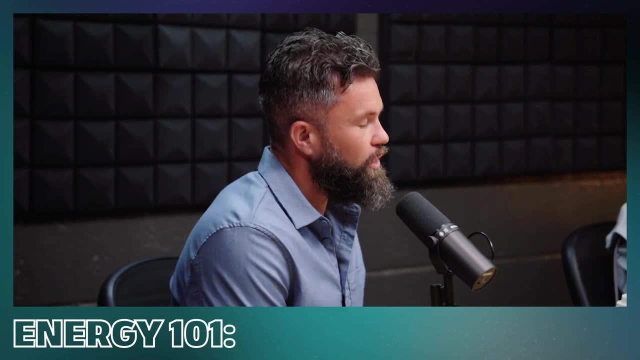 around having discussions about, um, you know, a lot of the challenges, the innovation, the transition, uh, and and through through uh speaking and interviewing energy thought leaders, And so, um, yeah, just continue to educate, dive deep into a lot of the challenges and and just some really. 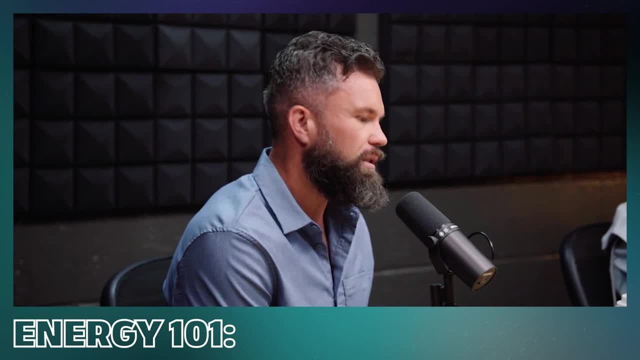 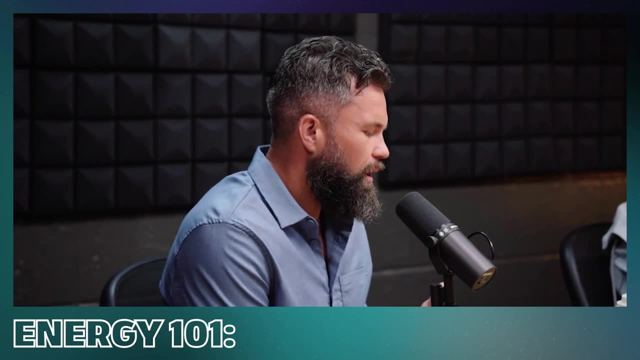 good discussion on oil and gas, whether it's technology policy, um, you know, the transition sort of all things Good for energy. So, and then two is like how? a lot of the conversation I'd like to have is: how can we help provide energy to the world? Cause I think one of the problems is, you know, it's one thing. 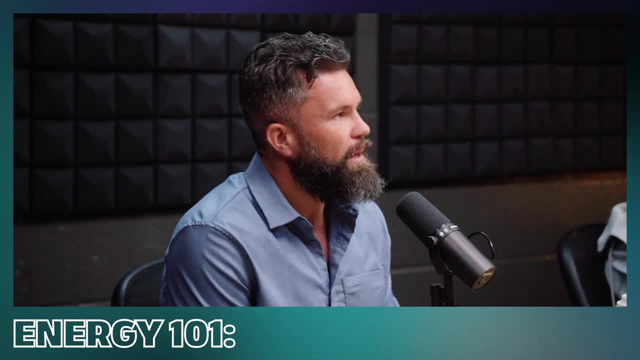 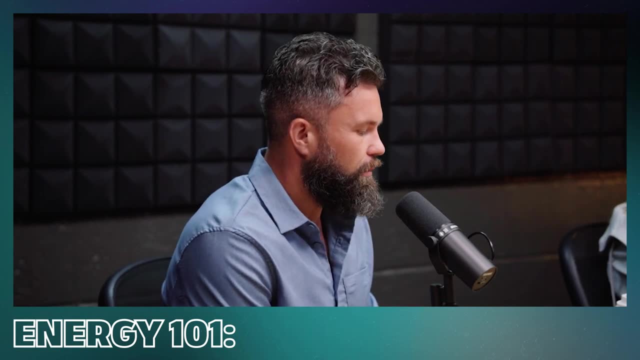 to help, you know, reduce emissions and everything else, But I think the biggest problem we have right now is energy. poverty in lots of parts of the world is so how can we, how can we allow for people to have access to reliable, abundant and affordable energy? I think that needs to be the 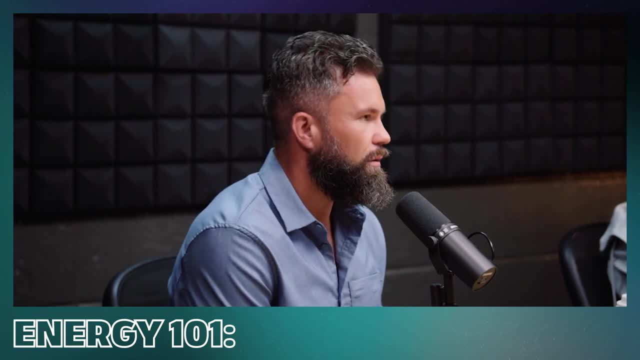 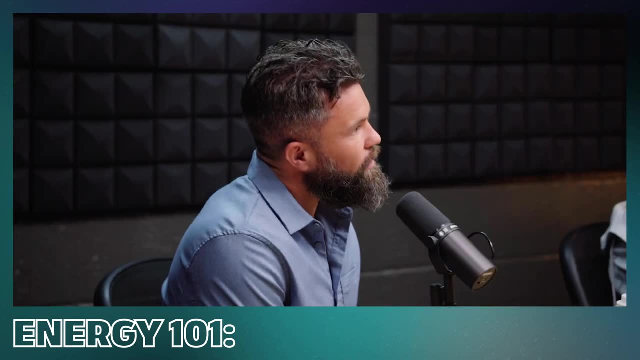 North star And then beyond that, we can continue focusing on, you know, reducing uh emissions and and all you know, the greenhouse gas effects and everything else. but that's a privilege, Yeah, it is Right. And so there's countries out there who don't care.